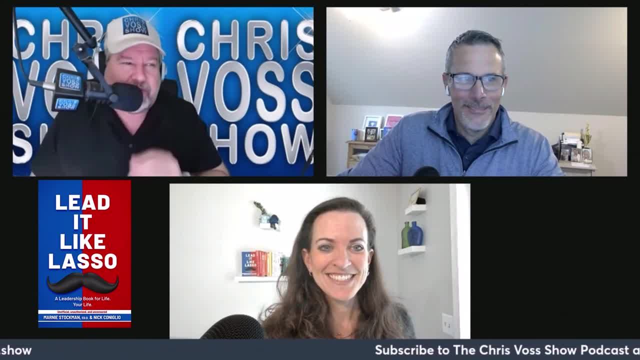 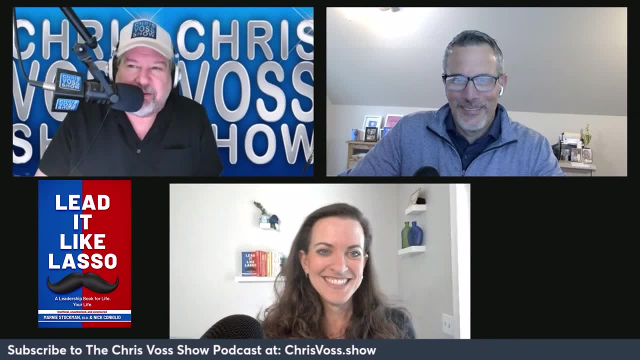 gentlemen, Welcome to the big show. We certainly appreciate you guys coming by. As always, the Chris Voss Show is the family that loves you but doesn't judge you, at least not as harshly as most of your other family members, because you're the one they always make sit at the Thanksgiving. 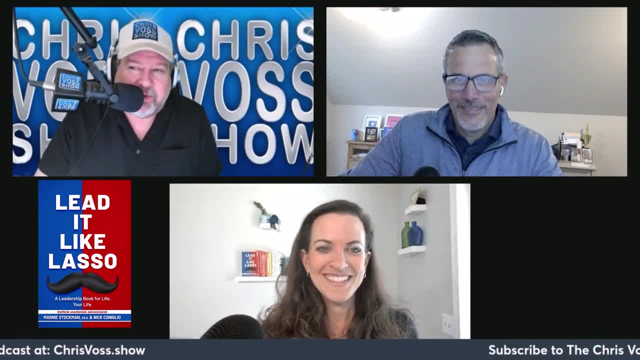 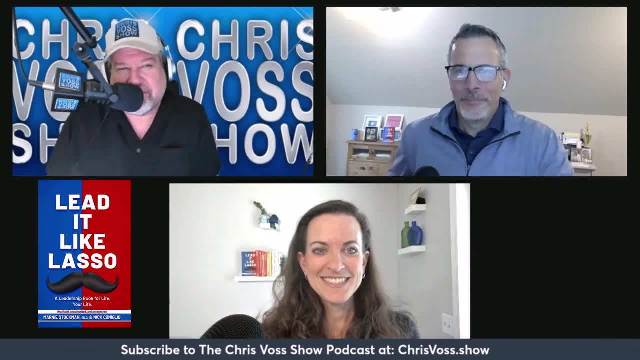 children's table, And you know it's personal. I would take it personal, But you know what? If you want to get on the good side of your family or friend in the Chris Voss Show, go to goodreadscom 4chesschrisvoss. linkedincom 4chesschrisvoss. youtubecom 4chesschrisvoss. 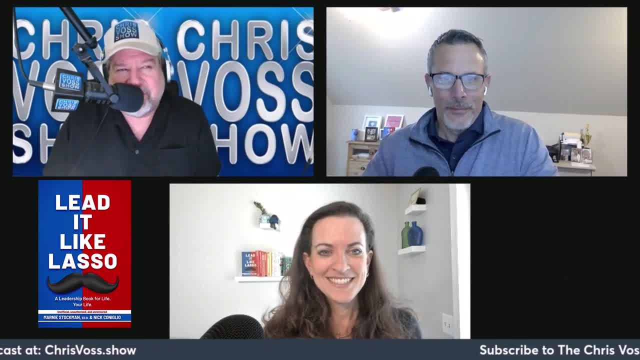 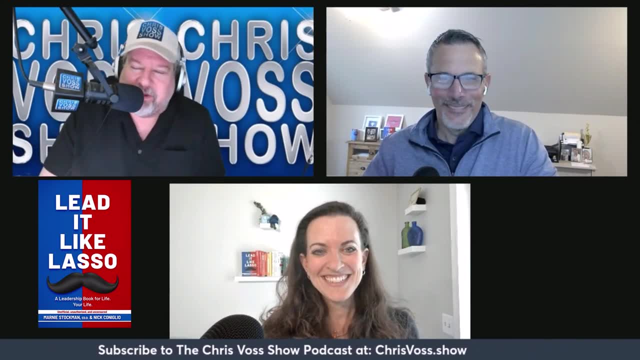 and I don't know all the crazy places on the internet, And we guarantee on the Chris Voss Show that they will invite you to the adult table this holiday season or not, I don't know. I don't think we can make those decrees. I have an attorney yelling in my ear. Anyway, guys, we have. 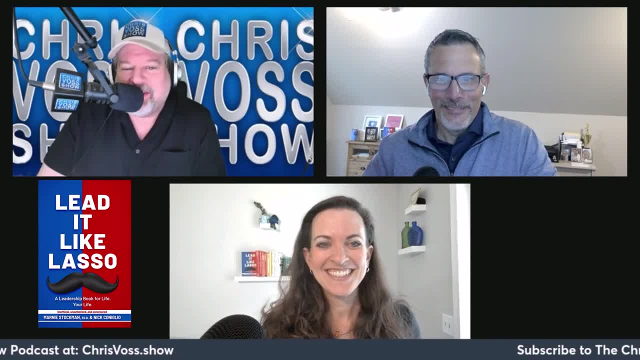 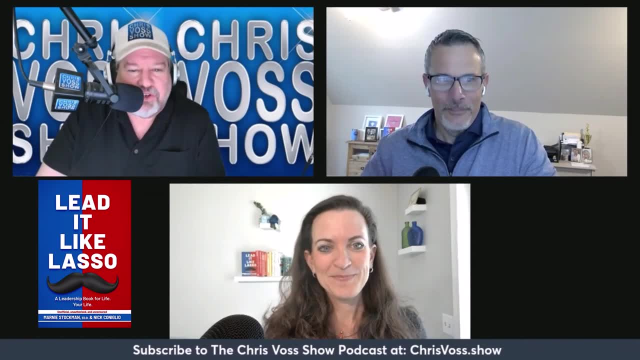 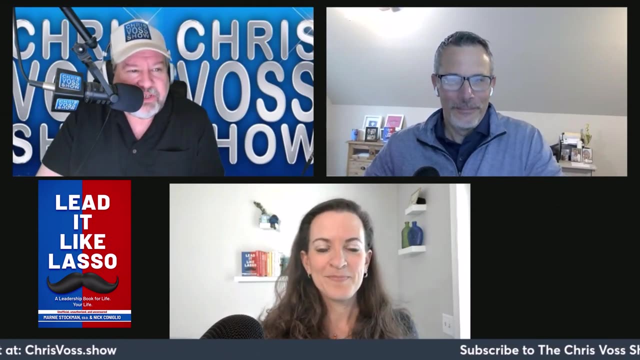 amazing authors on the show. Their latest hot new book came out October 27, 2023.. It's called Nick Lasso Leadership Book for Life- Your Life as well. We have Marnie Stockman on the show with us today and Nick Coniglio on the show with us today. Did I get that last name right, Nick? 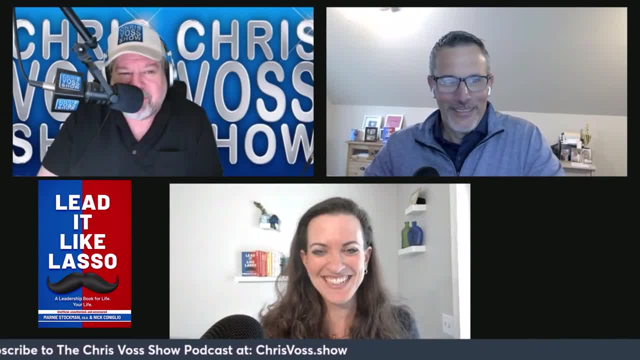 You nailed it, Chris Nailed it. That's a score one for me for all the times I failed. There you go, So we're going to have both of them on the book. We'll be talking to them about them on the show. Marnie started her. 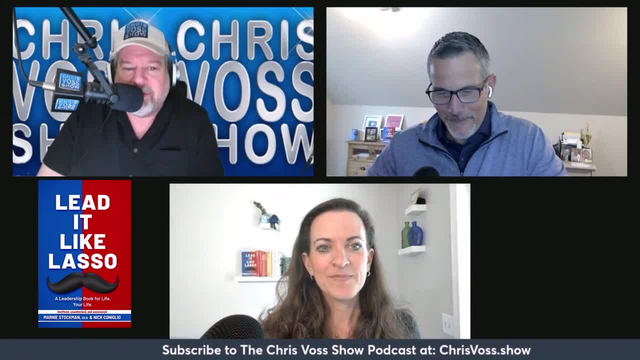 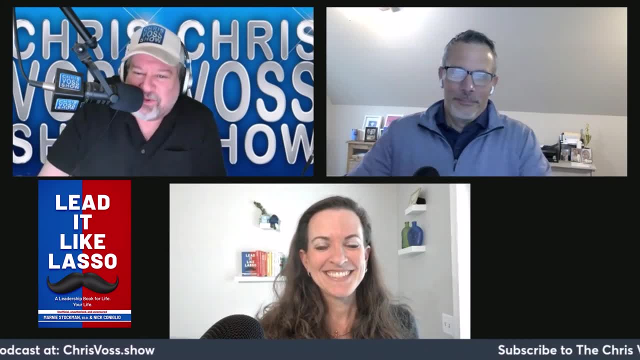 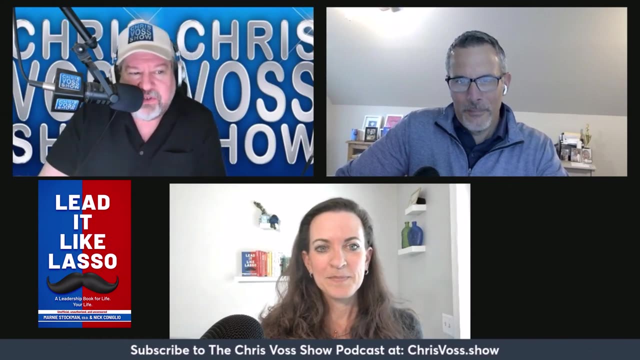 career in leadership with the toughest customers and employees of all high school math students. Wow. Her Passion for education and using data and humor to help others grow and succeed took her from the classroom to senior director of customer success of a leading education tech company, and now to 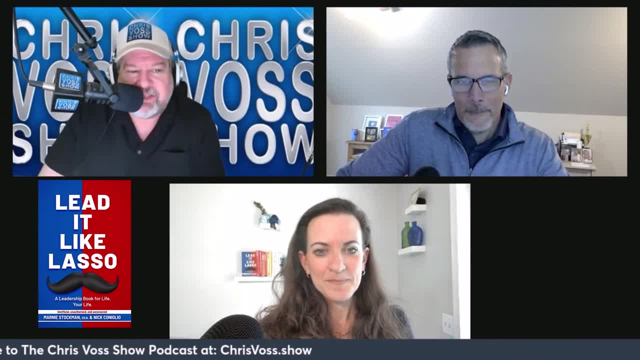 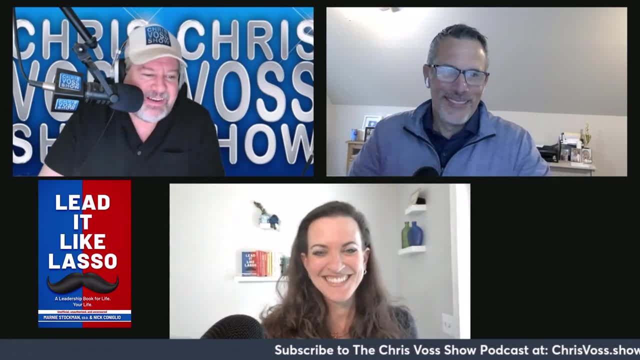 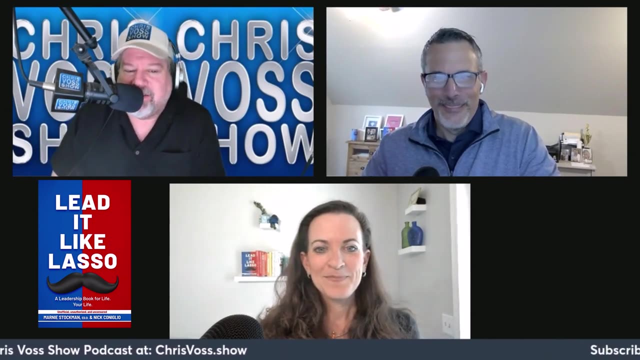 co-founder and former CEO of Lifecycle Insights, a VCIO customer success platform for MSP, She'll have to explain what all that means. Nick is a seasoned technology veteran with over three days of experience in the ever-evolving world of IT. I know what that is. No, I don't Born with. 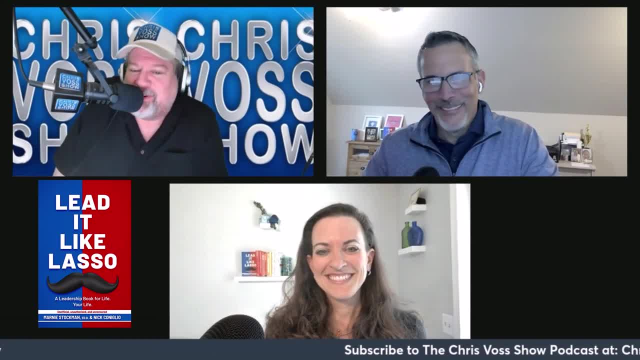 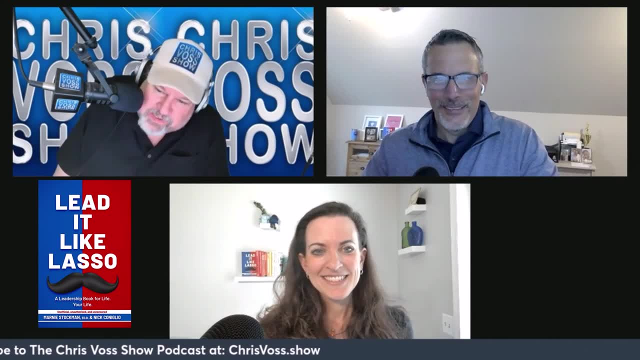 an insatiable passion for problem solving and give for unraveling the mysteries behind technology's hiccups, including the mic problem. I had earlier Nick embarked in his tech odyssey in the early 1990s as a mainframe programmer and he's done numerous hats. Welcome to the show. 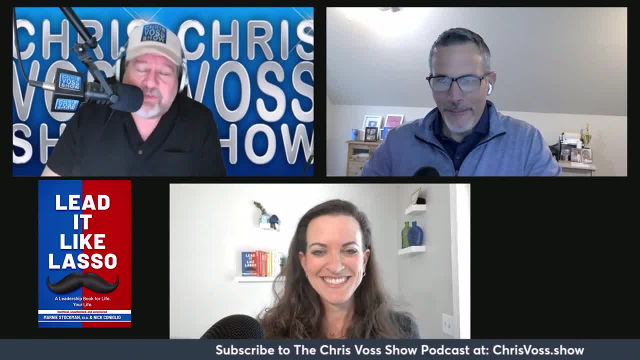 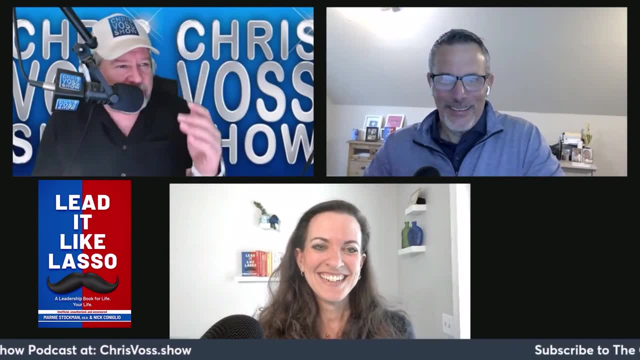 Nick and Marnie, How are you? Great Thanks for having us. Thanks for coming. We really appreciate it. All right, Thanks, Great show folks. See you tomorrow. No, I'm just kidding. Give us dot coms. Where do people want to find you on the interwebs? 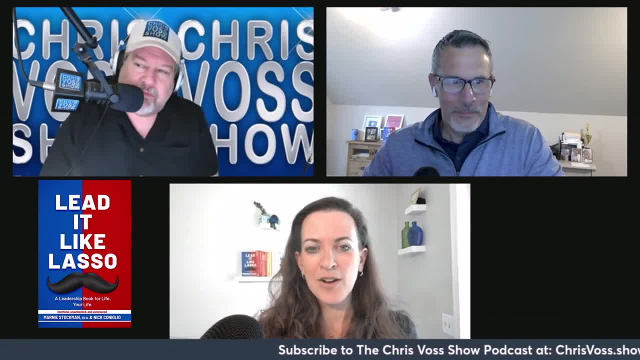 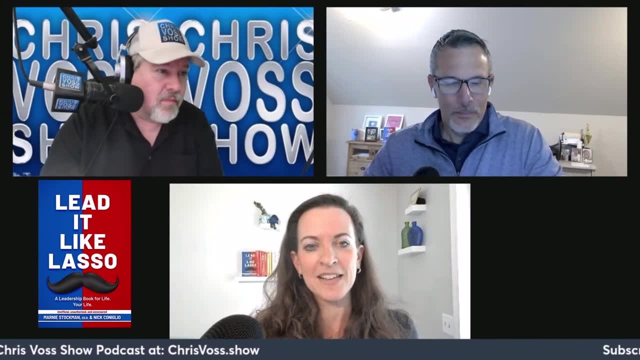 Yeah, Leaditlikelassocom. And we own all of the socials: Insta, Twitter, LinkedIn, Facebook, TikTok on Leaditlikelasso. So easy, We keep it simple. There you go. There should be a song for this, I think. 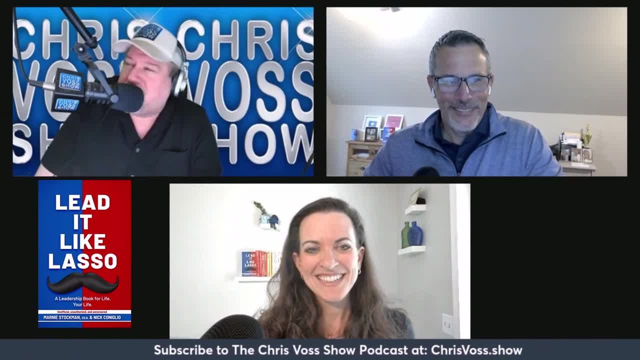 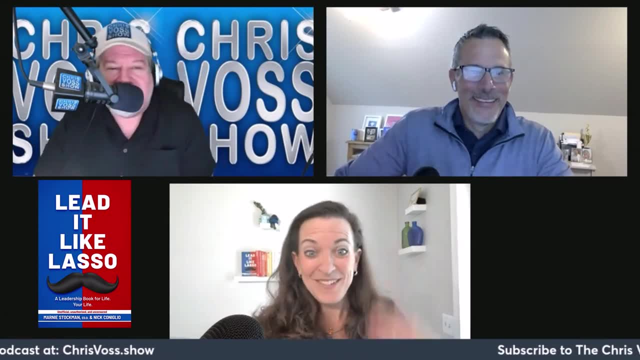 Isn't there like a? what was the song? Do it like a Jagger, Move like Jagger. Yeah, There should be a lead it like lasso. Take that They actually referenced that song in the show, So that's funny. 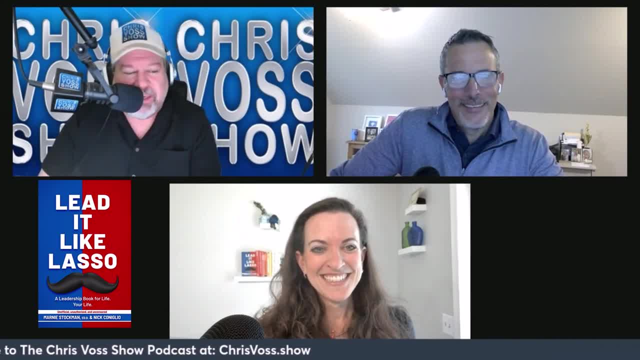 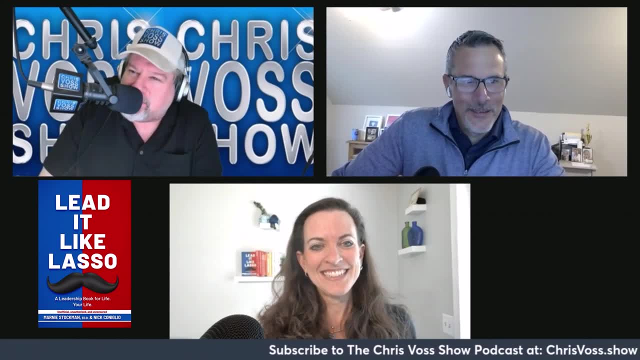 Yeah, Yeah, You know there's. there's a. I just came across this AI thing and I'll have to pull up what it is, but you can literally use it. It's Sono or something here. Let me pull it up. 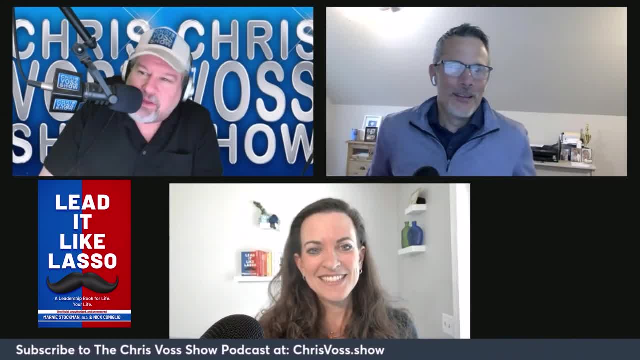 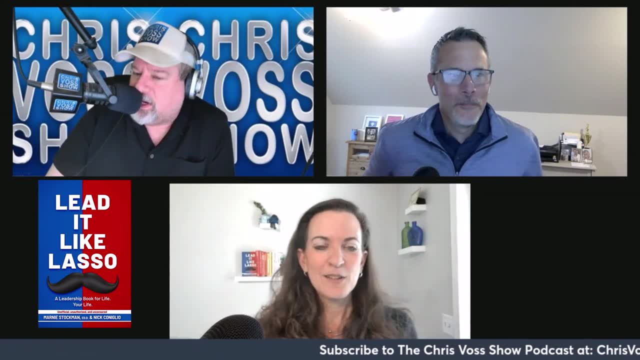 but you might be able to use this, but our audience will like it too, as well. There's something that I just found the other day That's really a hot new thing on Twitter and stuff And and it's called Suno at app Suno, Suno S-U-N-O dot AI And you can literally tell. 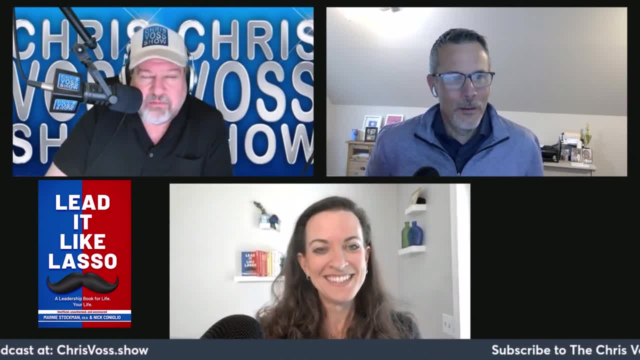 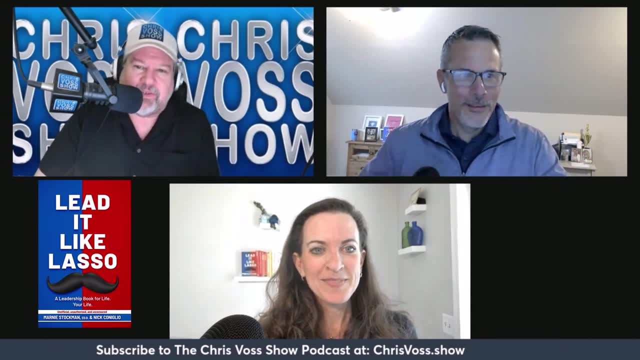 it to make songs and And Ling goes for you or Ling, whatever. you know what I mean. And so we went in and we told it to make a song for the Chris Voss show podcast and how cool it is And it like made up all these. 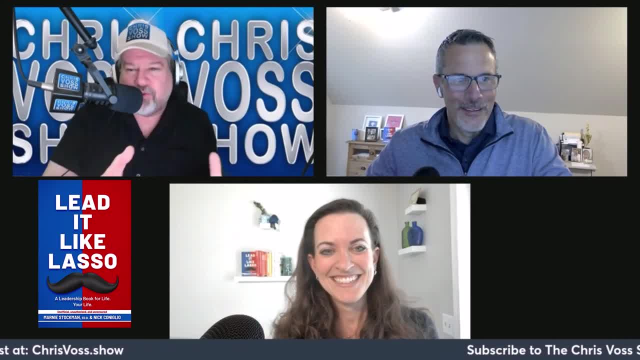 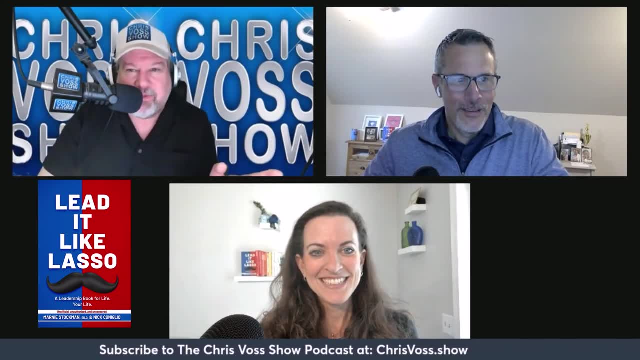 lyrics and and it wrote the song And then you can choose what sort of genre you want to have, like metal or blues or, I suppose, rap or you know whatever sort of musical thing is. So we had to make a bunch of Metallica styled the Chris Voss show podcast. 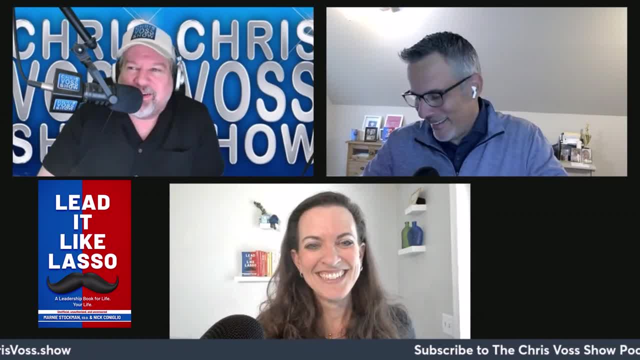 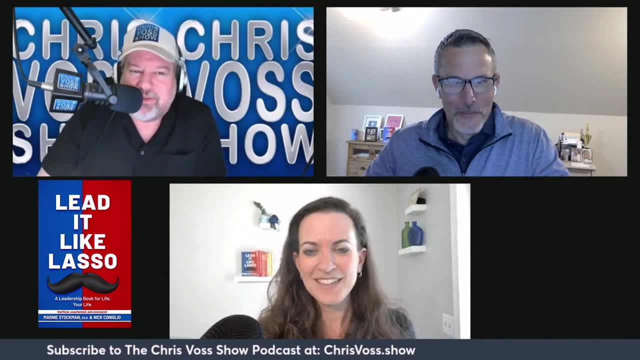 Enter Sandman Chris Voss. Yeah Yeah, It was like really heavy stuff. So if you guys want to do that with your lead at like Lasso, I think a song should accompany this book. I think that needs to happen. 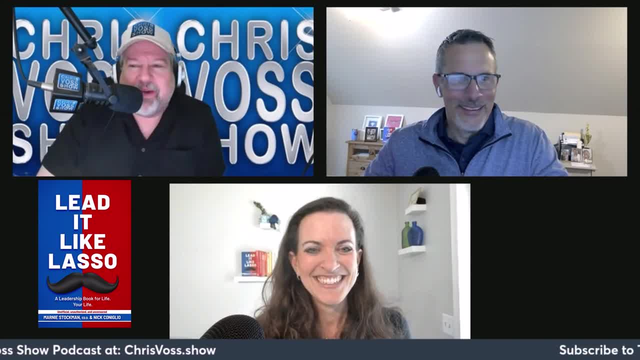 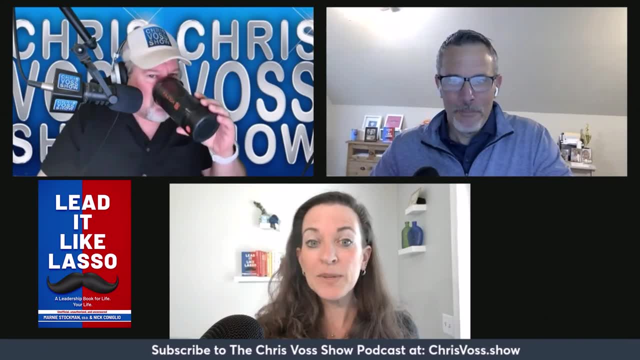 I think it's perfect. I love it. So, getting back to the book, give us a 30,000 overview of what's inside the book And I'll give both of you guys a stab at it. Yeah, it is. We said it's a leadership book for life, your life. So, as opposed to strictly being 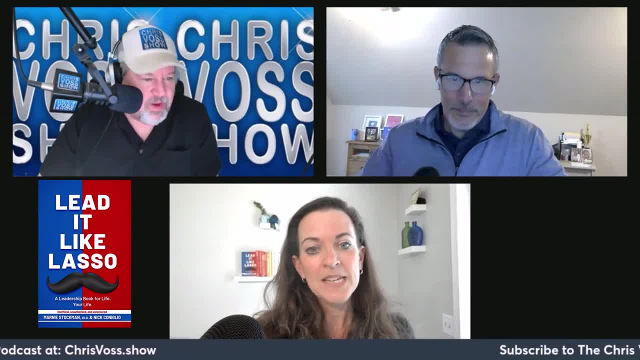 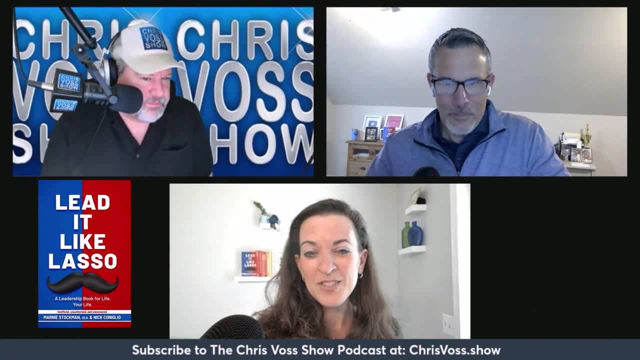 a business leadership book. we focus on personal leadership. So Ted Lasso the character was all about. it's not about the wins and losses, but helping people. It's about helping everybody become the best version of themselves, And so we really focused. 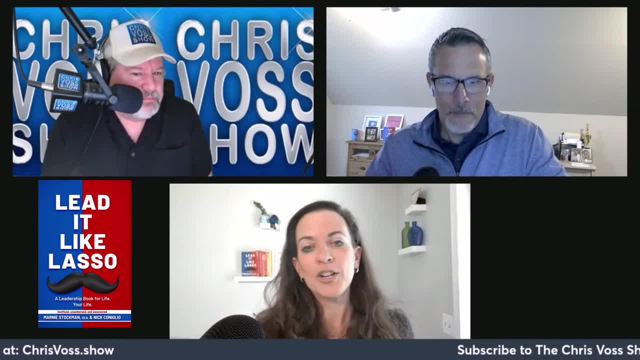 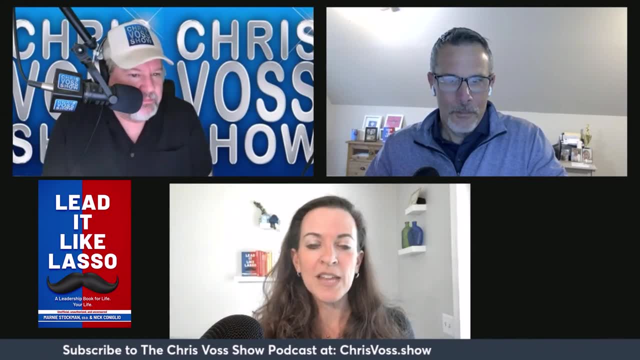 on how to take a look at yourself and work on yourself as opposed to you know they always say in business, work on your business instead of in your business. And so we kind of took that approach with a leadership framework And I'll let Nick talk about, like the relatability of Ted. 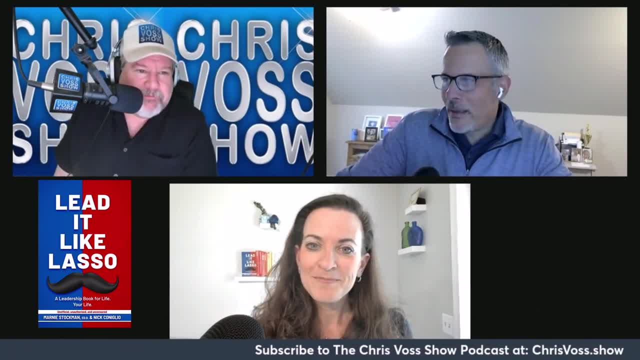 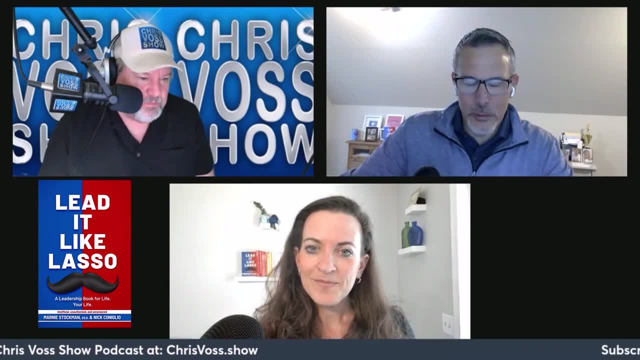 Lasso and more on that. Yeah, Yeah, I mean I think that was what we tried. I mean we watched the show Ted Lasso And if, if you scour socials and we didn't know this at the time, but there are millions of just. 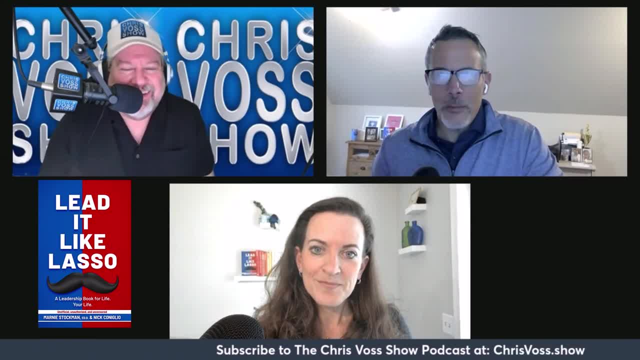 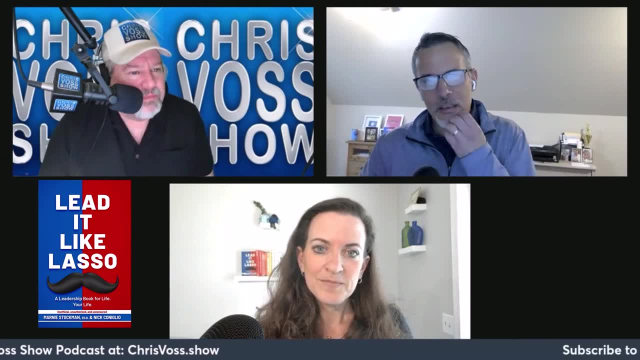 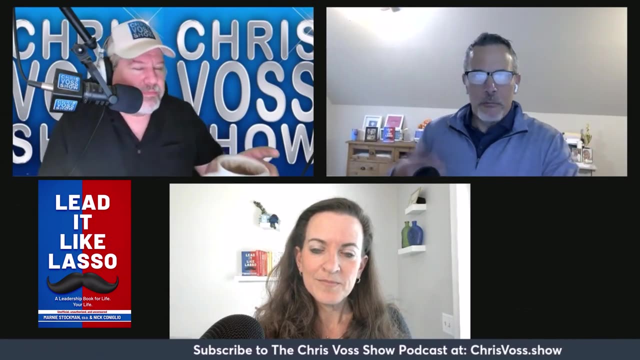 diehard Ted Lasso fans And I think what they talk about most is how they feel after watching the show. And I and I I think a lot of that is the character development right And how they grew over time And we kind of married the leadership framework that we had built over. 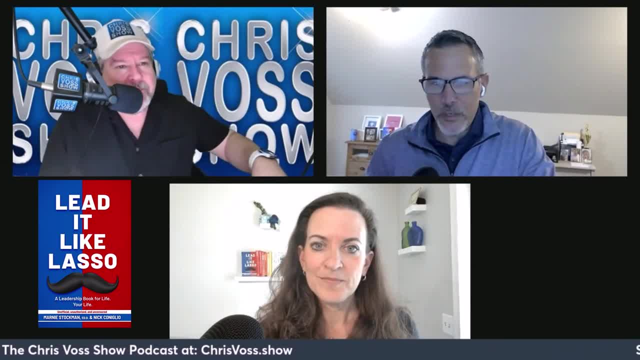 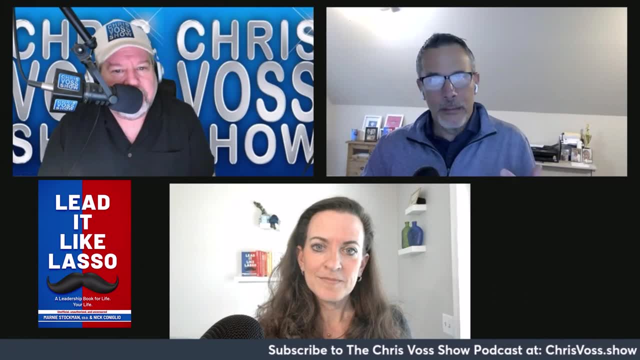 the years Marty and I have worked together- for you know, more than 10 years now- And we, we built a, an operating framework that was based on a leadership style, And when we wrote the book, we're like: Hey, you know, relatively, I mean, we're relative nobodies, right, I mean people. 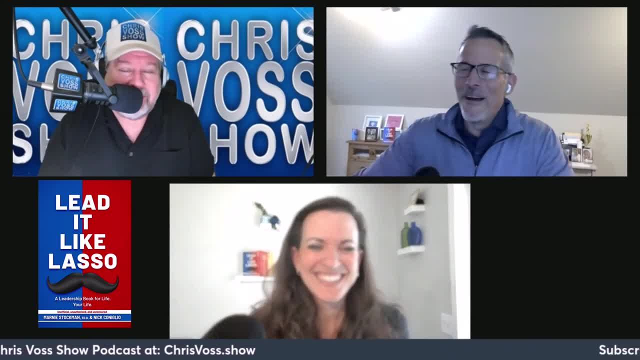 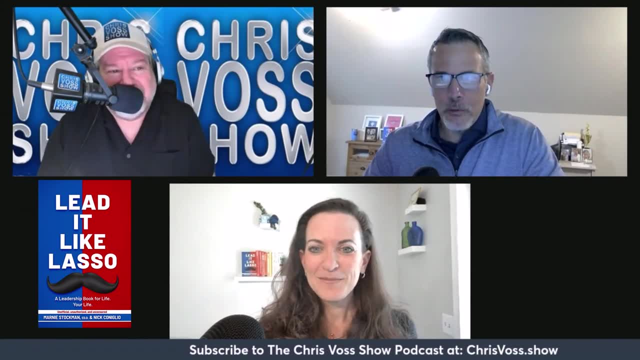 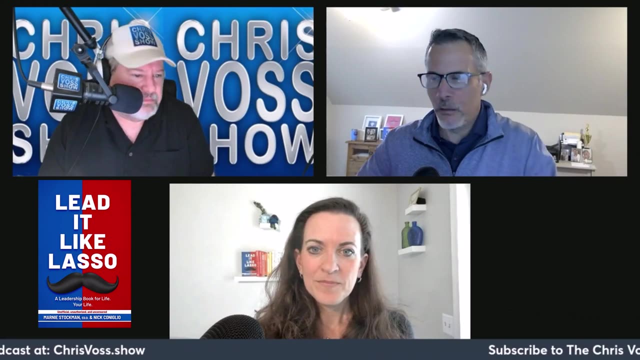 have never. we're not Chris Voss. People have never heard of him. That's not true. Yeah, But, but we wanted to to leave the reader, you know, in a different way when they then when they typically read a leadership book, right, Which is very theoretical and 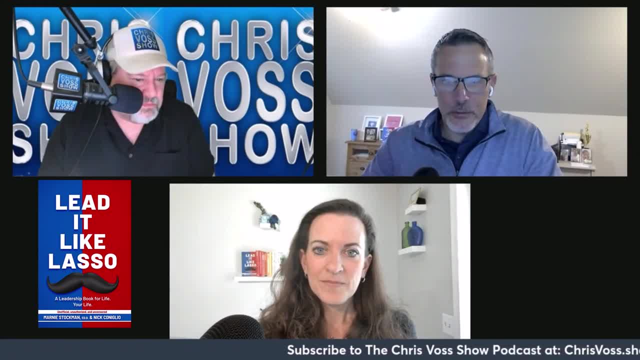 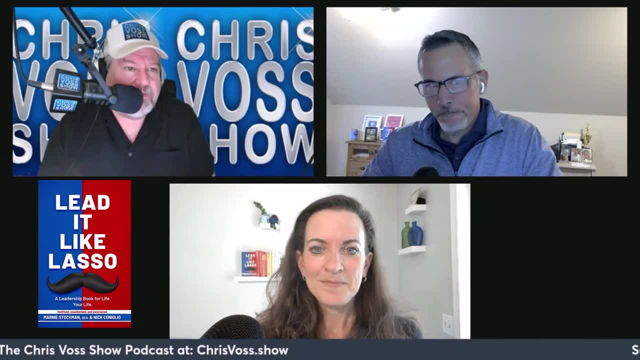 and classroom oriented. We wanted to make them feel good, Relate to it, And we use the show Ted Lasso as a reference and people have really, they've really grasped onto that. There you go, And then let's just flesh out for anybody. 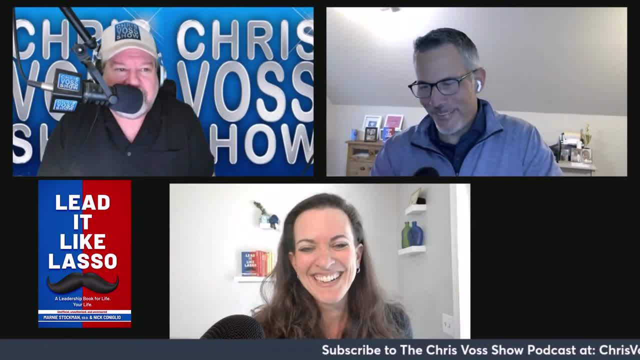 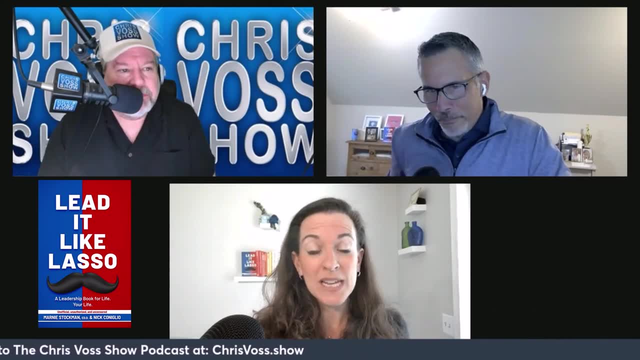 who hasn't seen the show because they lived under a rock or something. Who this Ted Lasso show and person is about? Yeah, So he was an American football coach who went to England to coach European football, which we all know is soccer, And what we find out at the very beginning. 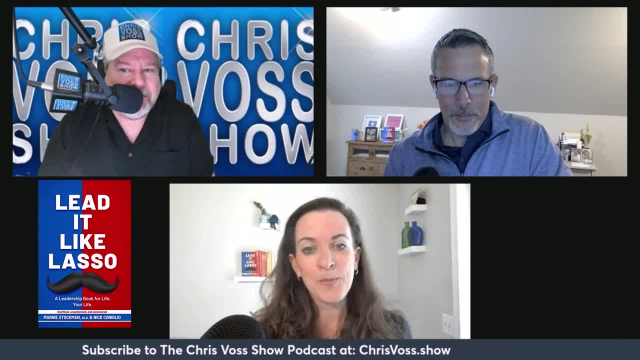 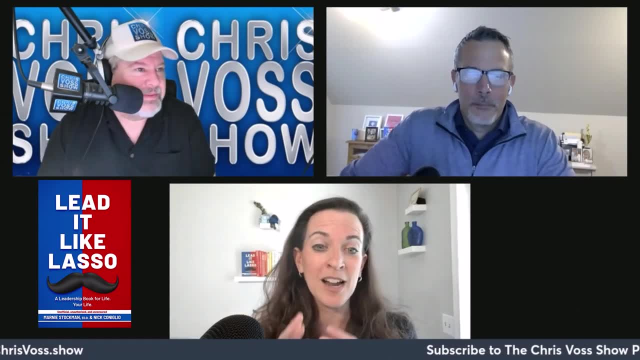 but he does not know is that Rebecca Welton, the co. the owner, is trying to get back at her husband, who is now her ex-husband, And so she hired him to sabotage the team and have it crash and burn, And so that this first season is. 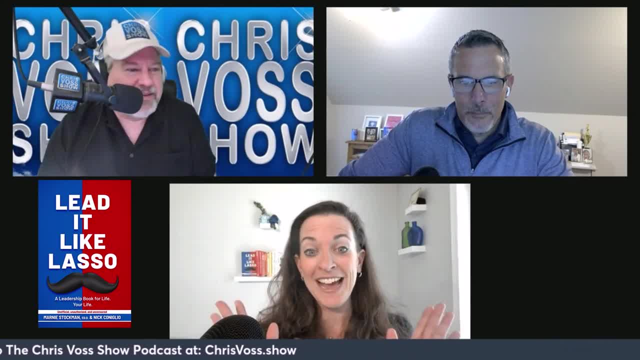 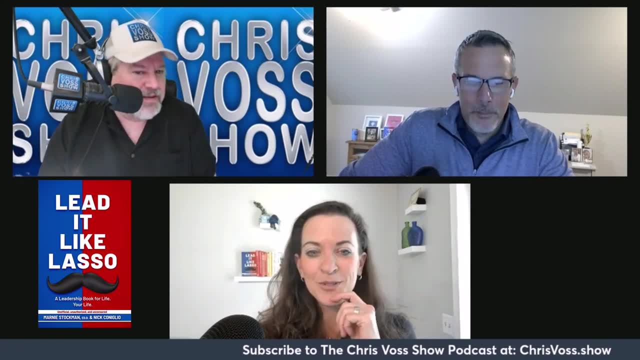 especially is watching the conflict of that, because even though there's two full internets of what Ted doesn't know about soccer, he does know a thing or two about coaching. Oh yeah, And it's it's. I think the other thing to add is his infectious optimism, and 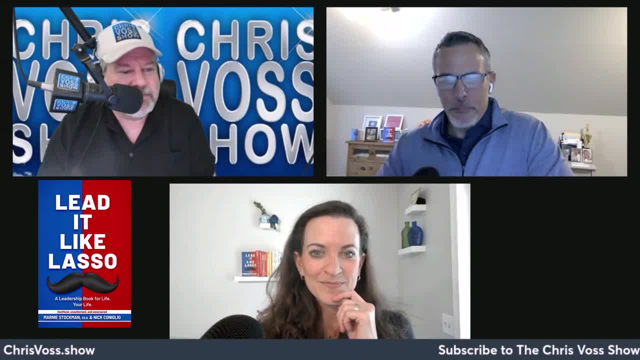 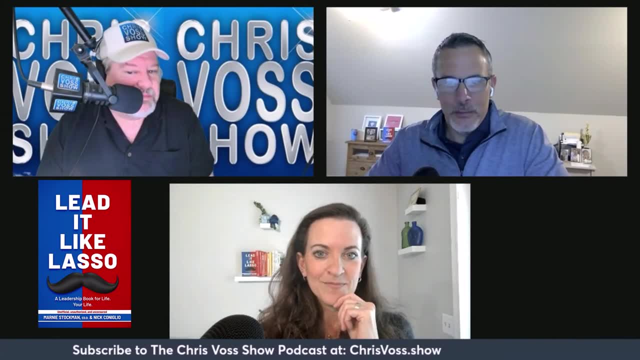 focus on team dynamics right If it basically fosters a transformative change, you know, with the players and the teams and it it kind of makes everybody feel good. It's not. it's not a show about soccer, which I think has stopped a lot of people watching the show. It's. 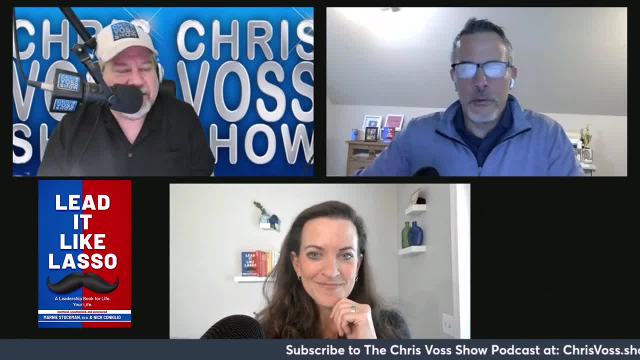 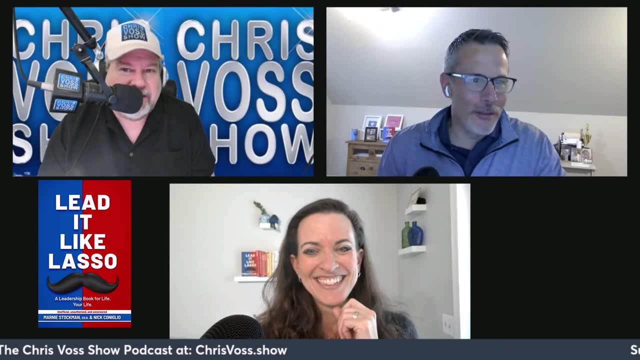 really a show about relationships, you know, personal growth and the power of positivity. I need to watch it now. You guys have sold me on it. Excellent. We also work for Apple TV on this. Oh, we don't, We do not. 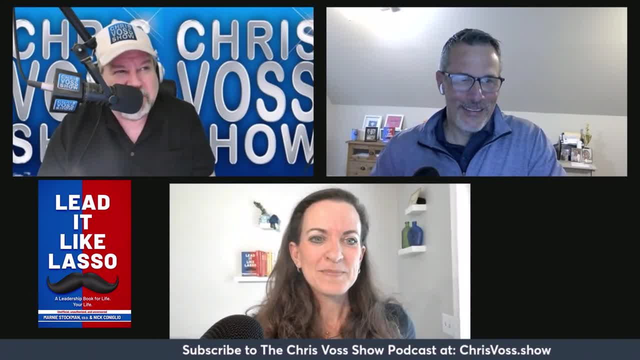 I'll watch it. I think we have an actress, a movie star for the for a movie on Friday, that I've got to watch a movie tonight. but I'll get to this lasso thing: The it's the, what's the movie? 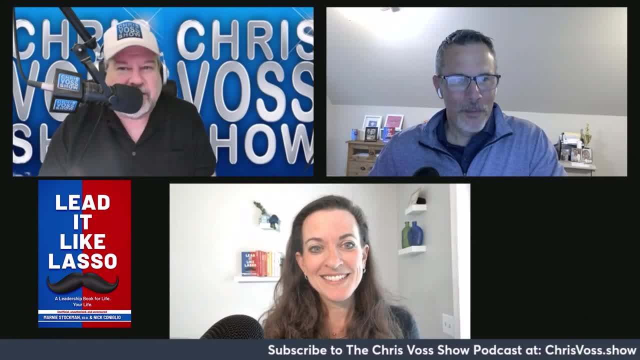 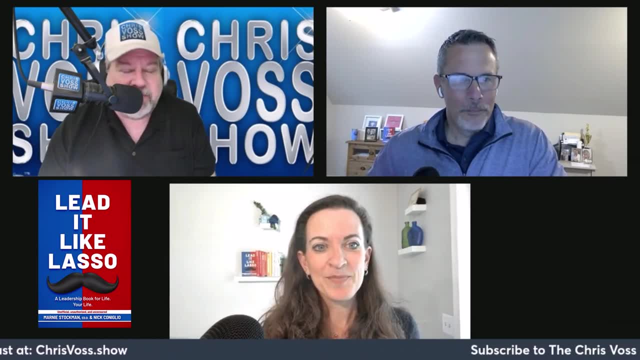 that she's in anyway, but she's going to be on Friday And so I got to go spend, I think, an hour or two watching the latest movie- and it's going with Al Pacino and who's the guy from anyway. So I got to watch the movie, So I know what the hell's going on. but after that I'll watch the. 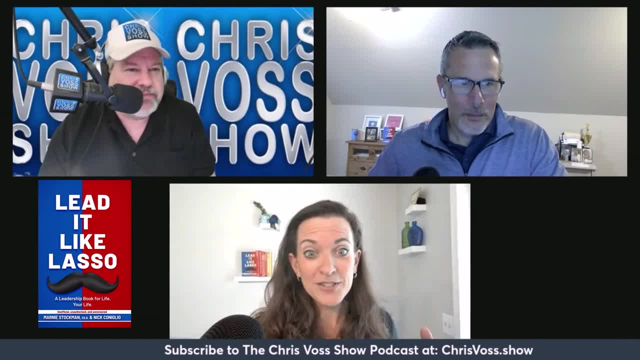 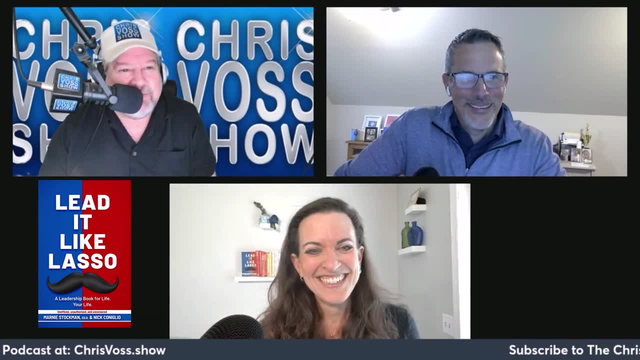 lasso stuff. So when you watch lasso and invite those actors to come on the podcast, let us be in the green room And we'd love to meet them There you go. I'd love to get, I'd love to get some of the actors from that on, Is it? 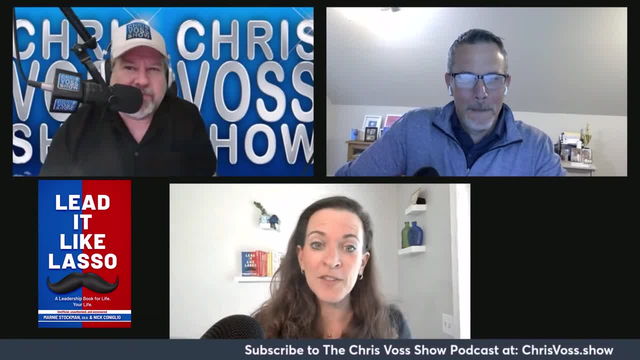 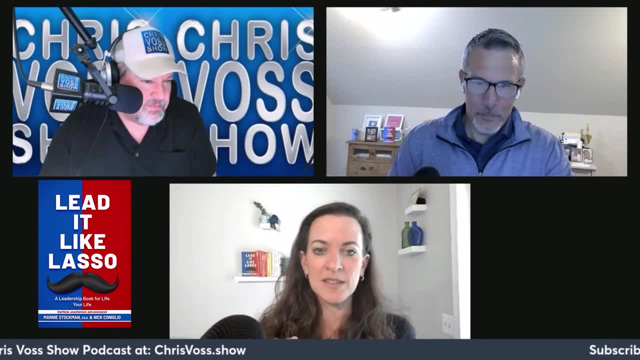 still running? It is not. So. that is part of the parallel of the book and our lives, is it? we grew our business from $0- actually from $16,000 bootstrapping- to an eight figure exit in the same three years that Ted lasso aired. 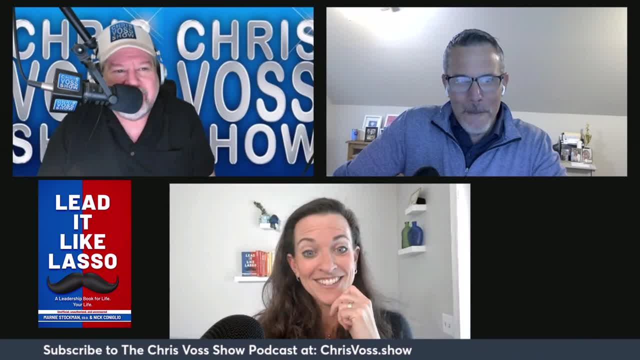 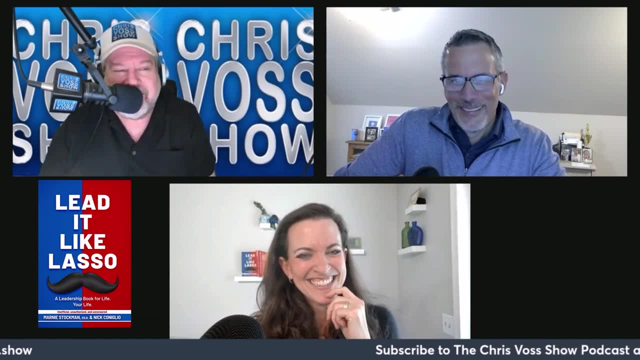 That is awesome. You know how hard that is to do. Yes, We do. I was talking to the audience. I guess, really To frame that to like Hey audience, do you know how hard that is to do? We started first two. 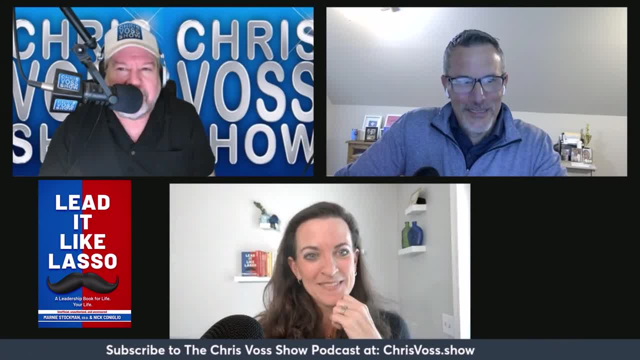 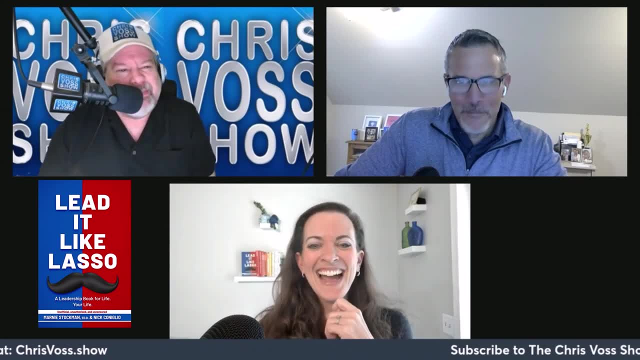 companies with 2000 and 4,000 built them into multi-level marketing or multi-level multimillion dollar companies. I went to the gym this morning so I'm hemorrhaging a little bit on the brain: bleed Leg day or upper body. 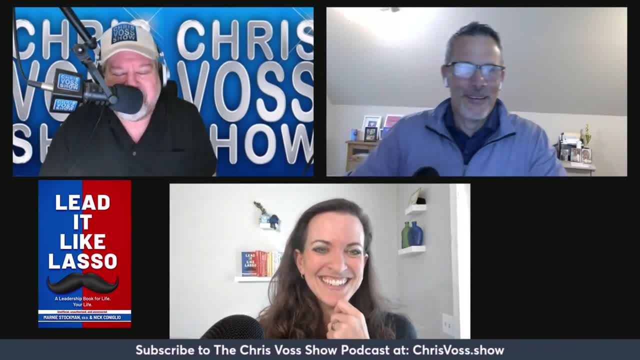 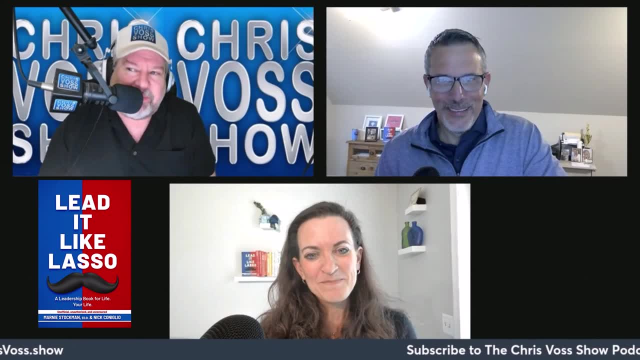 No, it was upper body arm day I tore myself up. So after this podcast I'll probably be napping and sitting in the fetal position going: everything hurts. So there you go. That's why the brain isn't working. So tell us a little bit. 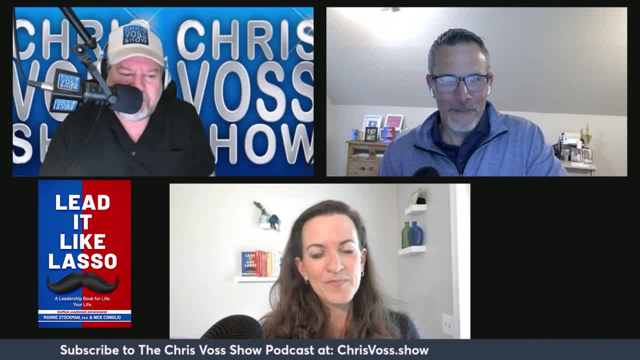 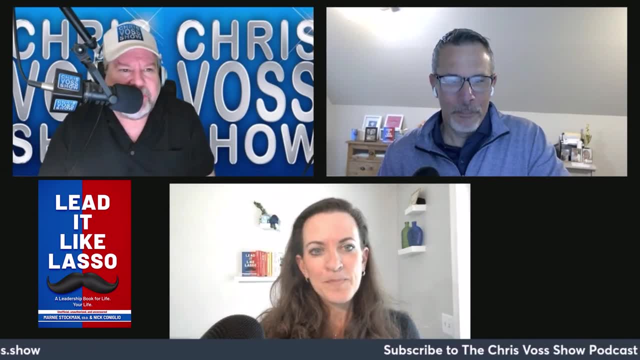 People like to know about the authors as well. Give us both, take whichever turn you want. Give us both your kind of histories, kind of your upbringing, your journeys a little bit. What got you to this point where you're writing the book? 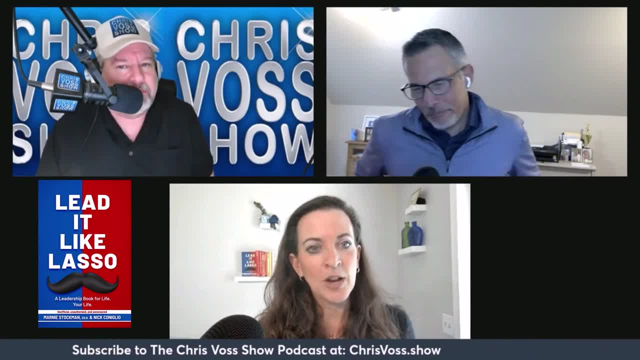 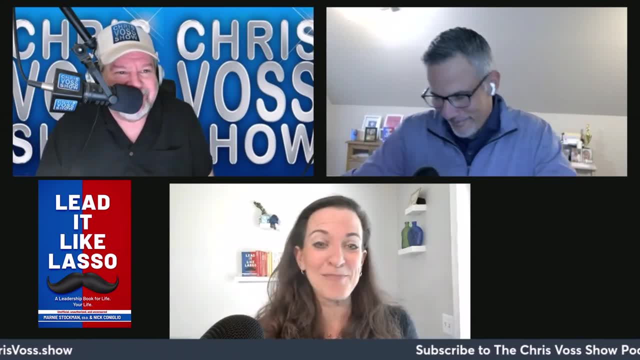 As I, as you said in the intro, I started out as a high school math teacher, which I always say means I sold pre-calculus to 16 year olds, so I can sell right, Like you had lots of stories in your book about how you sold. 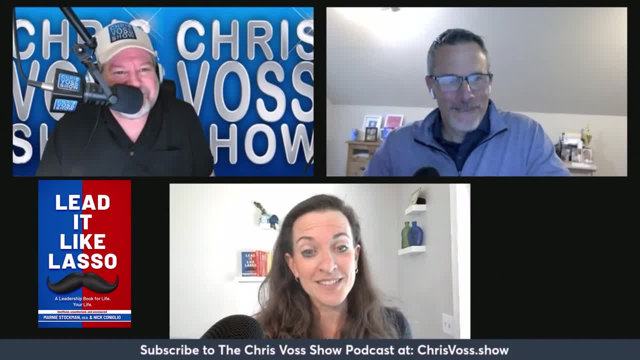 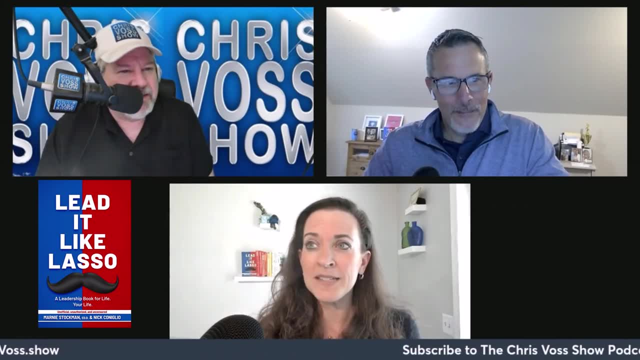 early on and I did the same. but when you're pitching pre-calculus it's a tough gigs. I left from there And you know it's a tough gig. I left from there and then did administration in the school district And we worked with a particular tech software. 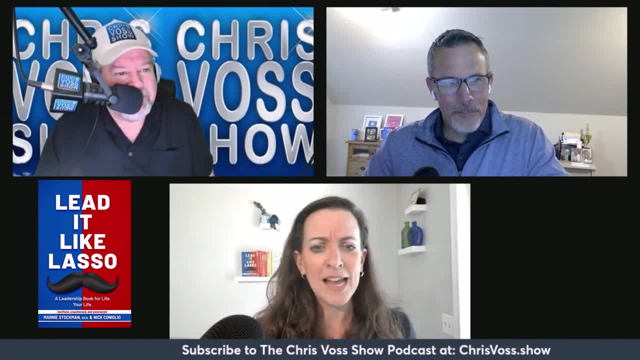 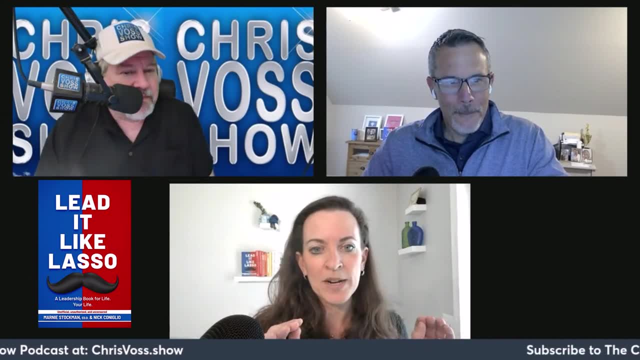 platform And one day I was sitting in a meeting and something. the trainer had an issue with the platform and she, she pinged somebody. It was the first time I ever saw a direct message on a screen And the person popped back and said: give me a sec, I'll. 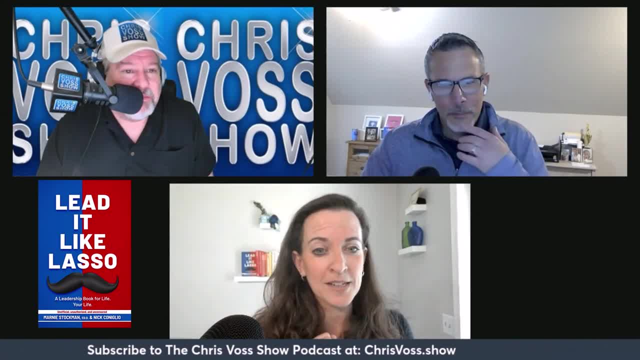 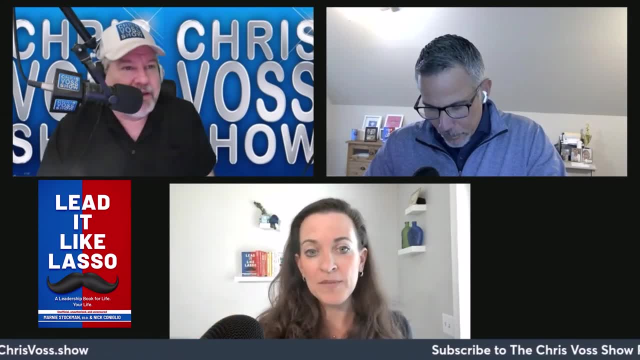 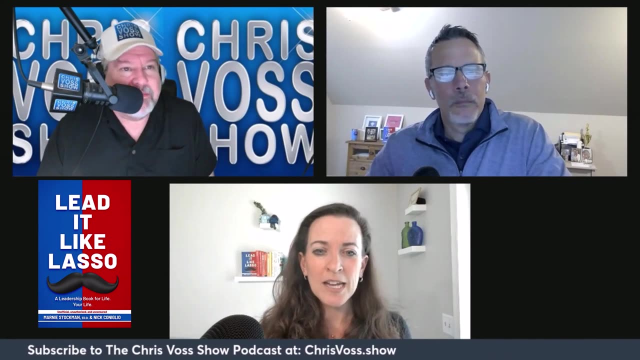 solve it. And a sec later it was solved And that person was Nick Coniglio. So I ended up working for that company Where he ran customer support. I ran- he does a lot more than that too- And I ran customer success. And then we got acquired and acquired and 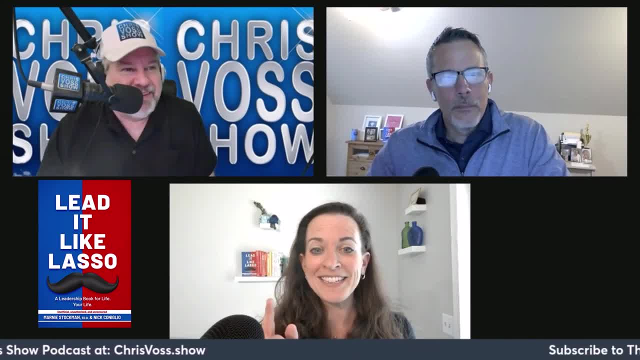 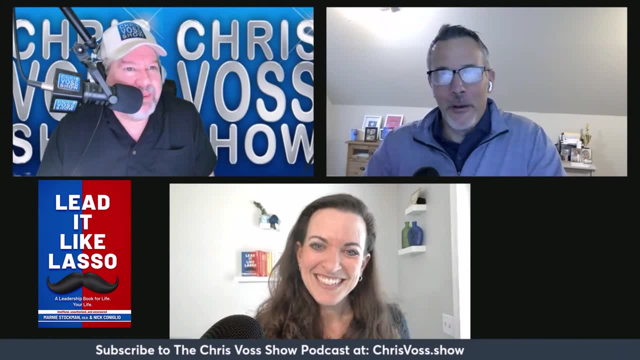 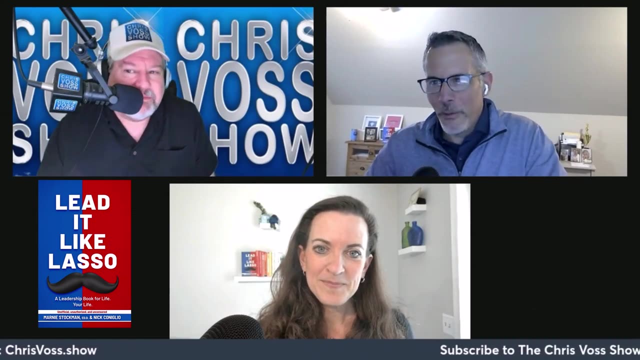 acquired. And I'll stop there and let Nick tell his background and then he can say what happened in the midst of acquisitions. Thanks, Yeah, I. you know, I was a technologist, I was a computer science major and it it suited me perfectly. My one of my first jobs out of school. I was 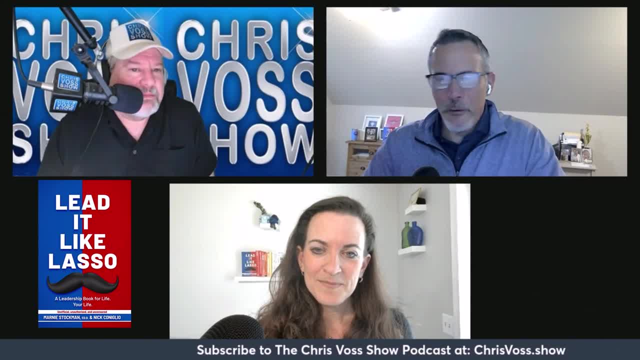 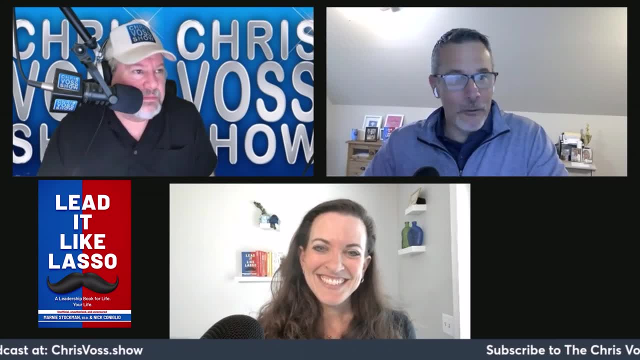 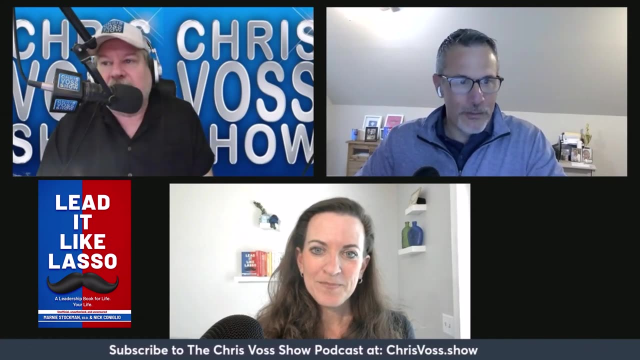 programming mainframe computers. You know I interacted with five people. you know every day drank 15 Coca-Cola's and which was perfect for me because I was shy, I was introverted. I, I think I went to, you know, went to high school. I had some classes where I said maybe three words, you know, the entire school year. 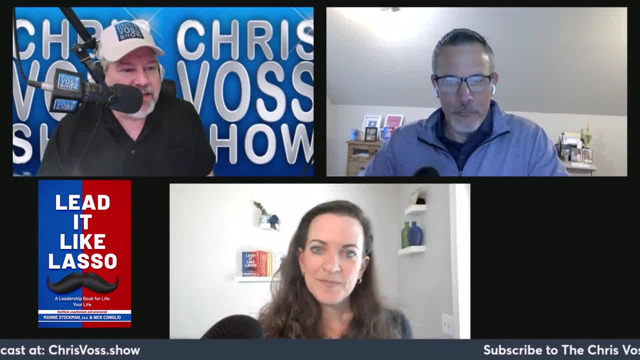 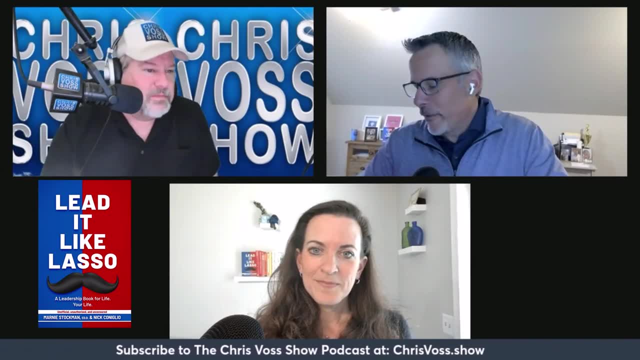 At some point I realized that in order to grow and really achieve the things I wanted to achieve, I had to make a change. I went into consulting and that's where I kind of learned the ins and outs of, you know, communicating and translating between business and 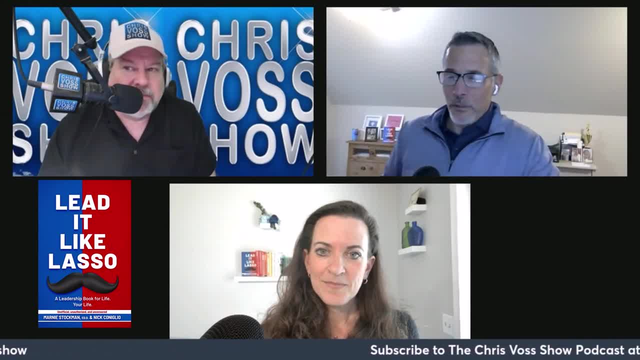 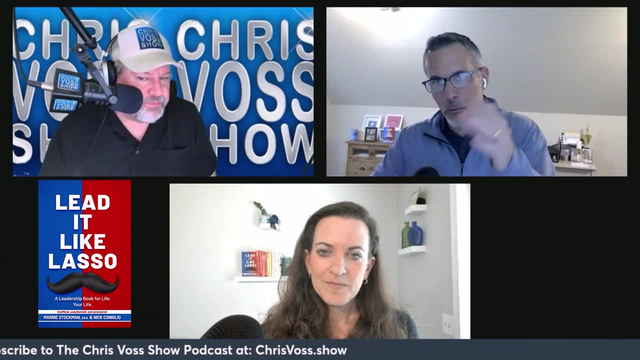 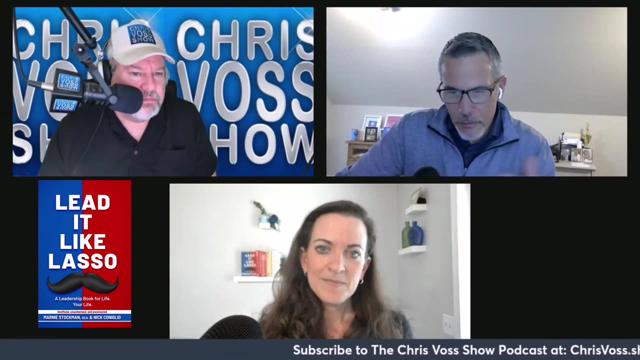 and and and technology. And I found a knack- fortunately for me, working for small companies, you know, single digit employee number- that we kind of grew, grew, grew and and and scaled and ultimately sold. Learned a lot during that time. And then the third time that happened was the ed tech company that that Marnie had had mentioned, And after we were acquired and acquired, and acquired. 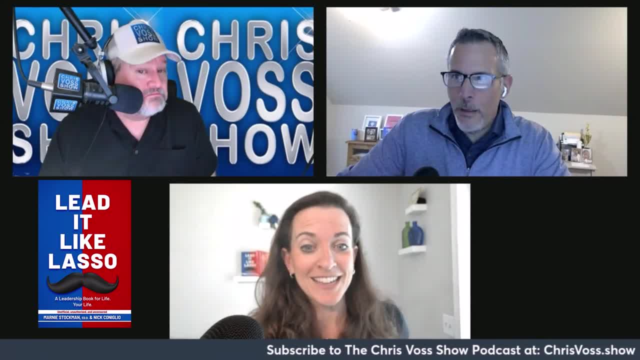 Working for the Rupert Manions of the world. if I can say that I don't want to interject that. That's the bad guy in Ted Lasso. That's the bad guy in Ted Lasso, The guy you don't want to work for. 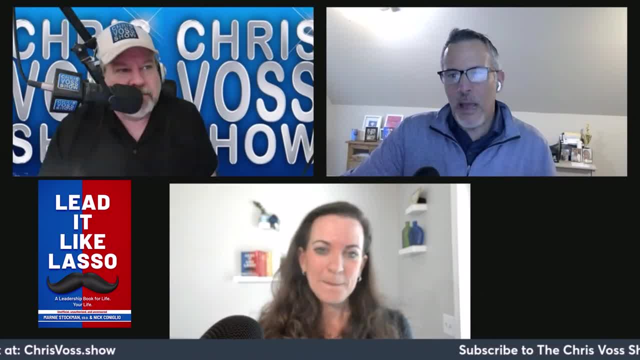 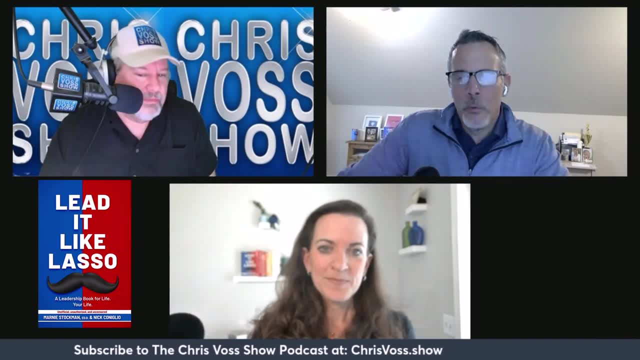 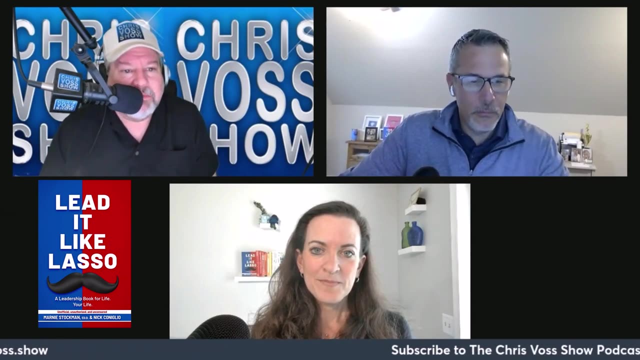 Yeah, But they they really started. you know we felt a clash right Their core values, that what they stated publicly was all about building raving fans with their customer base And Marnie and I were responsible for those fans. She managed customer success And part of my responsibility was customer support And we realized that the latest company that acquired us 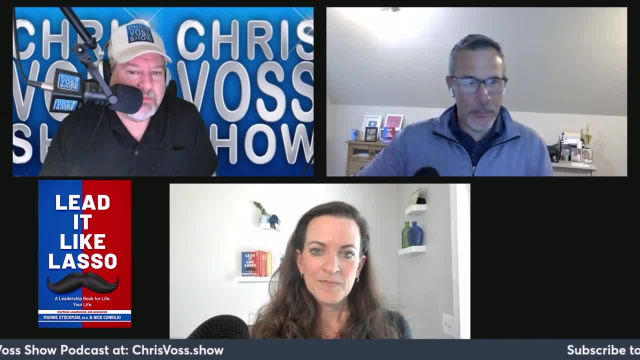 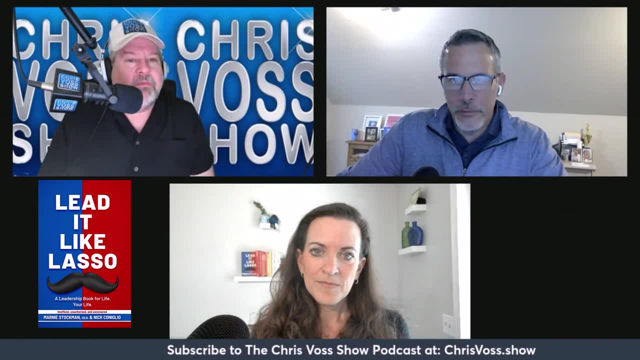 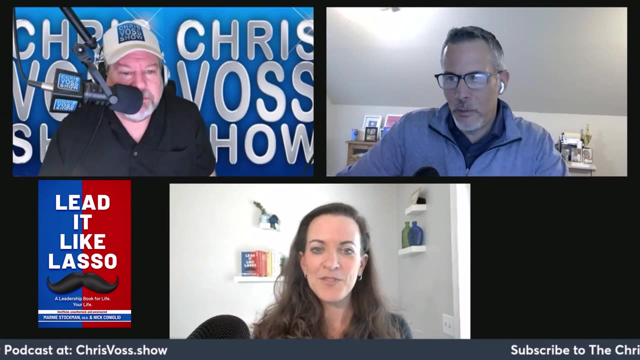 And we realized that the latest company that acquired us was dumping all this money into sales and cutting back the staff on the people, that the account managers, the success managers, the support team that were supporting these customers, And it was resulting in exactly the opposite of what their stated message was. 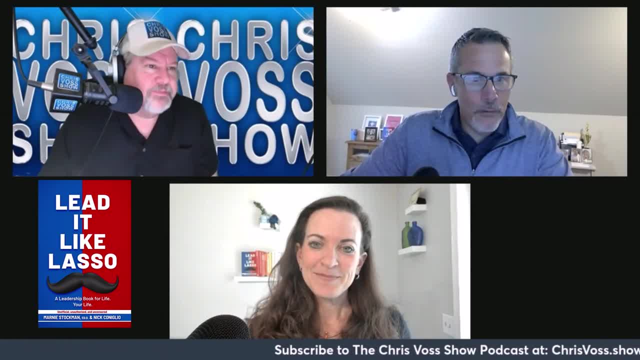 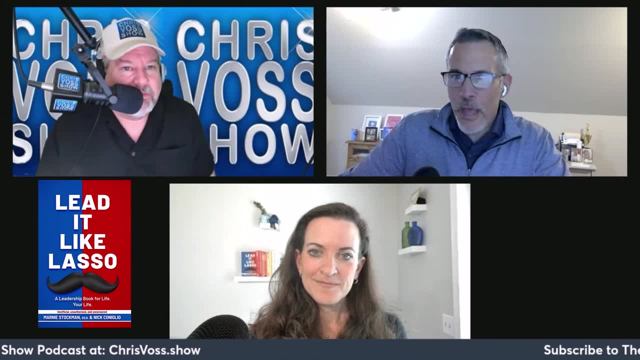 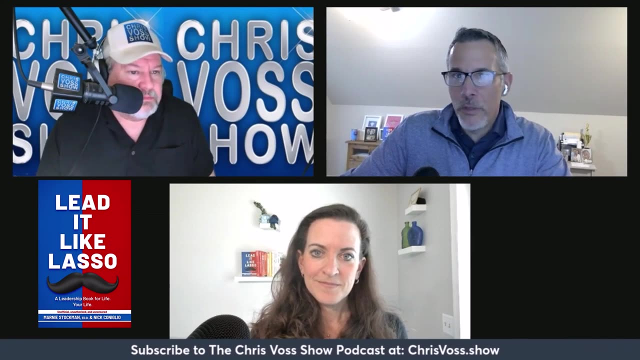 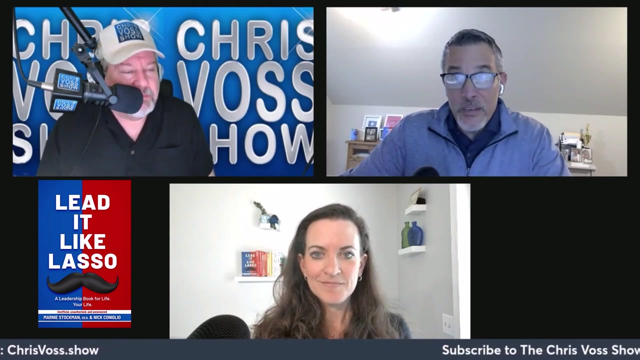 Lack of success? Yes, So we had. we had to come up with a way to fix it with limited resources, And we developed an operating framework, a business operating framework that was successful within this company. But we- really we- decided that we thought we can do this outside this company on our own, And that's that's kind of how we got into starting our business, which is a bit different, because many people start a business kind of with a product fit in mind. They have a business idea. 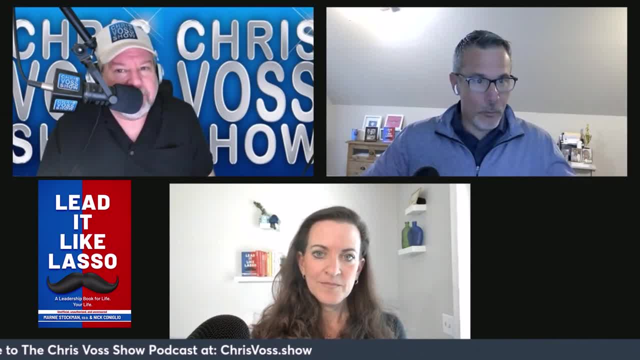 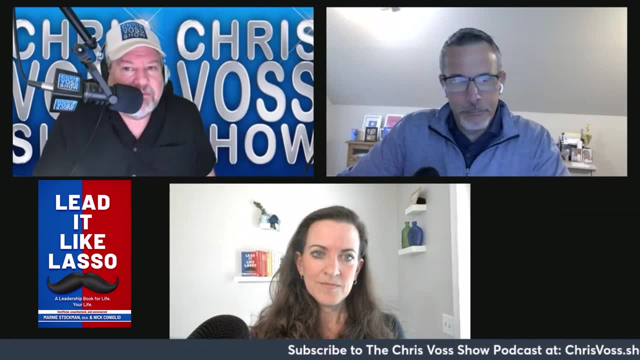 Yeah, We didn't at all. We started with an operating framework. We said: these are going to be our core values, This is how we're going to approach this, But we had no idea what we were going to do. You know, that's so important. 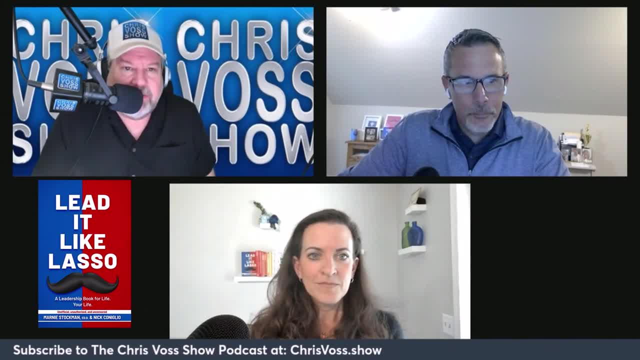 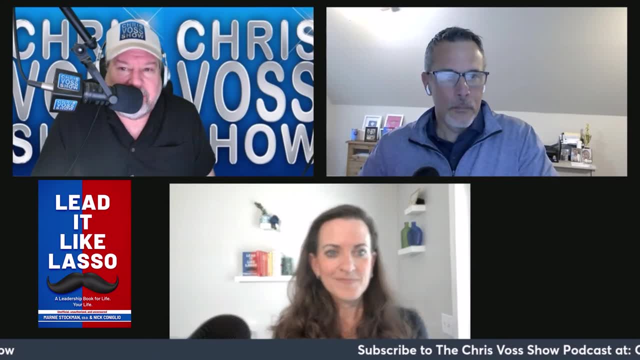 You know I I had read a lot of books preparing to be a CEO. I started a small, a few small companies when I was young, but then I I never gone to college, So I knew I had to develop my own MBA type thing. 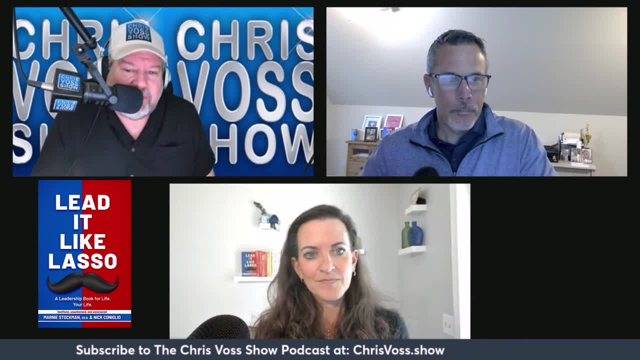 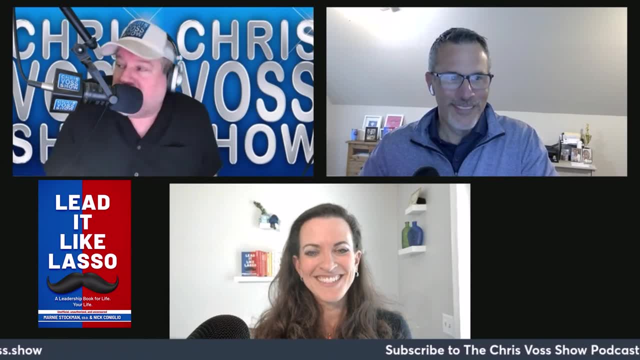 And so I studied a lot of Harvard business review And one of the big books that have impact on me was usually Tom Peters stuff. Although about half his stuff reverse engineered, maybe bankrupt, The other part made me rich. But sometimes you know these, these folks that are wonderful, like Tom Peters. they 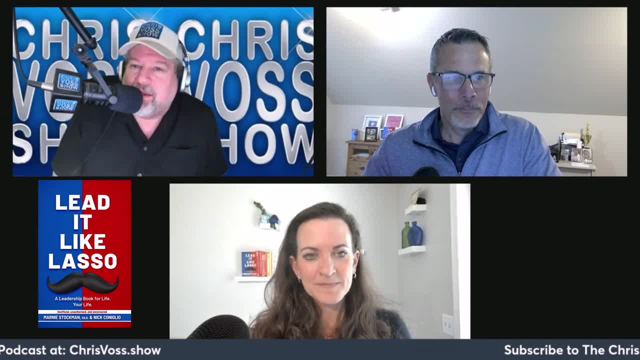 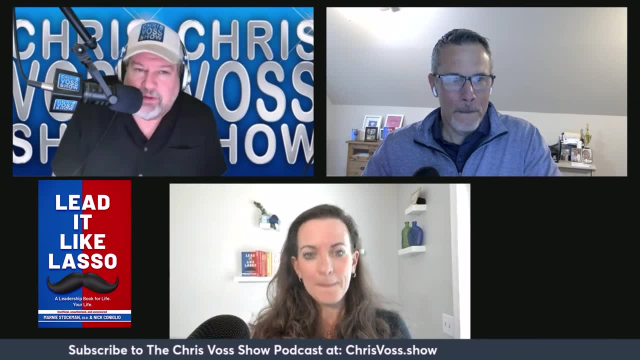 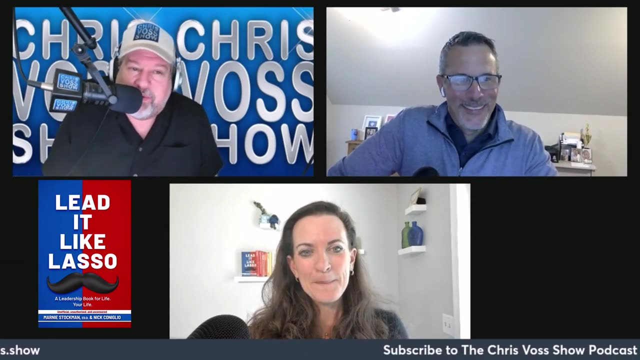 they reverse engineer how someone was successful and they and then they get the magic wrong. but the big thing that had to impact me was peter singe's book, the fifth discipline. my audience is like god he's gonna go into it again. but the fifth discipline taught me about building culture and over harvard business. for 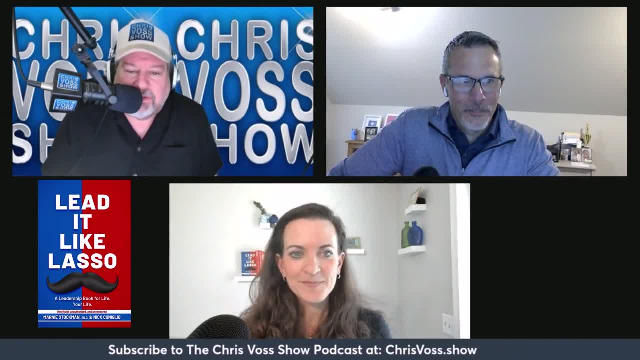 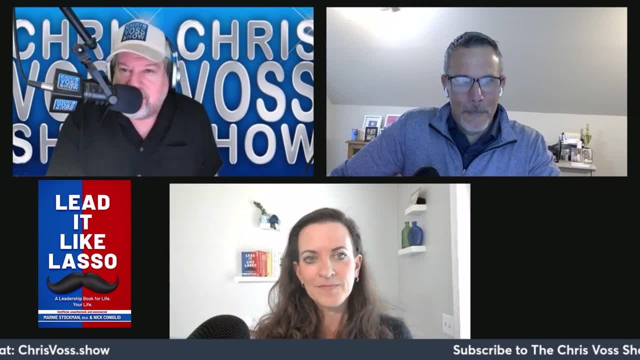 you and tom peters and other great authors, i learned that culture is so important and injecting that in the moment you start your company and having that, that vision, like what you guys talked about, how you wanted to make sure that you manage culture and the vision and 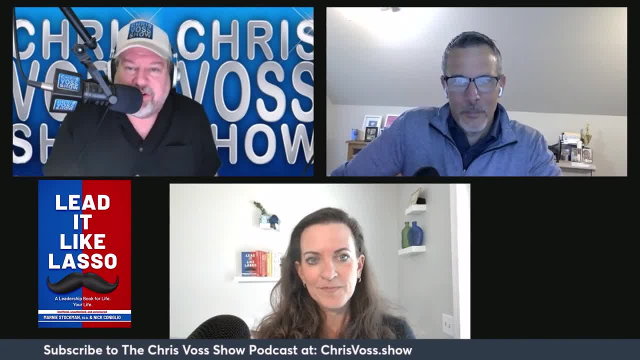 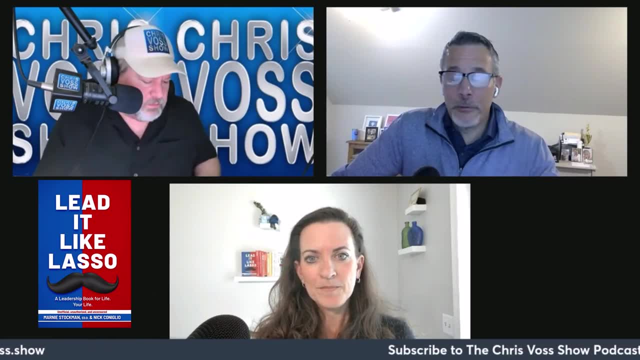 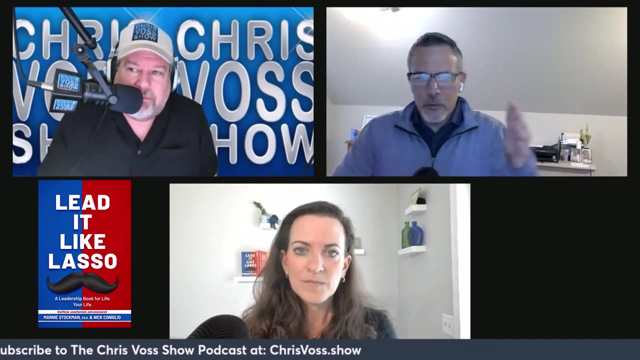 and all the stuff that went into a business first, so you can lay that foundation and build something on it. that's so important, yeah, yeah, and, and more than absolutely- and we live with culture, but it's it's also. i think one of the things that frustrated me just as my career evolved is especially in 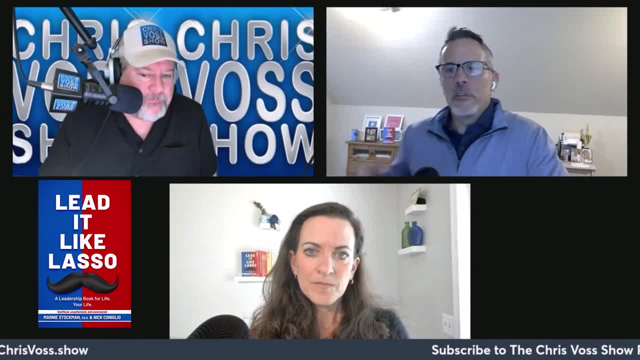 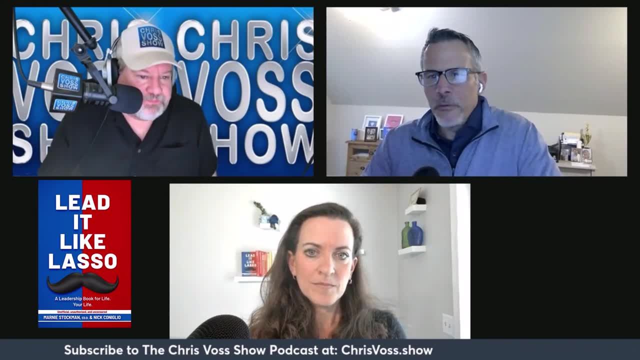 technology i would work with so many people who would focus just on their technical skills and ignore kind of their professional and character skills and it. that was so frustrating because all the folks i worked with that excelled really focused on both the metaconscious efforts, grow their 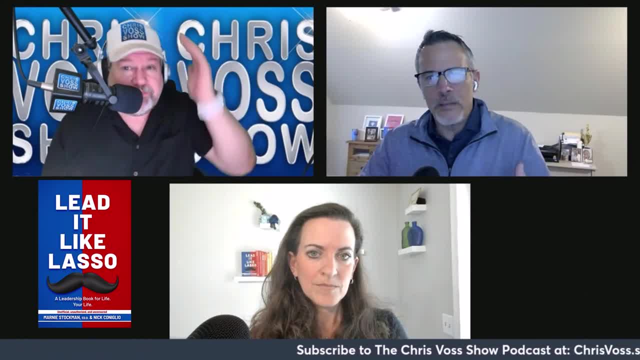 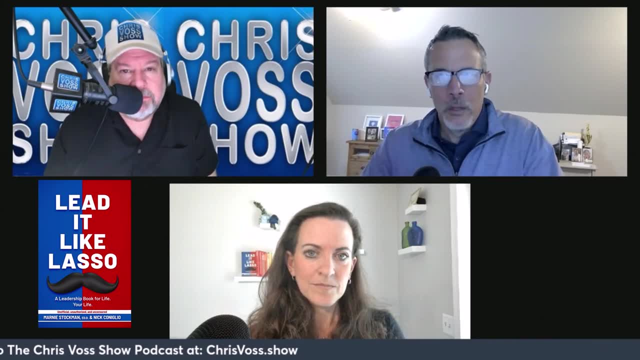 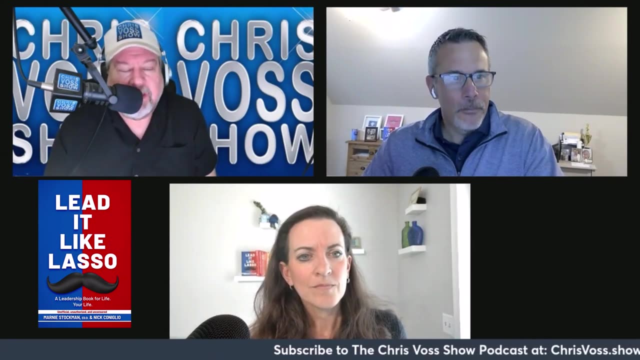 character skills and it just said it felt like such a waste of talent and and so, in addition to the culture, i think it's really important to talk about character skills, and that's that's what we try to outline in the book. i would agree with you, yeah, yeah, sorry, it's so funny how you. 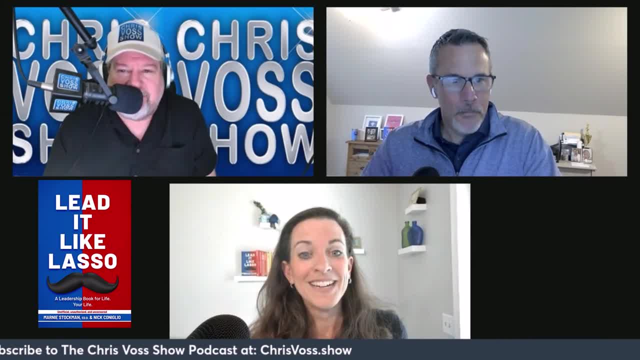 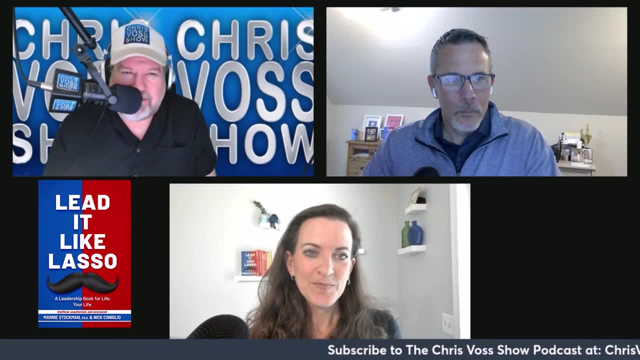 i'll ask so many leaders: what is your leadership style? i don't know. yeah, yeah, a lot, a lot of people i've had on the show that advise you know leaders. i'll ask: do you? do you? do you get the same answers? i do like they don't know. they. they have an operating system. they usually just don't know. 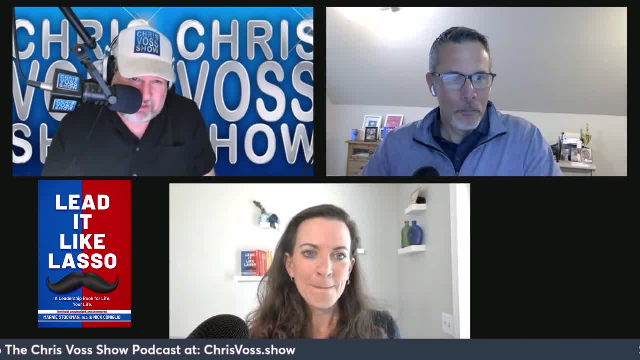 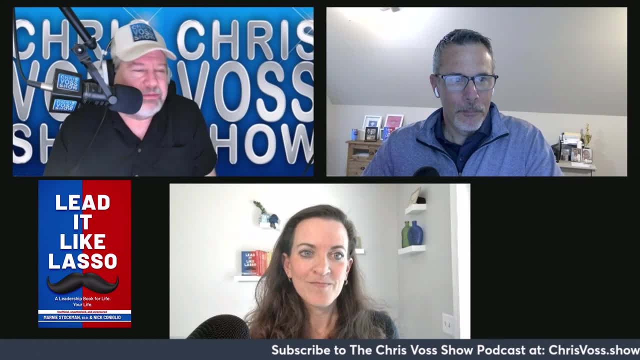 what it is. they're flying on a subcontract. they know their toolbox. they just don't know their toolbox, which is interesting because they haven't been intentional about it. it's just kind of, i guess, developed by default. yeah, and it's interesting that there are tons of assessments. 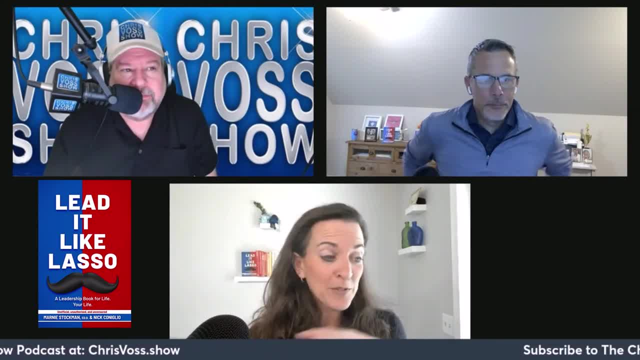 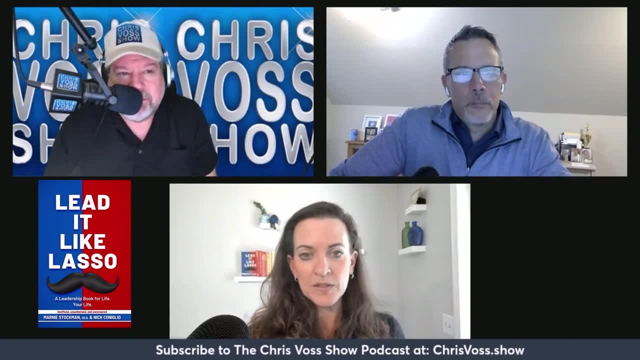 out there to determine leadership style etc. and and everybody's got their favorite and it really doesn't matter which one you do, as long as you focus a goal on working to improve the places where you have weaknesses. so in the book we actually created an assessment of the five main. 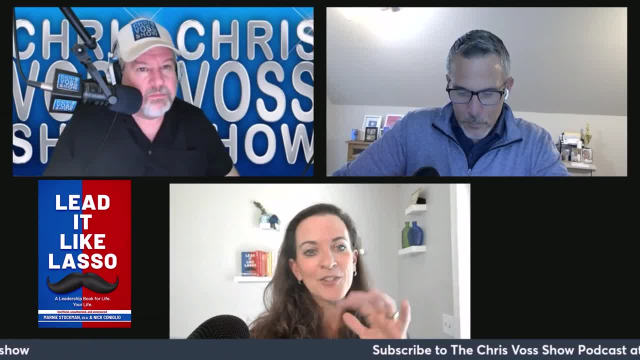 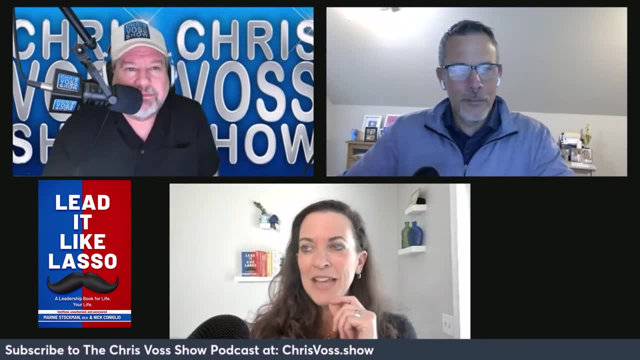 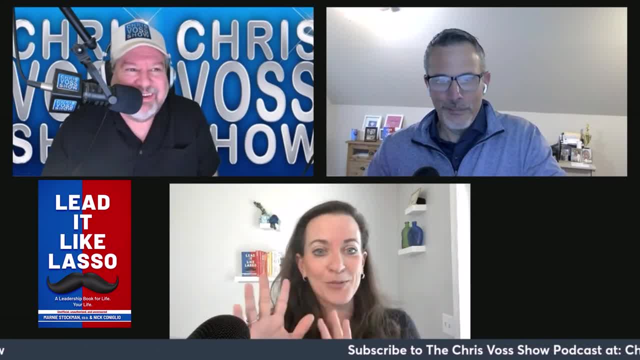 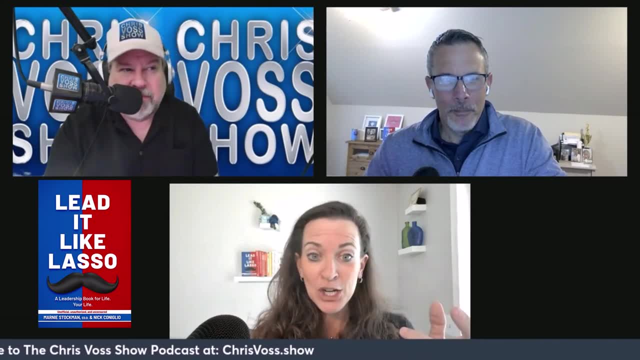 Facebook post: oh my gosh, I'm a Sam Obasanya or Roy Kent. he's my spirit animal. So it's a lot of fun to have people think about which character they would be And, in the show, part of the secret. 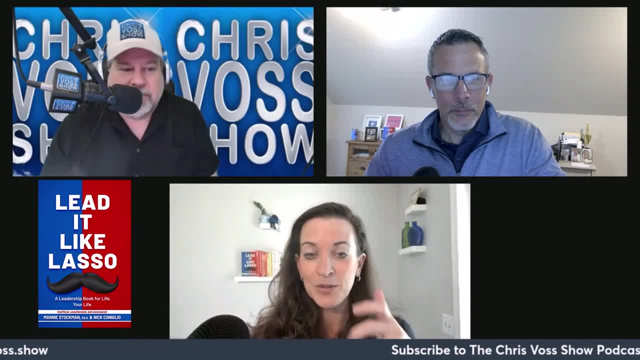 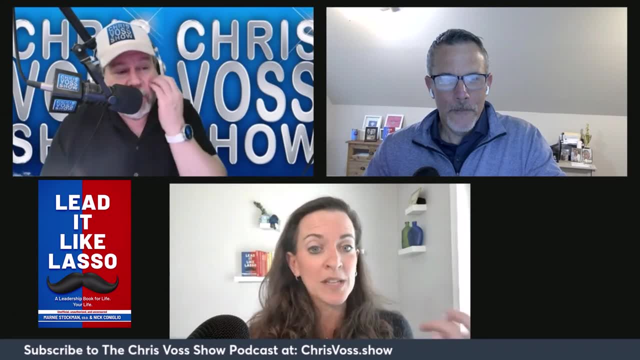 sauce is the assistant coach and coach, Ted Lasso, give books to each of the players to help them become the best version of themselves, And in the book we say: these are the books we would give the players if they were aiming to be a leader in business or life. I like that how you have that. 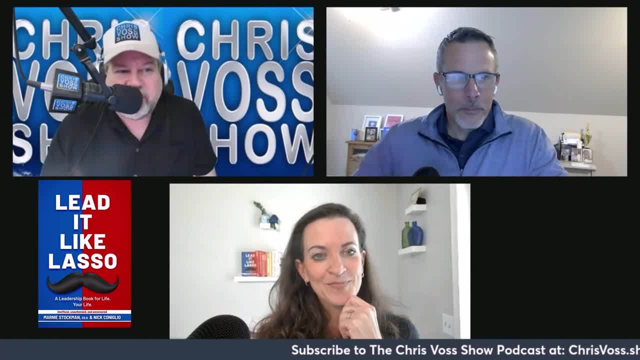 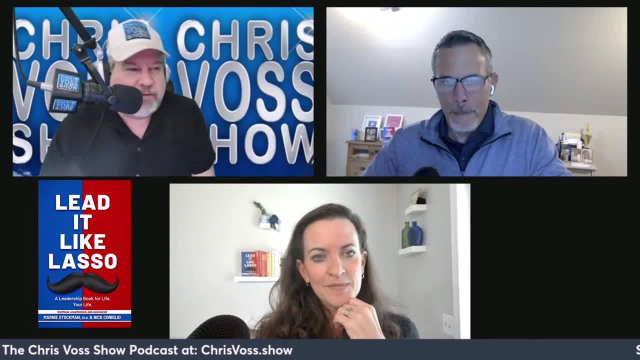 alliance with those characters, because then anybody who's watched the show can put them together And I think it makes it easier for them to understand, maybe because they can see it play as it was played out through the media And we parallel it with real life leaders as well. 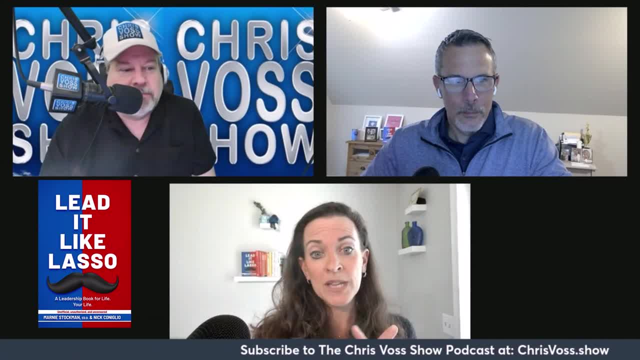 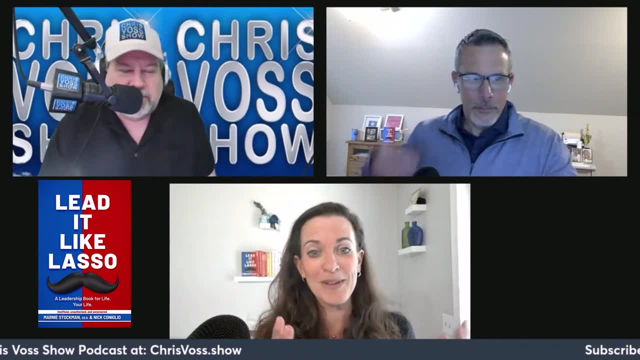 But for them, as Nick was saying earlier, the show is so relatable. I mean, you watch the show, you want to be better, You want the world to be better. It's really inspiring, which is why there are so many millions of followers of the show, So for folks to be able to see themselves in. 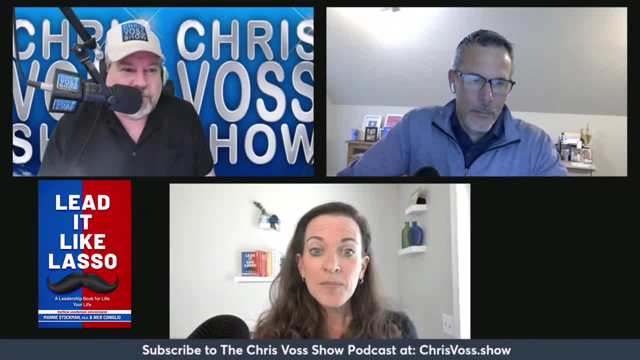 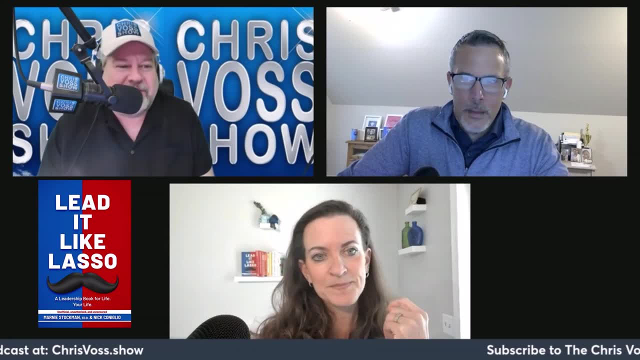 those characters, we hope gives them not just the wish to be better but some actions to, to you know, improve their skills, their character skills, like Nick said. There you go. You know, my employees have a TV show that they use to ally, who I remind them of. 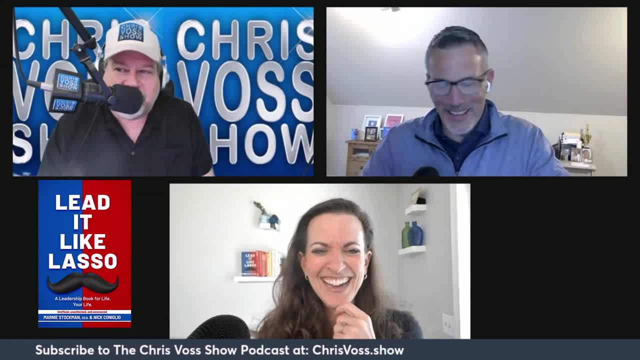 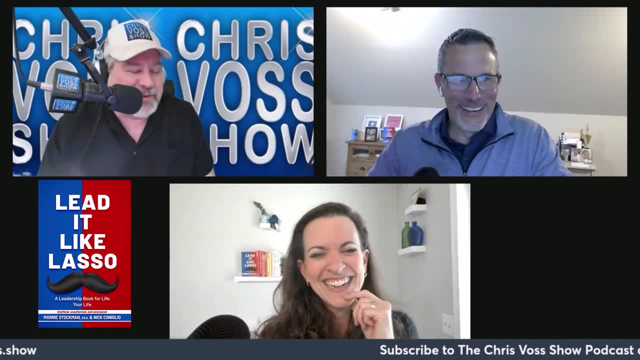 It's usually from the office. It's Michael Scott. I was going to say: is it going to be the officer of Parks and Rec? I'll dodge and I would love to be the character from from Parks and Rec. Who's? who's the guy? 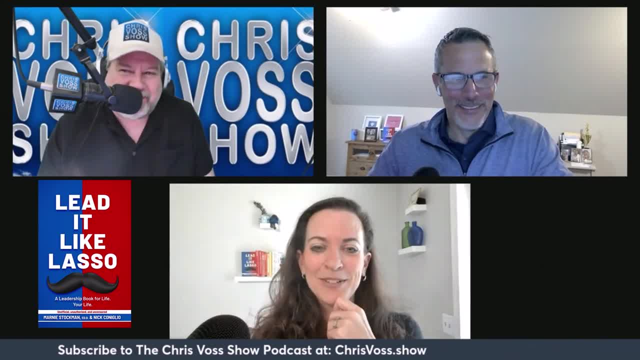 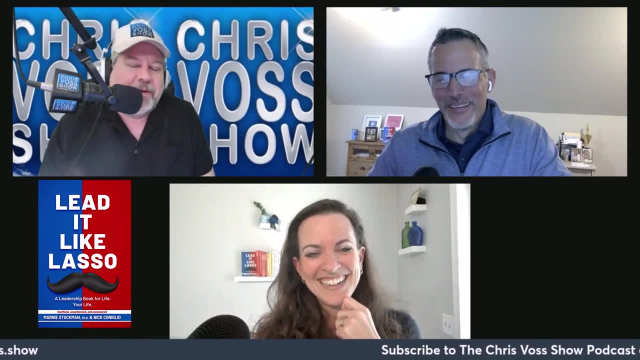 I know I don't. I don't know who his name is, but I know we're talking about the same one. I love that dude. They think I'm Kevin Malone from the office, One of those two, maybe both. It's a mixture, but, jokes aside, I think so. I noticed something on the website. 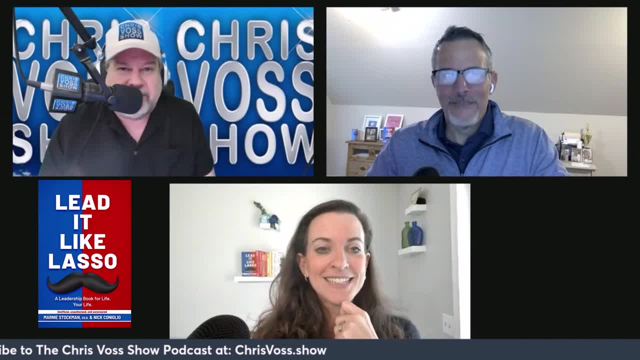 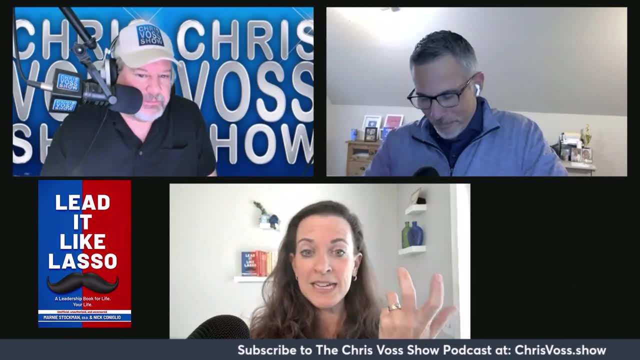 There's a pop-up of the real Ted Lasso. Tell us about that interaction. Yeah, So, on mom, on Monday we're having we're having a webinar with Lee Elias, who is so part of Ted Lasso's thing, as I mentioned at the beginning, is he left the United States. 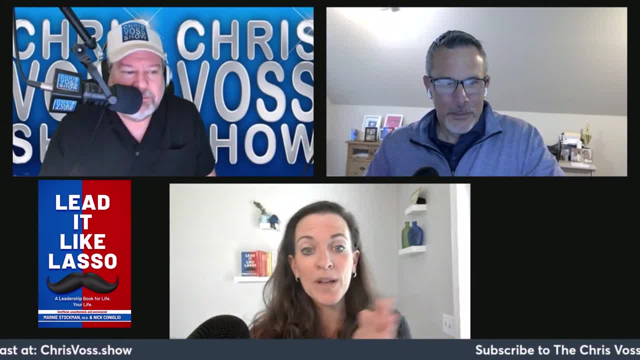 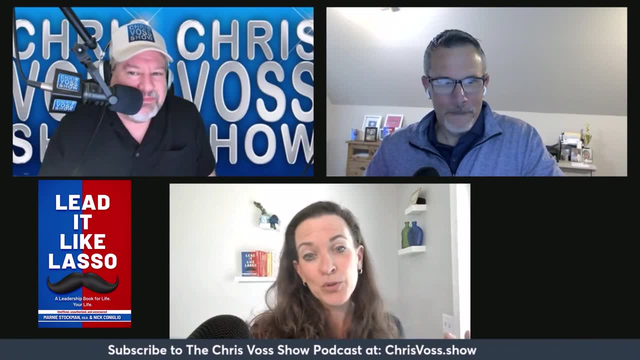 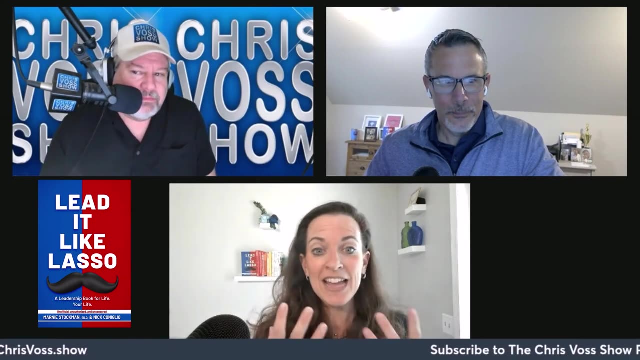 and went to London and coached for three years. So Lee went to London, coached hockey for three years in a world he didn't know Right And was extremely successful through team building skills And he is a team building coach and strategist And so he feels like everyone was tagging him and commenting to him after the show of. 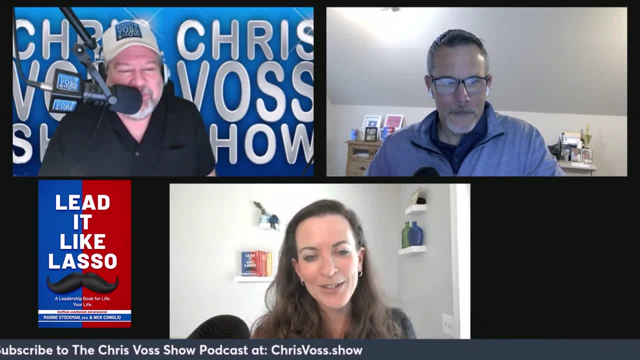 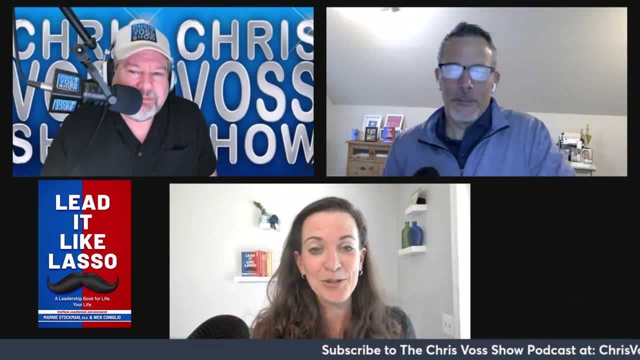 oh my gosh, you are Ted Lasso. He has quite a following on social media because of his team building, So he's not related to the show other than he just feels it in his heart, Like I'll assume many others do. There you go. That's gotta, that's gotta be a pretty good show and a pretty 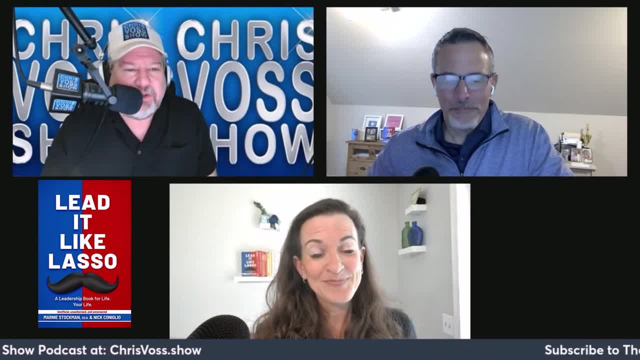 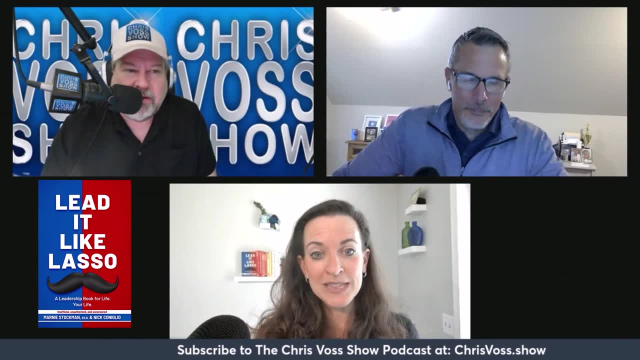 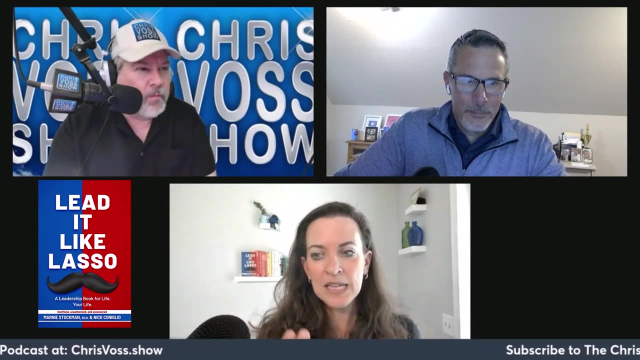 good gig for him to back up. you know off the show And did you interview him for the book at all? Is he in the book or are you just doing this post interview? So we met him right after the book released. I we were on social media and I found one of his books and we reached out to him and 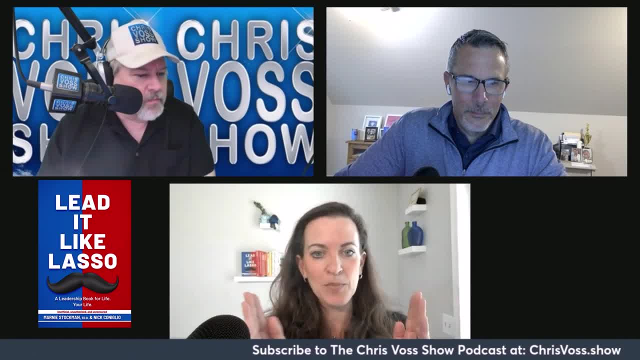 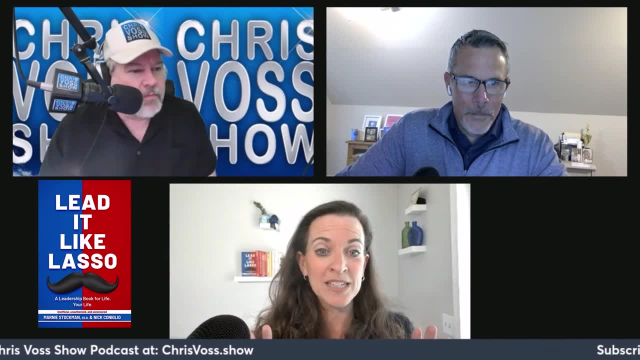 said and just exchanged backgrounds And we both thought: oh my goodness, you know, there are a lot of similarities. So Nick and I looked at his book and he looked at our book and it's, frankly, a good thing. We- neither one of us- knew the other before we read the books, because we might've thought the other. 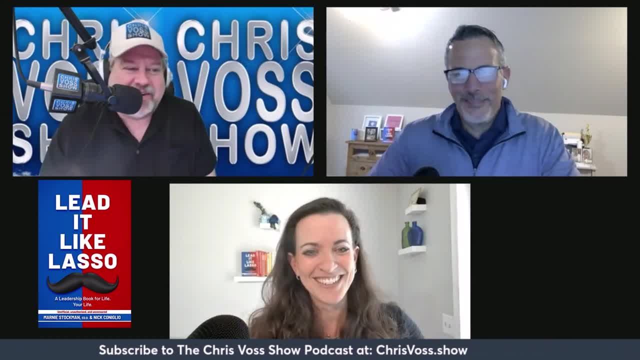 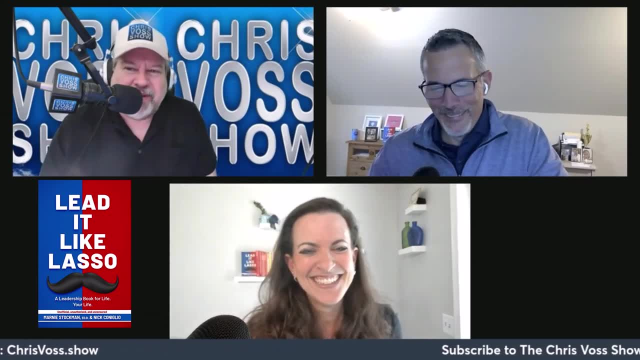 one was copying our style, our tone and strategies, Oh, then you have to sue him. Not a very Ted Lasso thing to do. My, my, my, my. people who think of me as a TV show, think of the guy. any show from Dateline: 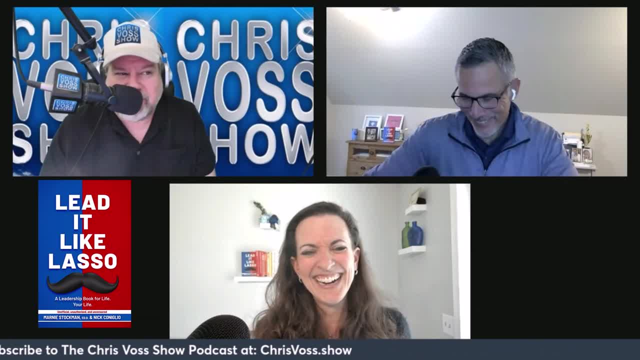 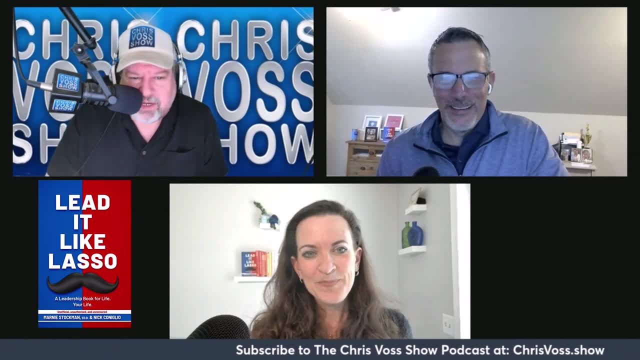 pretty much. I don't know what that's about, but I'm sure the judge. we'll get to it later. So in the book, give us a few strategies that you guys are some of your favorite strategies for what people should do to you know. get their leadership down for their 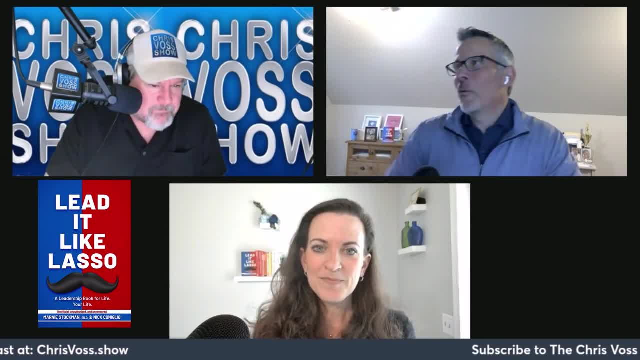 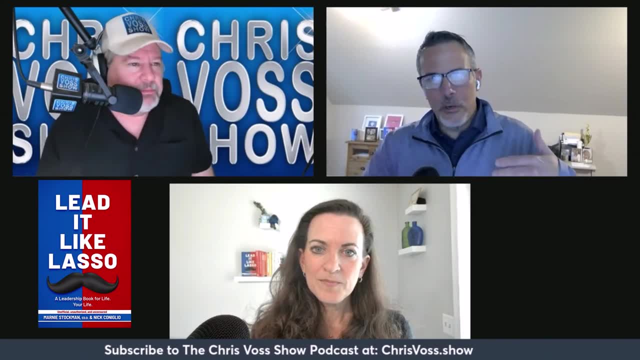 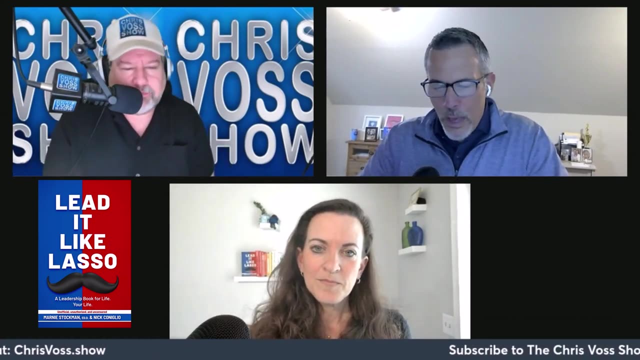 lives. Yeah, I mean, I think so, unlike a lot of leadership books, and we talked about this a little bit earlier, but but we start off. instead of starting off with vision and purpose as part of the, as kind of the, the foundation of the, of the framework, we absolutely start off with core. 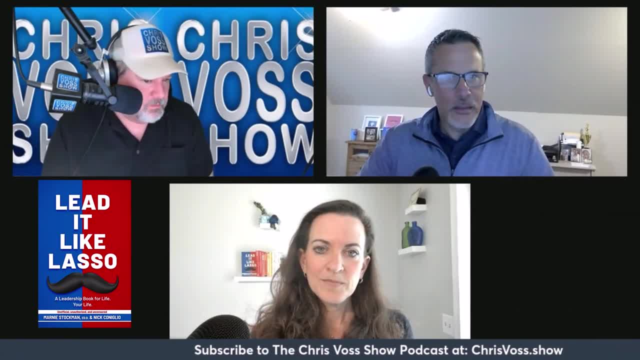 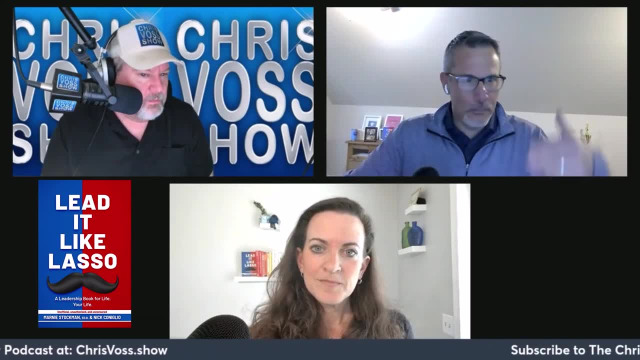 values, And to us it goes back to the whole authenticity thing. right, You know I struggled a lot early in my career with imposter syndrome. right, I happened to be in a position where I kept getting promoted and promoted, and promoted and being put in leadership position And I really felt like a 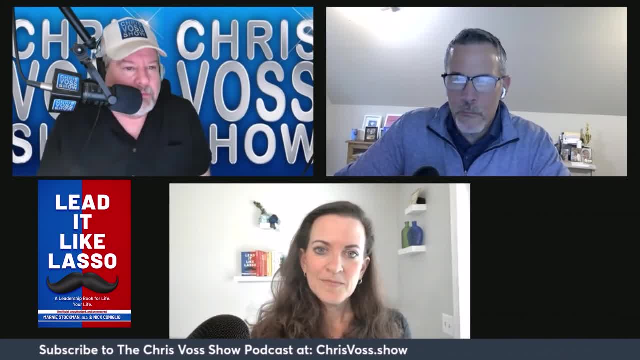 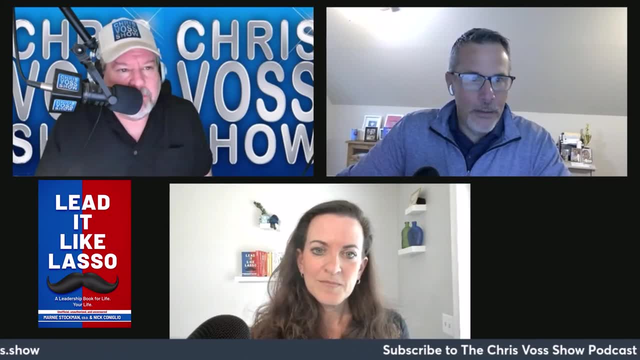 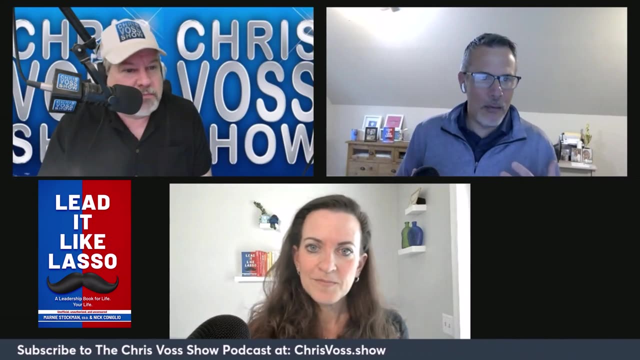 fraud And I think part of the reason for that- I know part of the reason for it- was I didn't take the time to do the introspection, to figure out what my guiding principles are, Right And and that seems straightforward And easy- you know, I know who I am, but time after time we would run across people who really 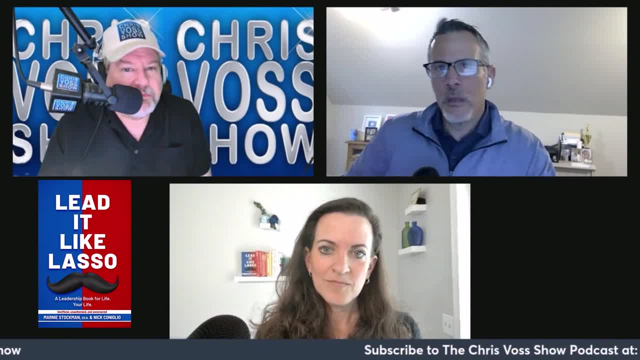 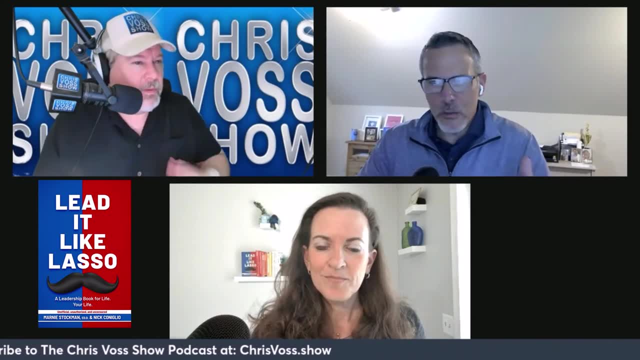 don't know how or really haven't put much thought into what their, what their core values are, And we help them do that. And I think that's just the first part And I think just in general. I don't let Marnie talk about some of the other activities that we have, but one of the 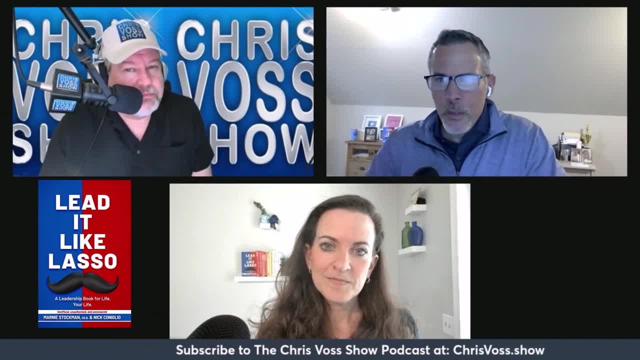 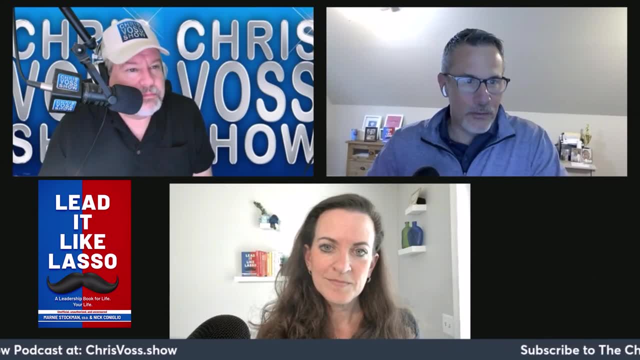 the other things about our book that we should have mentioned up front is: we don't just- we don't just- outline our framework. We don't just outline our framework, We don't just outline our framework. We provide activities for people to actually execute on it Right. So, whether it's it's 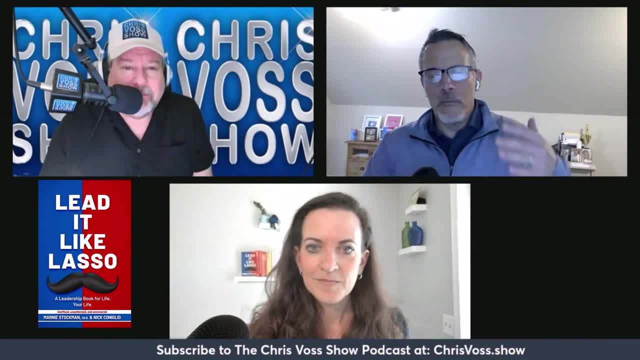 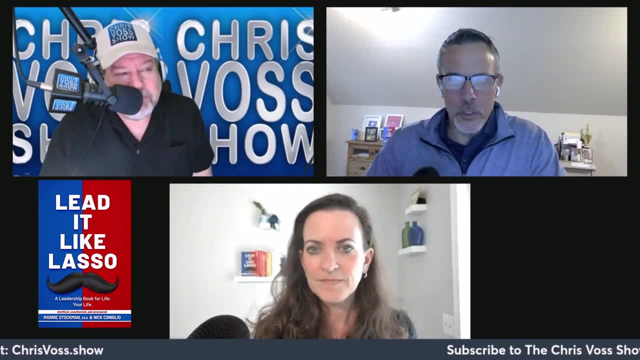 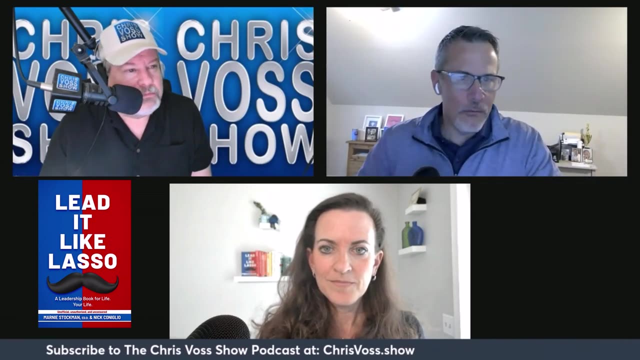 identifying your core values, how to establish a vision and then goals that can be tracked to that vision. You know we have the whole notion of we. we feel it's very important, as you define your vision and you set goals, that you should have guide rails. So we talk about. 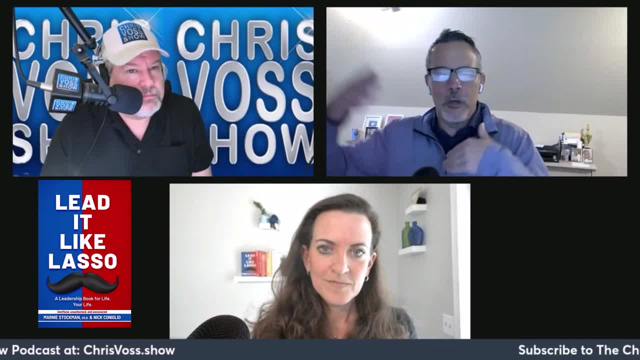 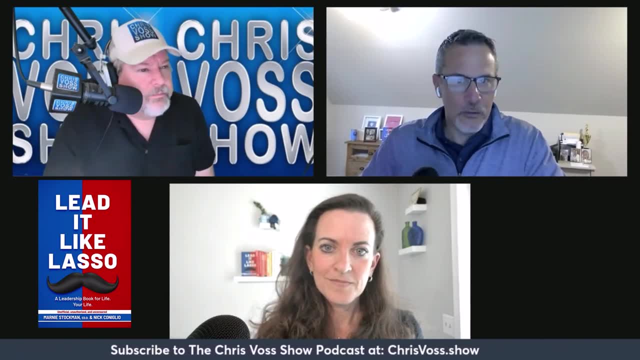 different strategies around projecting where you're going to be in the future And exercises to to really put those guide rails in place. So if you get, if you get knocked off, course right, And you know who doesn't right When, either personally or in business, you get. so 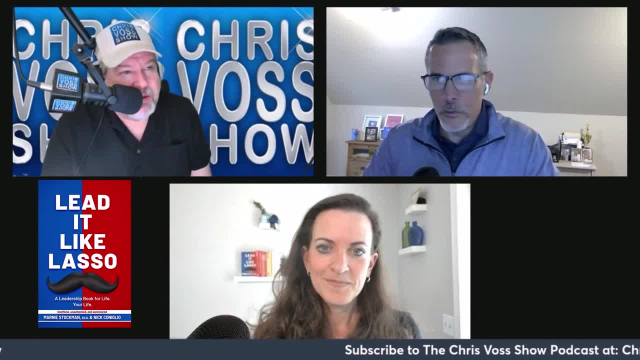 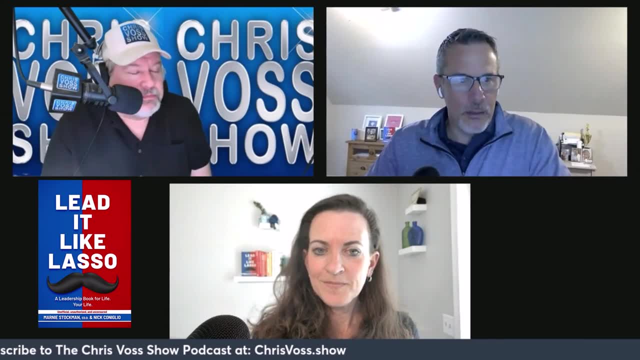 involved with the day-to-day. sometimes you, you, you, you lose where you you ultimately want to go. but we provide activities that that help you keep on track and execute the framework, And some of those are a lot more simplistic than you would think, Like you mentioned. 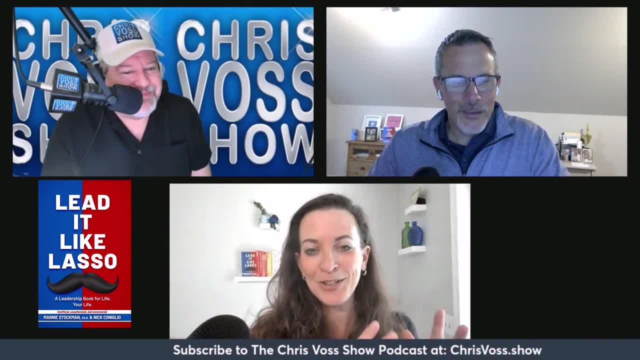 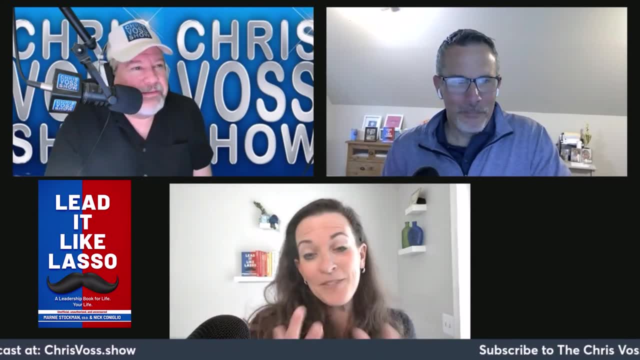 you don't always have to do the, the Harvard MBA, to learn a lesson. I mean, we put Mad Libs to a whole new level with a very fill in the blank. Let's do some brainstorming. One of my favorite activities is at the end we basically have you. 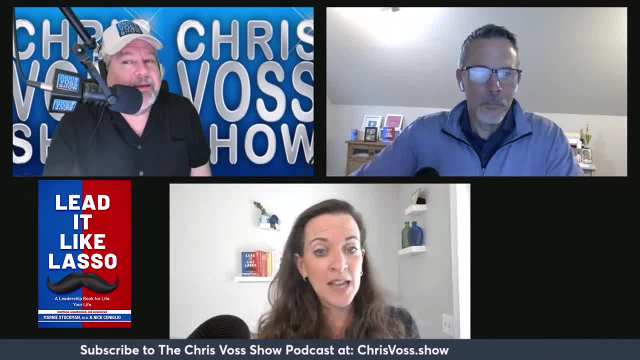 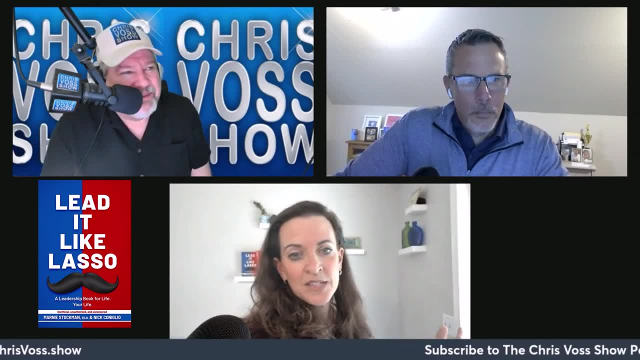 Mad Libs, your retirement speech. So you could say I'm Chris Voss. and here you know, at age whatever, this is my retirement And these are all of the things I've done. And those are the guardrails that Nick is talking about. If you can really define for yourself where you'll be in the 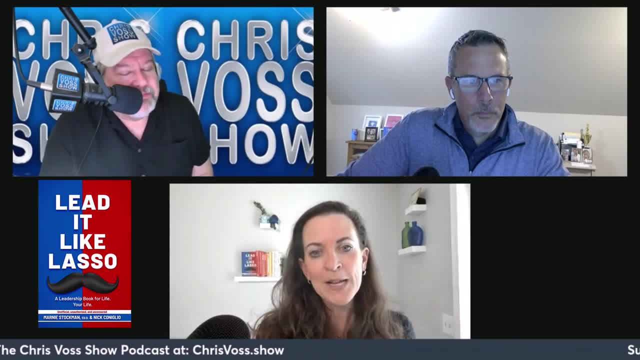 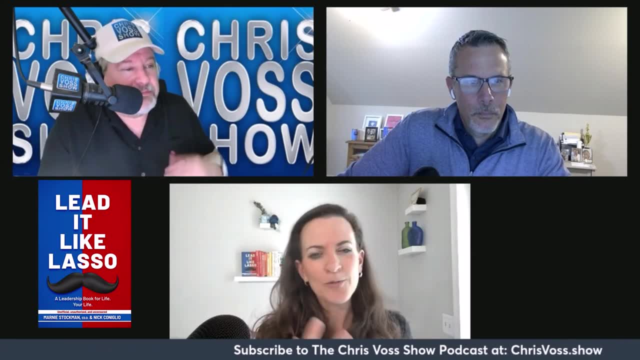 future. it helps you make those decisions, Yeah, Along the way. So they are serious outcomes that get delivered from the activities, but they are thoughtful and easy and fun to do because you're really thinking about introspectively what are your core values, You know. 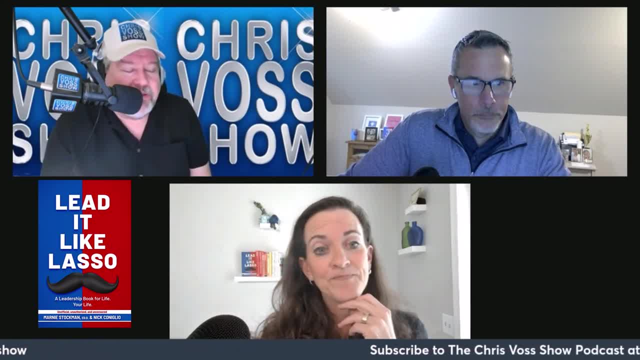 There you go. So it's like a workbook, where you've got the learning and the workbook to help you really cement those activities. Exactly I. you know I read a lot of books and you know there's always books like mine that you're just. 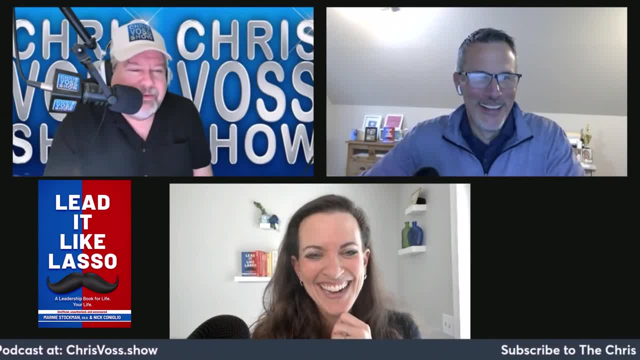 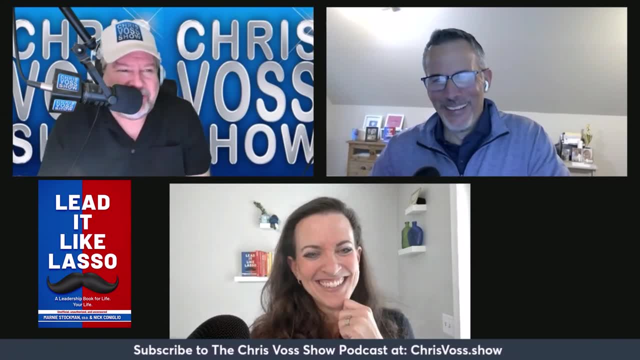 like Hey, you should do this and then have fun with that. So hopefully, do them, Good luck, Good luck. a little trooper, Even Peter Singe in the learning organization, I think the fifth discipline he had to put out a. 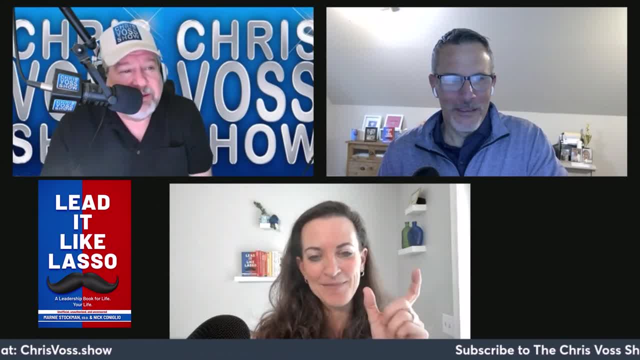 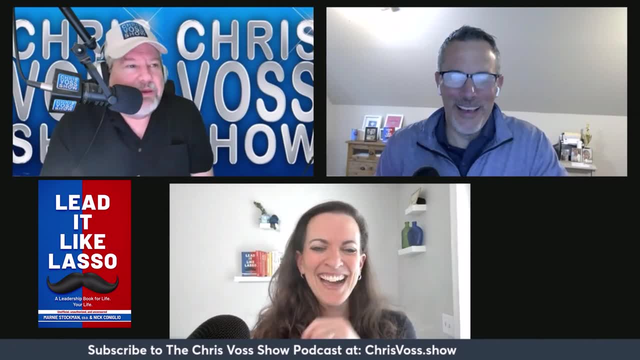 workbook on the second one. So he did I. I have both the accompanying books on my shelf. So yes, In fact he owes me a couple of checks at this pace. You know, I was going to tell you the one way that I found to overcome imposter syndrome. You know what it is. 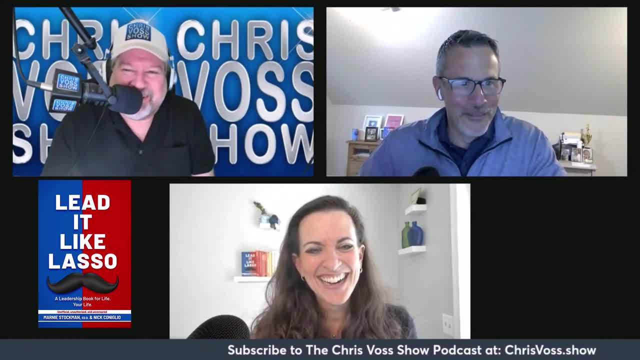 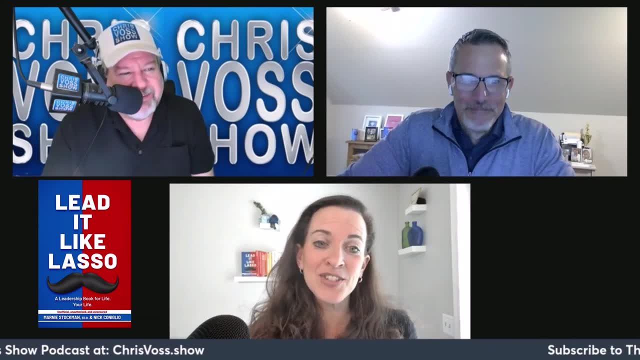 No, I wish you were. you were telling me 25 years. I don't know why I'm setting this up this hard. It's totalitarian egotism and narcissism. Oh yes, Those do. They will crush some imposter syndrome for the win. 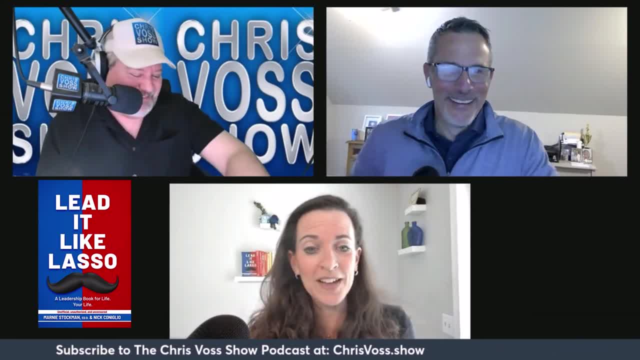 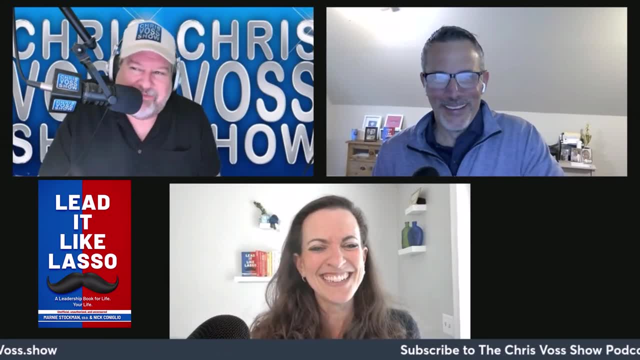 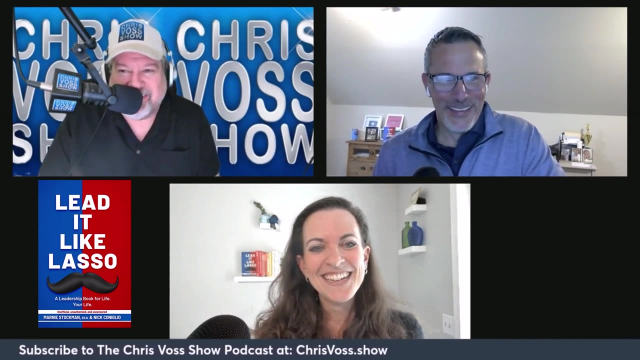 That's why I never had a posture syndrome. We already know your core values now, So that's great. I'm full of shit up to my ear. That's not what your book said your core values were, but that's okay. I had a PR agent write that, maybe, But no, my audience is sitting around going. yeah, that's true. 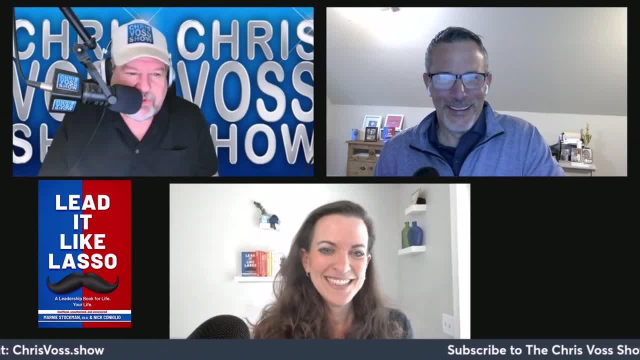 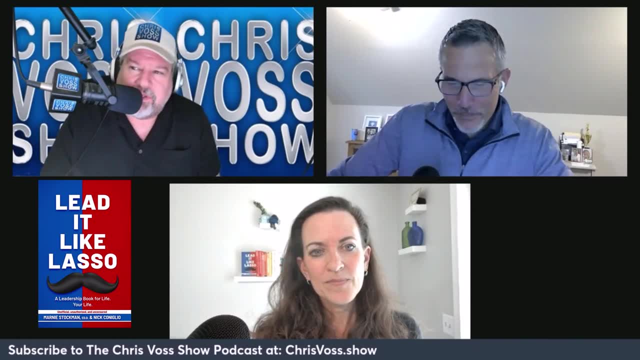 He's not fooling anybody. Any other tips and tricks that are in the book I thought it was interesting. You, you talk about vision. Vision is so important for leaders- And then there's a lot of other things that I'm seeing on your website. You talk about empathy, compassion, loyalty, fun, teamwork. 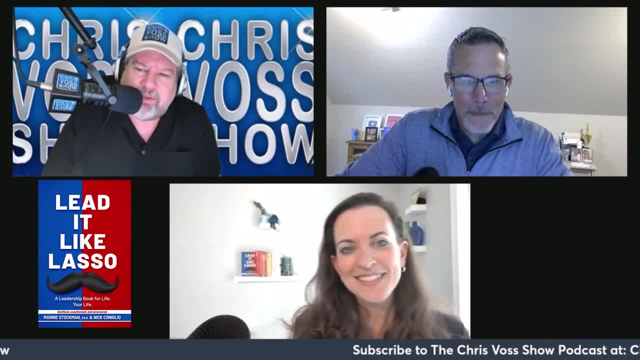 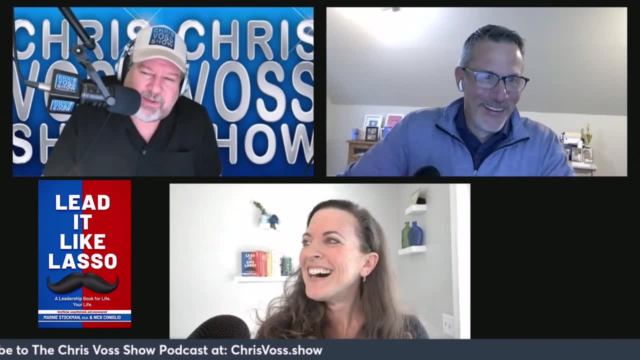 achievement, growth, honesty and a few other things. What the hell are these things about? I just totalitarian, totalitarian, authoritarian leadership is my style. Empathy thing You mentioned, yeah, empathy, which Ted Lasso was very empathetic in the way he dealt with it. 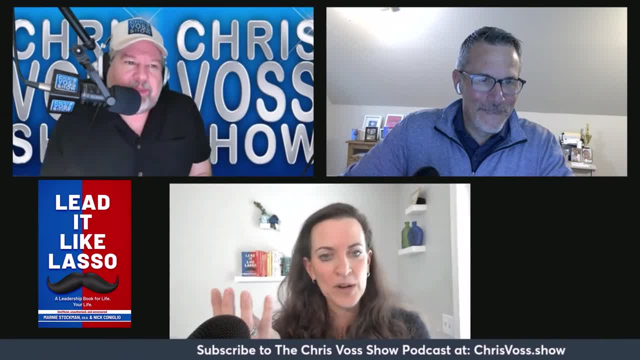 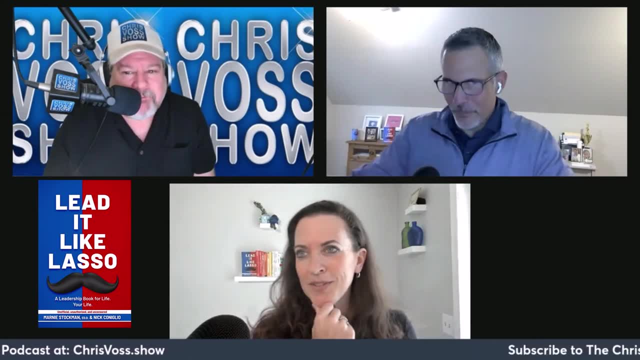 He was very empathetic with all the characters and it's really acknowledging taking everybody from where they are to where they want to be in an understanding way when you read. So that is the soccer field we have on our website, with some core values as folks can select of their own. 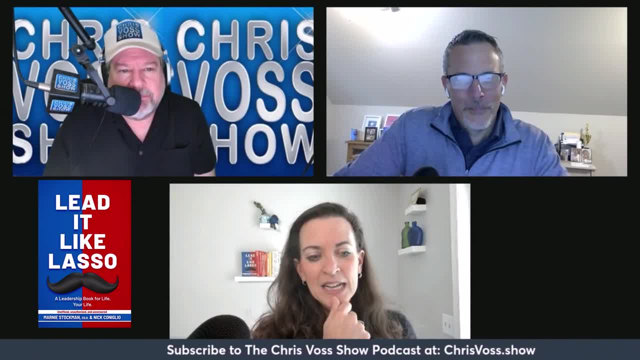 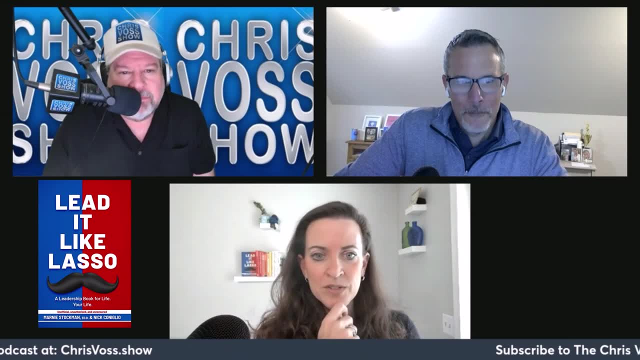 But you mentioned one which is fun, And while we took business seriously, obviously like we aimed at the beginning, we said we're going to grow a business in three to five years to sell for 10 to 15 million. That was our goal, But we also didn't take ourselves too seriously. 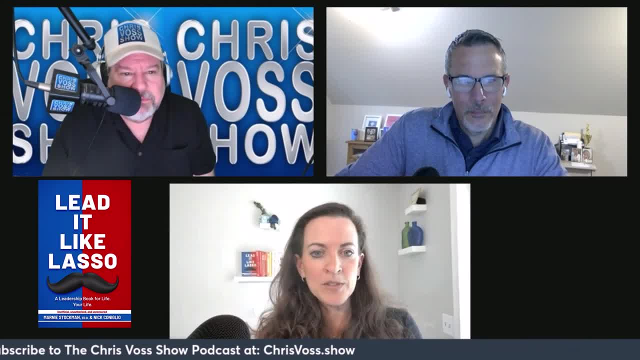 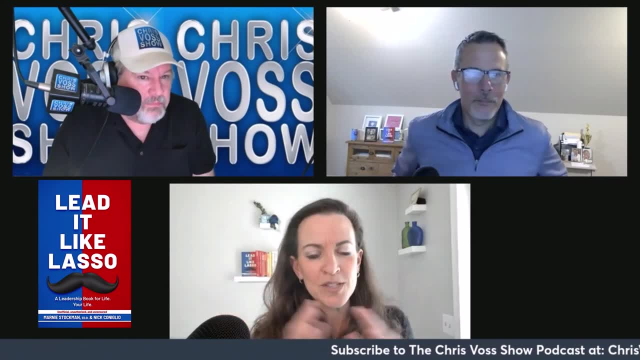 So our company was called Lifecycle Insights and we bought the domain lifecycleinsightssucks And we had our partners write one-star scathing reviews about what they hated about us, And they would say things like: I have to pay so many taxes because I'm making so much money with your. 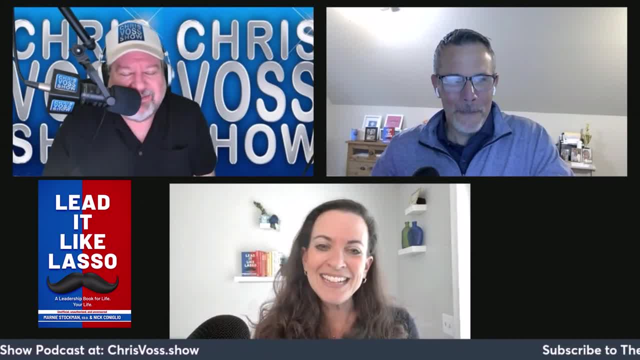 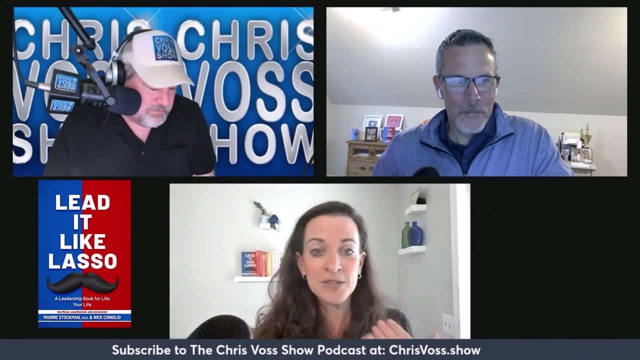 software, you know like, really mocked us the whole way, And it's not what it when we say. fun was one of the you know our strategies. it was not that we had ping pong tables in our office because we all worked from home, Ted Lasso. 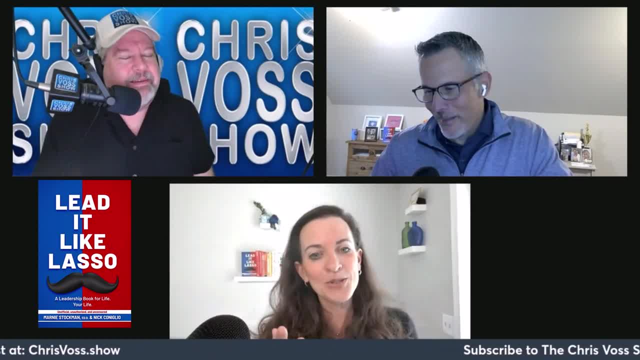 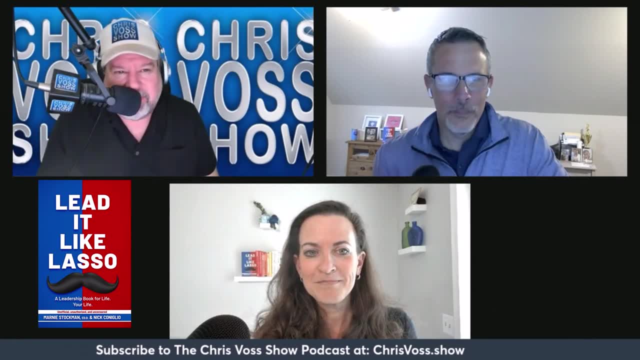 And only one of us had a ping pong table. but we would do, we, we, we didn't take ourselves too seriously And our messaging was really light and fun. Mark Leary, Maybe you should have a ping pong coach come out for this. No, I'm just kidding, Sorry, Here's a. there's a few quotes, I think. 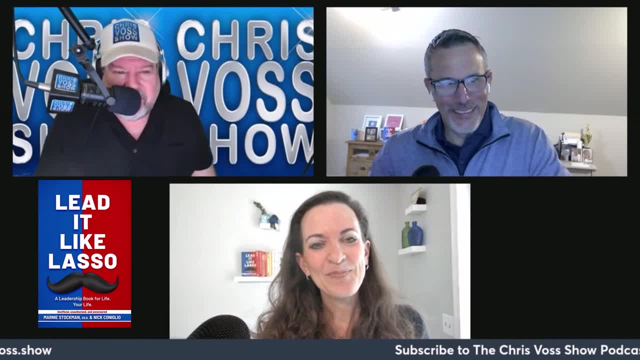 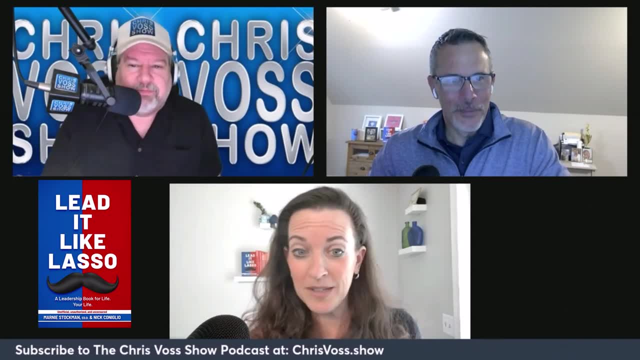 that are from the book that I'm reading on your website. Here's one that's a favorite. I'm not sure why A vision is a beacon that leads individuals or organizations towards a higher aspiration. I love that quote, Ted Lasso. It could be that you wrote beacons of leadership. 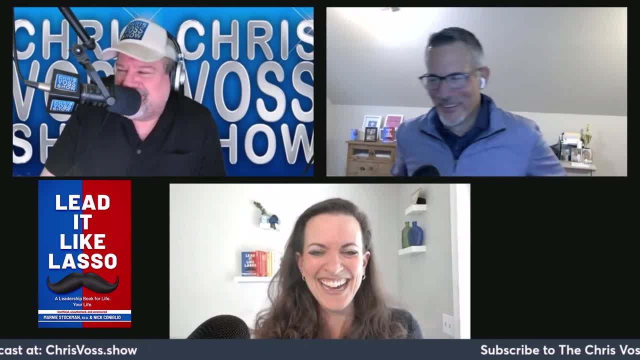 Mark Leary, Is that what it is, Ted Lasso? Mark Leary, Is that what it is, Ted Lasso? Mark Leary, Is that what it is, Ted Lasso? Uh oh, we're getting sued now, Ted Lasso, Shameless, plug in there. It's my show So. 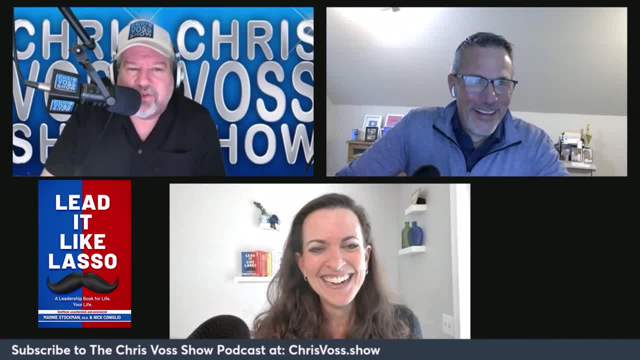 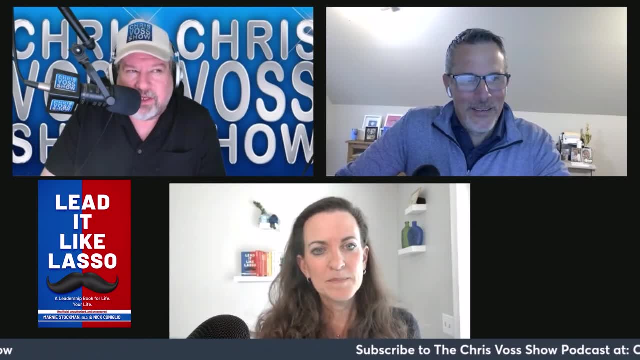 you know I'll pay myself for that one. This is an interesting one, though. Leadership isn't a title, It's a way of life. I can't remember if I talked about this in my book, but I used to have a picture that sat on the edge of my desk when we really were starting to hit scale, And it was a. 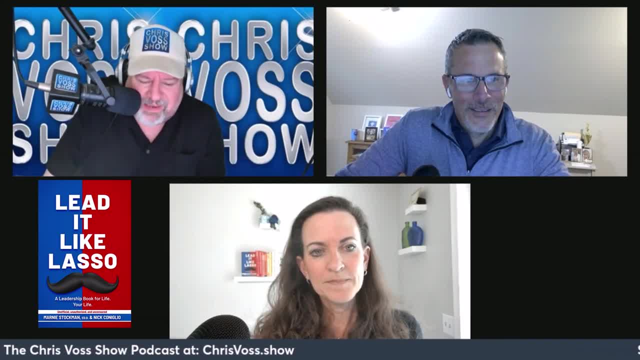 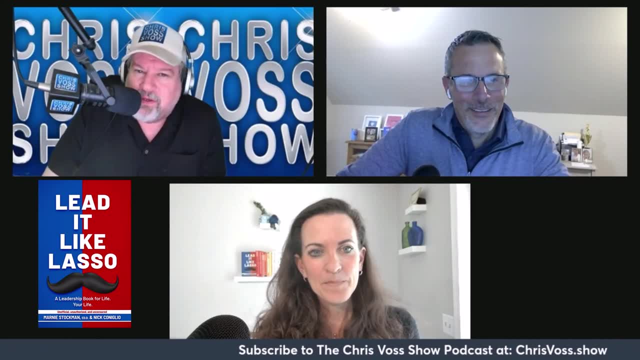 picture, I think, of a wolf, and I still have it in storage. I guess I don't love it that much. It's not on my desk anymore but there's no room, But it basically it says something to the fact that you have to earn your title every day. Just because you get a title doesn't mean that. 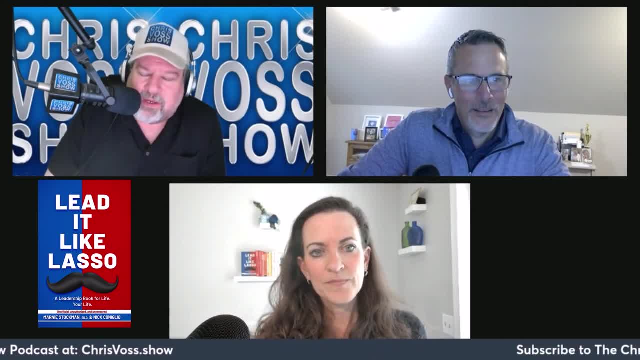 it's yours And I think a lot of people they fall in that trap when they get a title of a manager or CEO or you know whatever it is they're like. I must be that you know that's part of the. 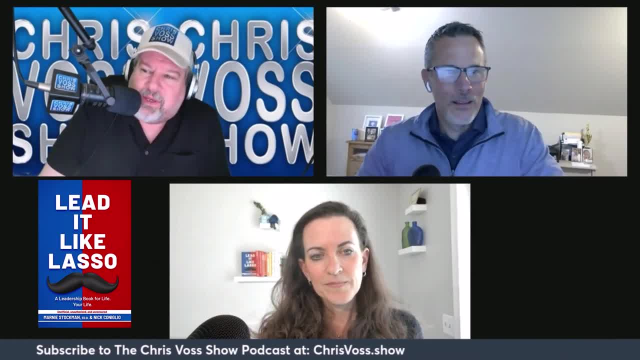 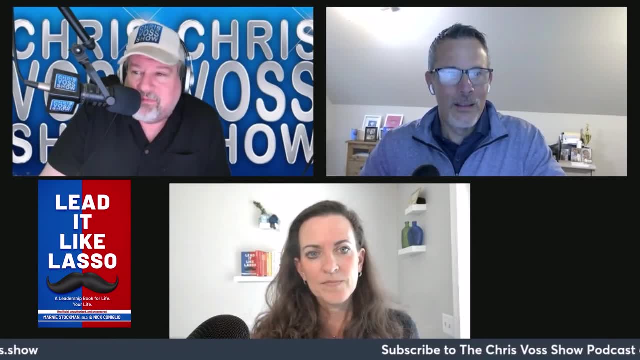 totalitarian egotism And they and they don't realize they have to earn it every day. They have to go out, they have to work their team, They have to earn their position every single day, Even even with me being an entrepreneur, where I, you know, I could just be an egotist and no one could. 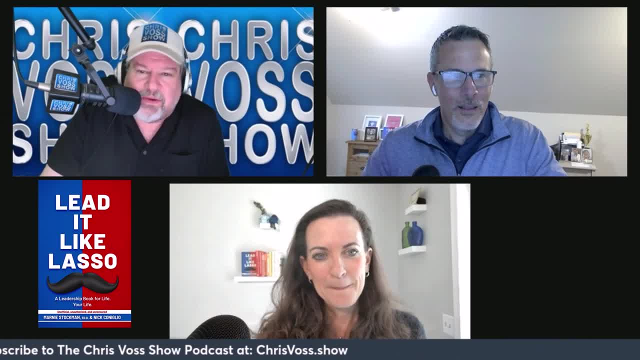 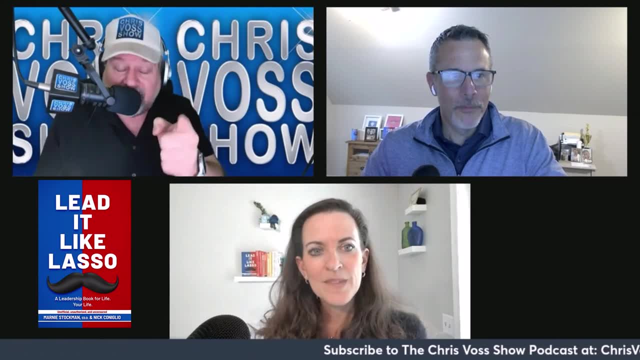 fire me, Ted Lasso. You had to. you still had to have that if you wanted to get the most highest performance out of your team. But not just that: you don't have to have the title to be a leader. Ah, I love it. 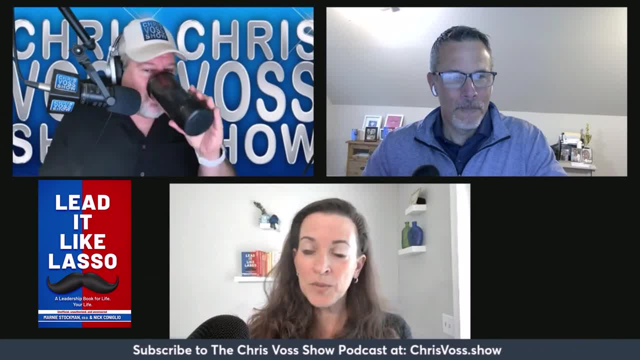 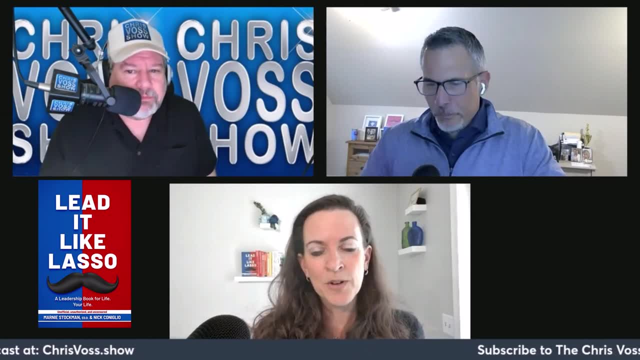 So in the company, when Nick and I worked together, it was the first acquisition that we went through together and it was. it was tough, right, It was emotionally. it was not easy for folks And, Nick, you want to tell them what we did with Performance. Pete the mascot. 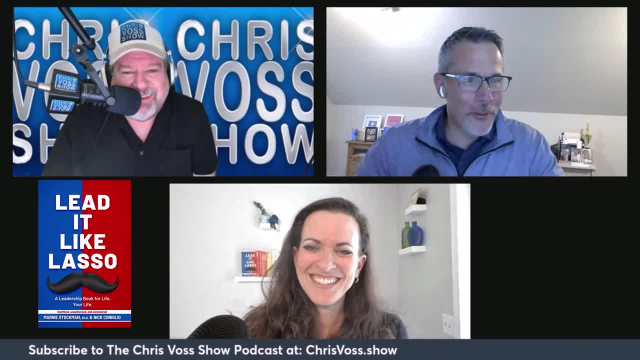 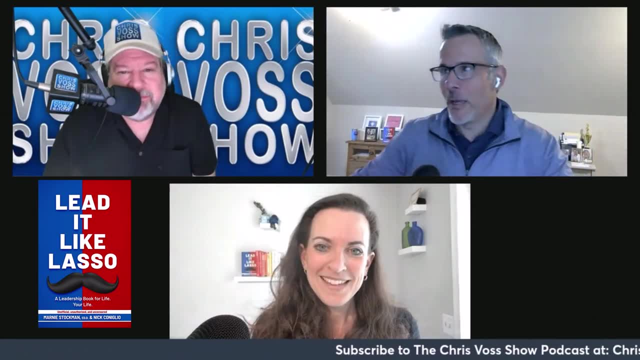 There's a mascot. Yeah, the mascot It was. I wasn't going to go there, but you know it was. it was a six foot steel sculpture, or a sculpture right That that we ended up- Kidnapping. 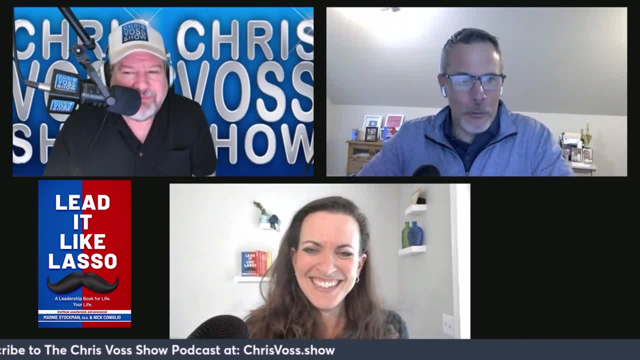 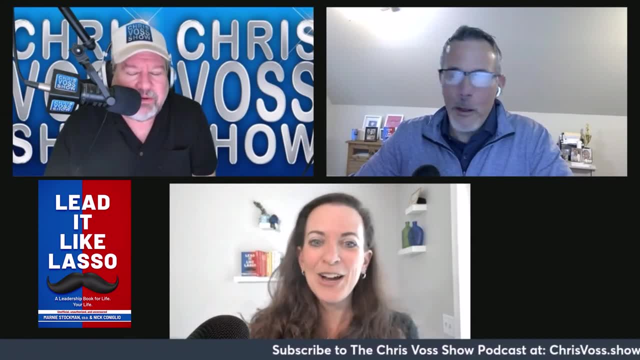 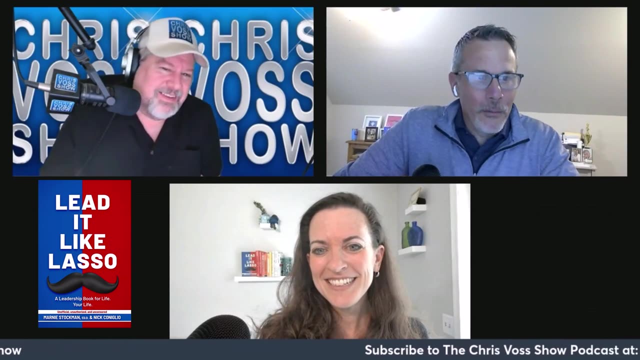 Yeah, we were. we were going through the hard, we were going through a difficult time. We were about to be acquired The six foot performance sculpture. Was this from Viagra or what? No, it was a testing platform for students. But, yeah, we, we kidnapped it and we we posted pictures all throughout Orlando. 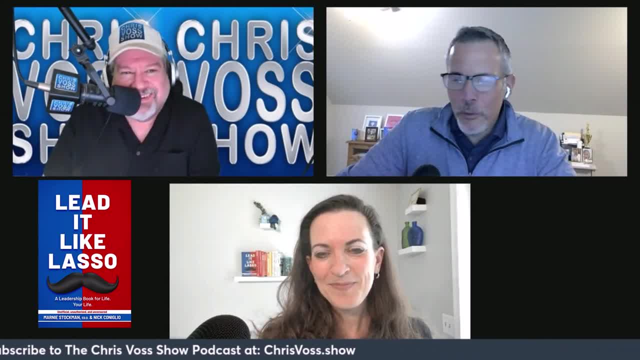 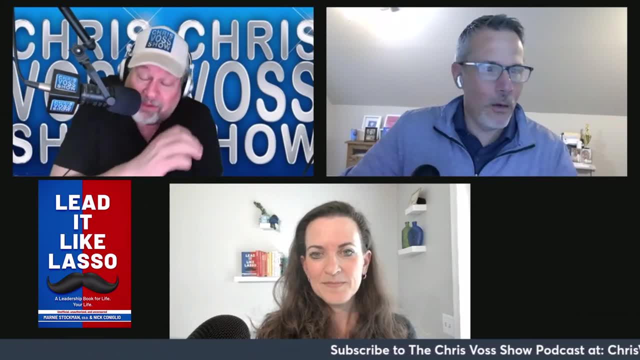 Where is performance, Pete? But you know really what we were trying to do, right is we were trying to make everybody in the company realize that you know what, okay, we've just been acquired for the third time, or the second time, or what have you right? 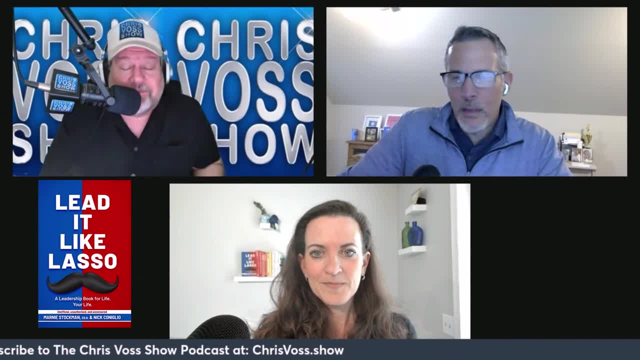 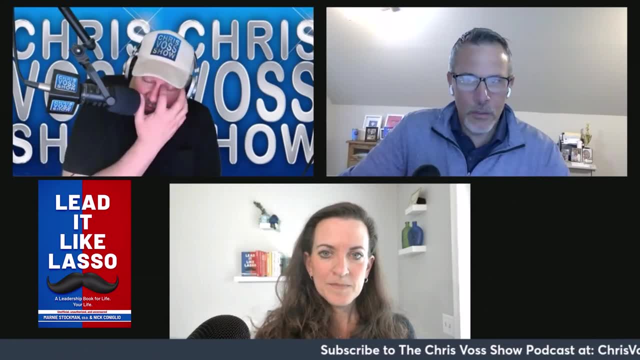 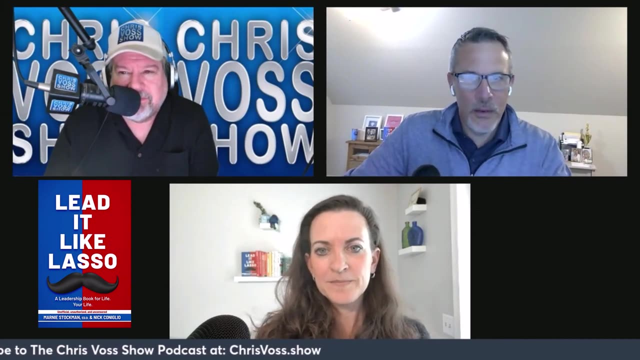 It's okay, We're the same company, right? And I think you know, while Marnie and I were not the CEO or co-founder of that particular business, I think we really stepped up and demonstrated, you know, what it's up to everybody in the organization to make sure that everybody is feeling good about where we're at. 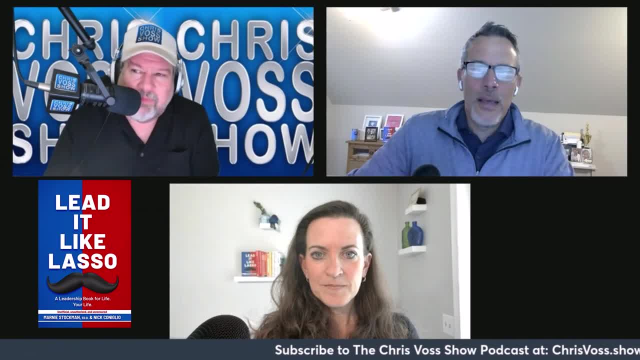 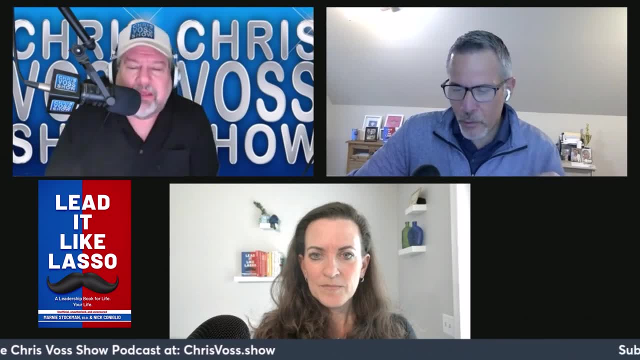 And I think that's to Marnie's point- Everybody's a leader And you know the feedback that we get. you know, I have one story just about our book And you don't normally. You don't normally think of students as leaders, right? 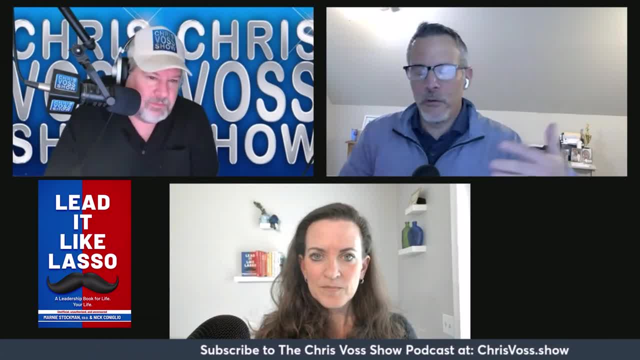 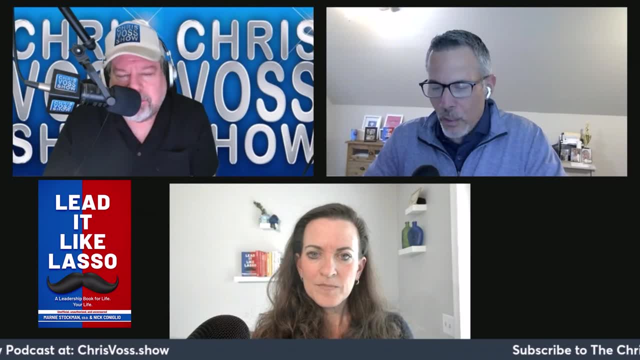 They're typically they're so young and they're- you know, you're graduating college, looking for jobs. And we had one guy that's a friend of my son's who read our book and he kept on having issues with the interview process, trying to get his first job out of college. 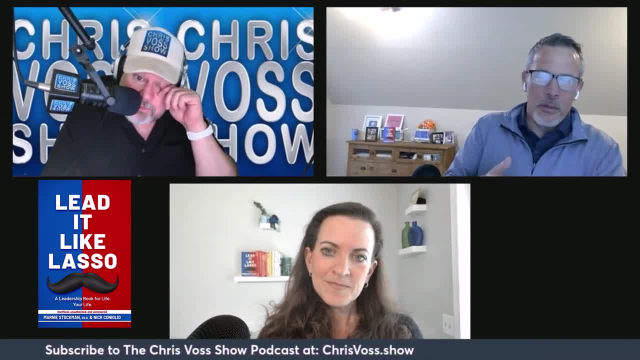 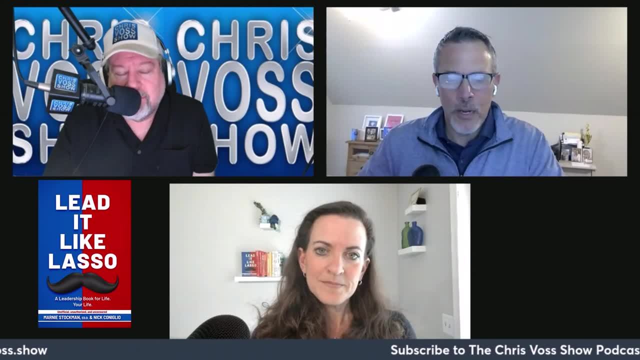 And he kept getting stuck with the question of all right, talk about a time when you've demonstrated leadership, Right, And you're, you know, you're just like, okay, I was treasurer for my fraternity, or you know? so I was captain of my baseball team. 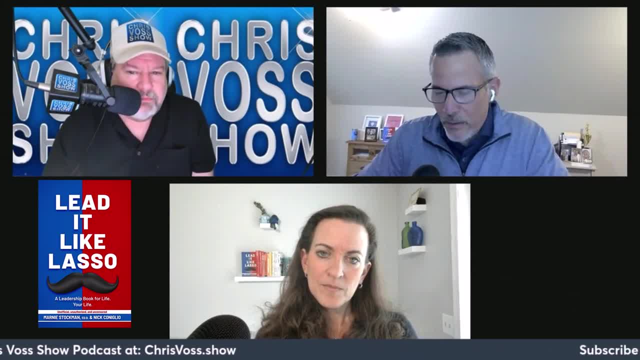 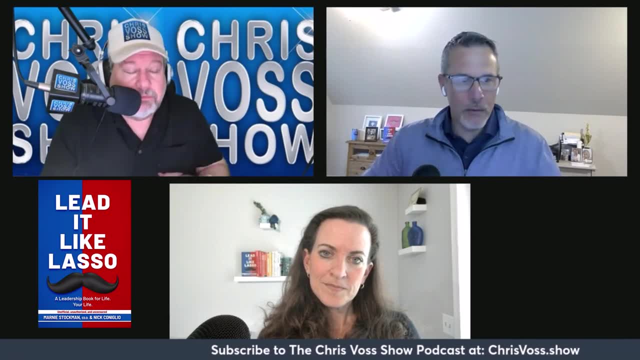 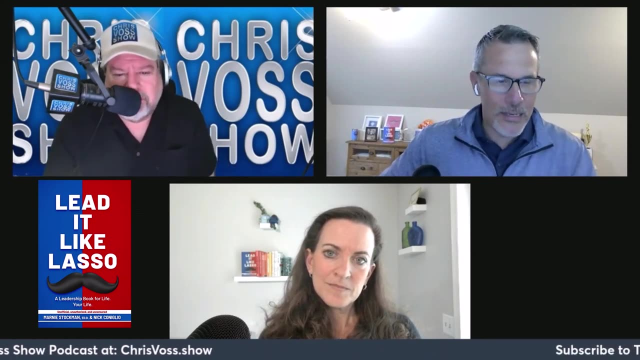 And he just never really was able to nail that answer, But after he read the book he actually, the next time he got asked that question, he talked about modeling out his own personal leadership journey and what he did in terms of setting goals, creating a vision, identifying who he was as a person. 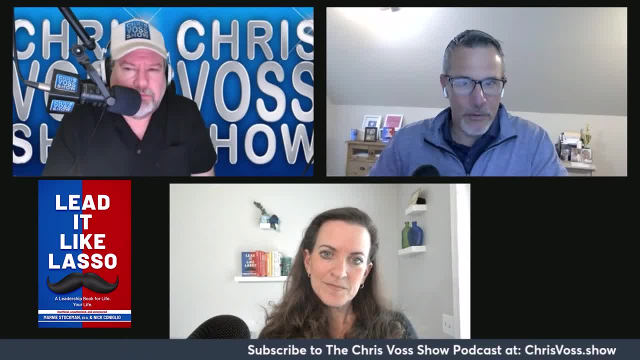 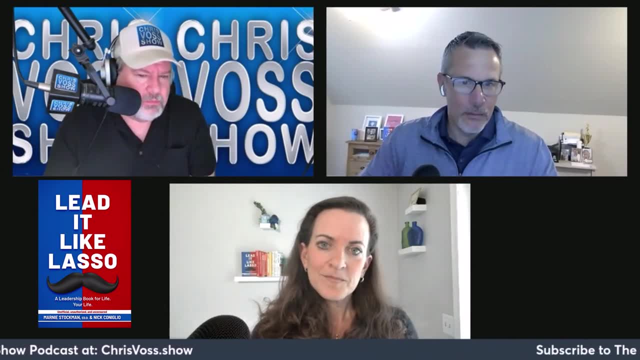 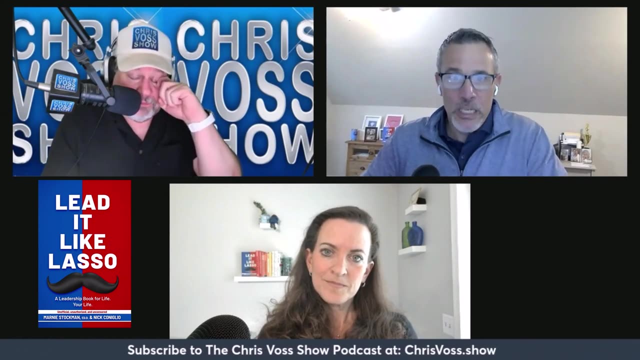 And the feedback that he provided as part of that process Was how well that was received. It just it bangs home the point that you know everybody is a leader. I don't care if you're a parent, if you're a student, if you're, you know, a clerk at a bank. you know you lead your own journey. 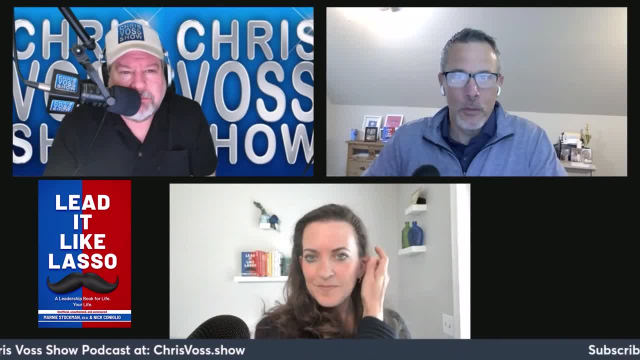 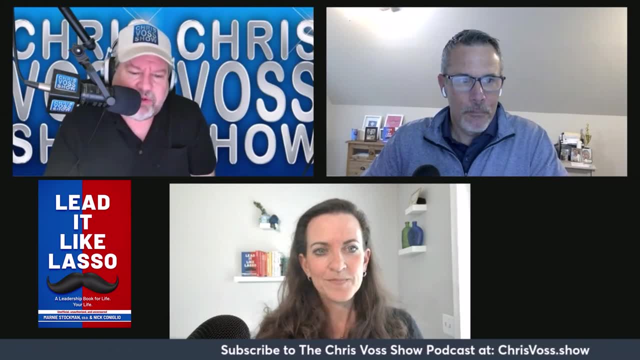 And and and. by that alone, it indicates that that you're a leader. It really does I. you know that. that's the thing that I want to espouse to a lot of people, Cause a lot of people are like you know. they work inside of a company and they're like: I'm not the boss. 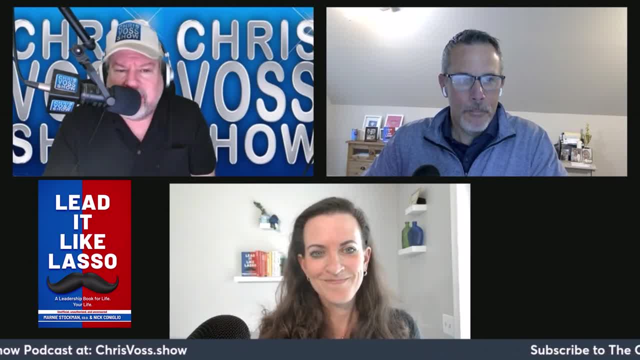 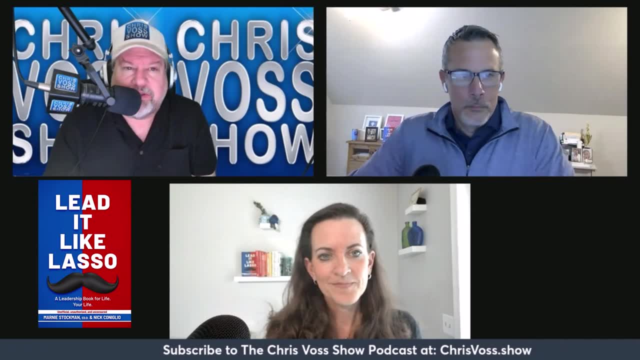 So I just- I can just Just kind of slum it here. No, you have the ability to lead in lots of different places. I mean, I've been running companies, I guess, and being a boss and having that sort of leadership personality so much that I get that everywhere I go. 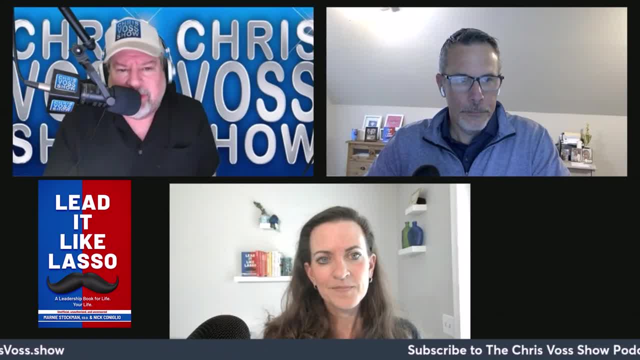 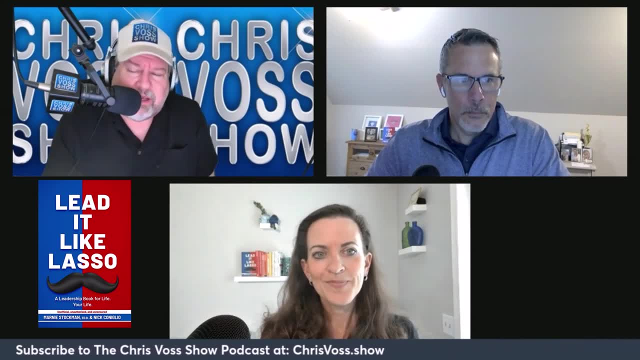 Like people kind of. they kind of stand up a little bit and they kind of notice me a little bit more. Maybe it comes across in my voice and my delivery, but maybe it's that I carry on myself like a totalitarian asshole all the time. 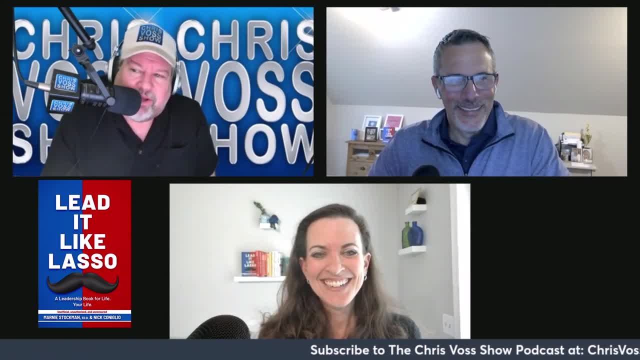 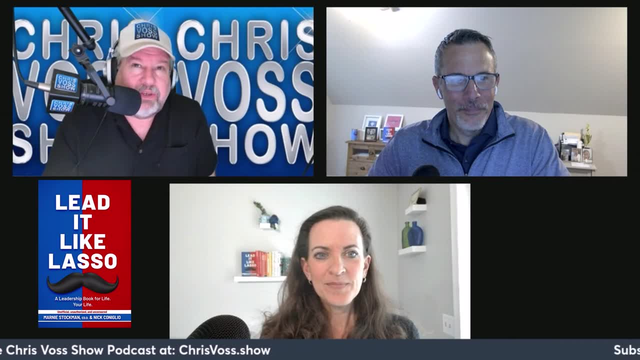 It's just the theme of the show callback. But you know I was. I was on a coffee date Saturday and I was wandering around the place getting getting us refills And so some guy came in to the coffee place and I don't know, I just come across as that guy. 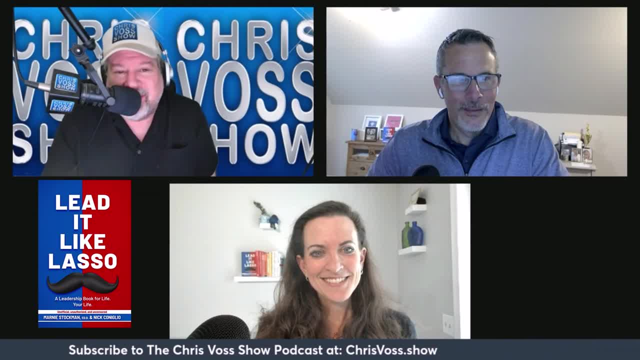 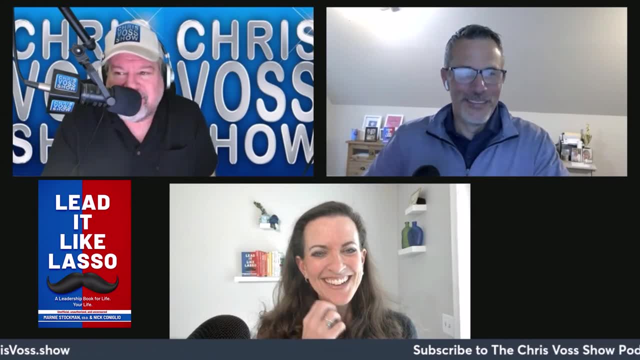 And I- I've had this happen a lot where I remember, And then he, he goes, he goes. do you own this place? And I go, and I actually have a standard answer for it: I go. no, I just look like the kind of guy who owns a lot of things, because I, I do. but you know people get that from you. 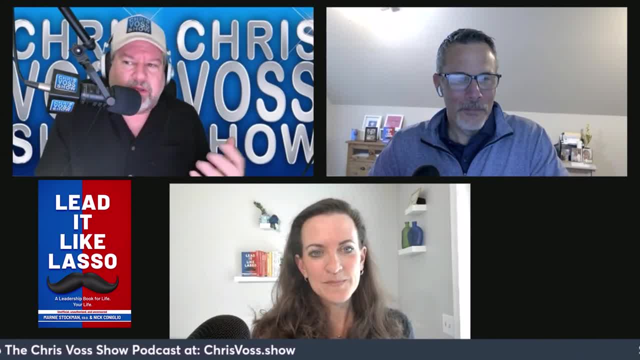 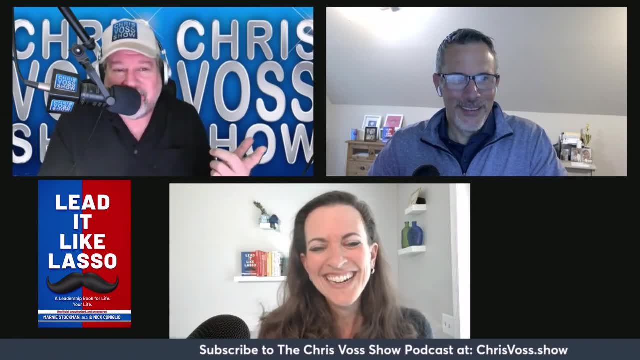 It's. it's really. It's really weird how people can sense if you're a leadership type of person or if you're a totalitarian monster like I am and narcissistic, And in fact, you guys are giving me an idea for a mascot for my company in the future. 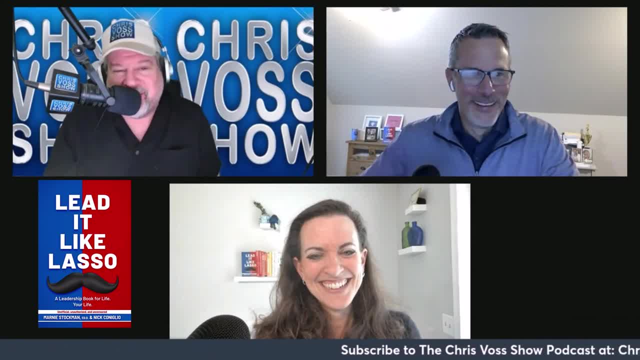 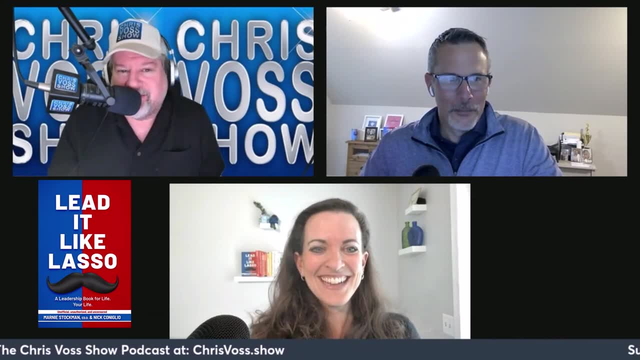 We're going to. we're going to, we're going to put in sticking with a totalitarian, authoritarian regime- sort of leadership style that I have. We're going to call him Mussolini, Max, Nice, They'll love it. Yeah, All my employees are going to have to do that high stepping thing. 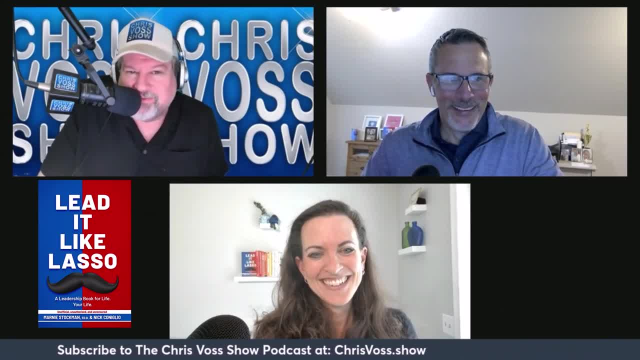 I don't know what that means. Don't do that, folks, please. He wasn't a good person. Don't do that. Maybe we'll just make a mockery of him and that will be the funny thing about it. You know, you guys talk about that in the book everywhere all the time. 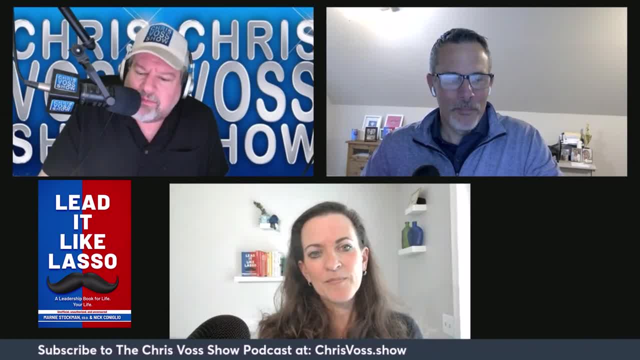 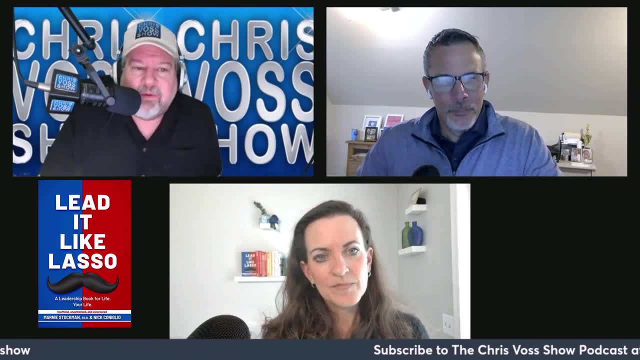 Leadership. you know thinking about it. You know I was watching the. I think it was a CEO of HP. go talk about going through his day and what it was like to march through his day with him And it was amazing how much time he spent not behind a desk- not, not, not. 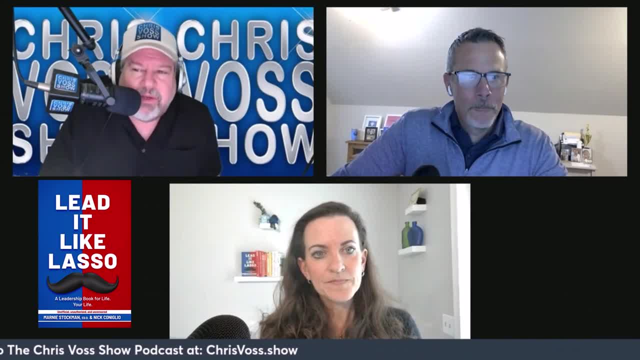 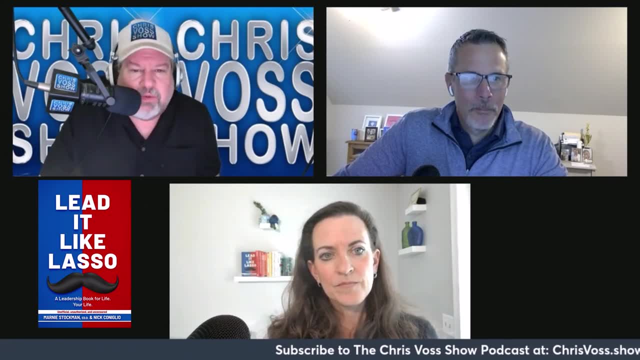 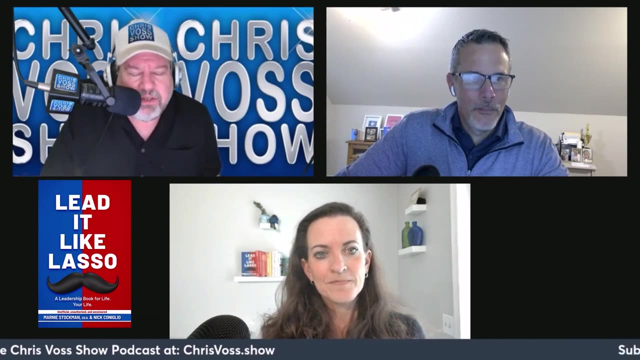 I don't know standing behind a podium barking at people like a Mussolini. but he was actually going around and it was meeting with his team, meeting with frontline employees, And sometimes it was just a little bit of wandering through the frontline, like he'd go down to the lobby and just kind of meet his, you know, whatever employees are there, talk to them, answer questions and just kind of just kind of be there for them. 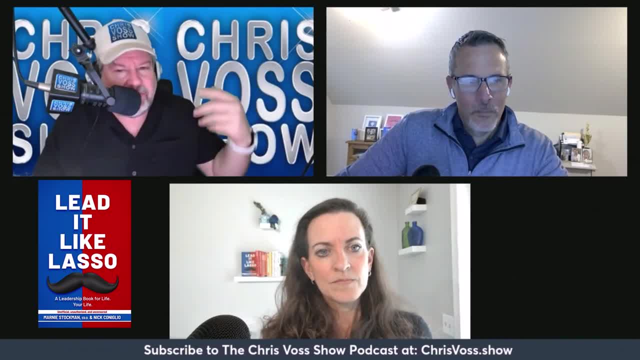 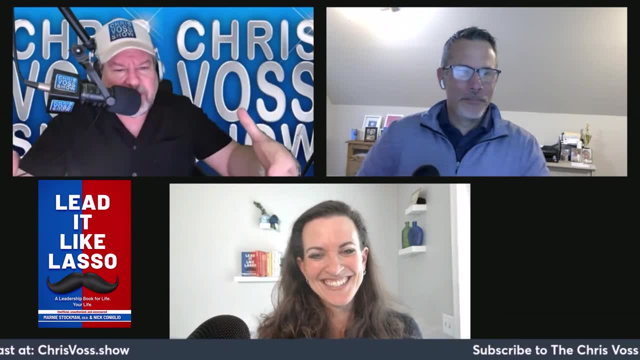 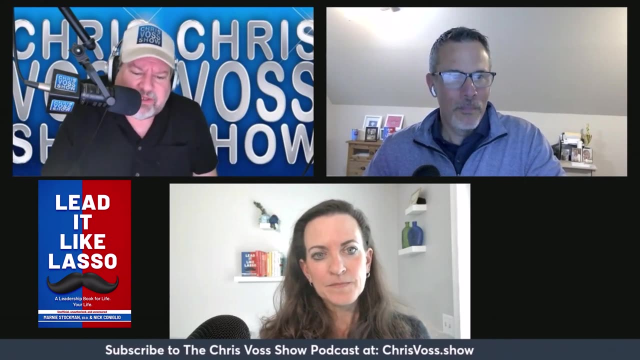 And he would use that to get a lot of. you know we all get stuck sometimes when you're in the ivory tower, you know, if you live in the white house, et cetera, You get stuck behind this. you know you. it's hard to get information on what's happening on the ground and you know you, you create this bubble. you know people talk about it with presidents and, as a CEO, sometimes you you get that. you know you get a bunch of yes men around you. 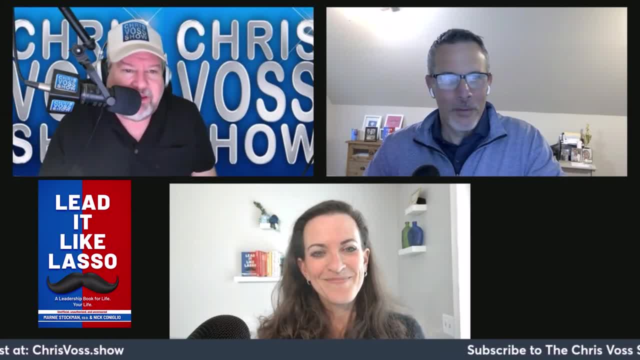 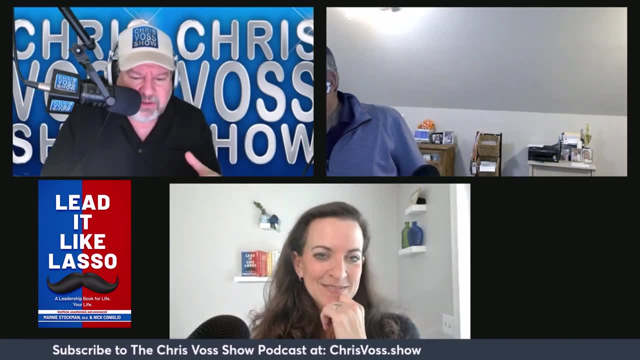 Yeah, you're the greatest with the best ideas, Chris, And you're like, yeah, I am, There's the Mussolini, you know seeing him wander through his corporation and and just you know meeting people, meeting vendors, talking to them. 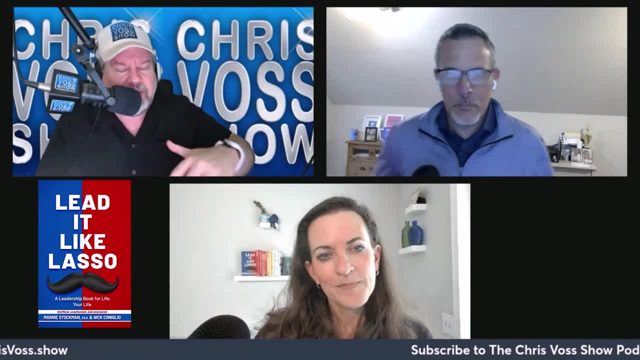 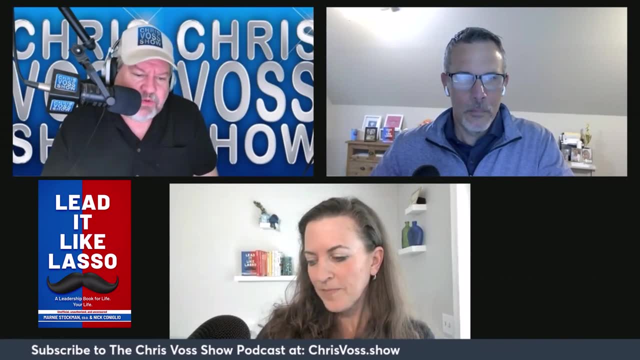 And like every day, this is like his thing was just going around And surveying and talking and asking questions and being human being, empathetic- A lot of things you guys talk about in the book. it just really made me really. it made me really rethink leadership. 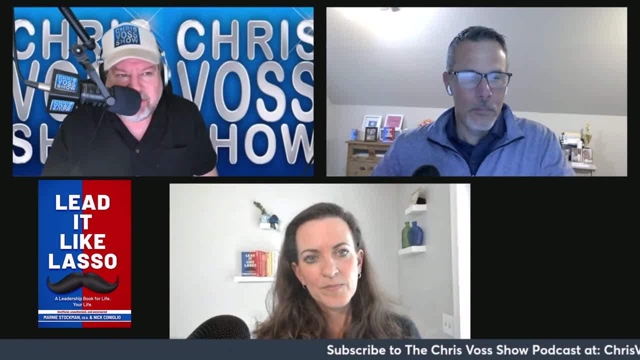 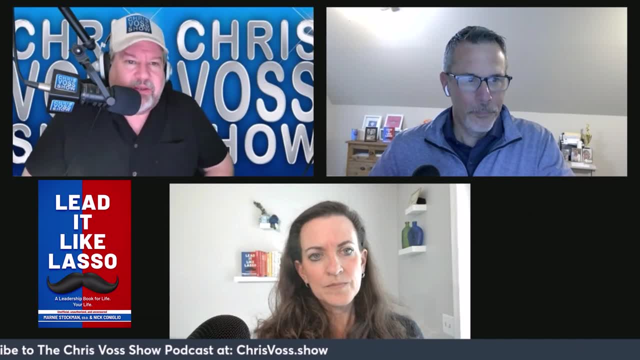 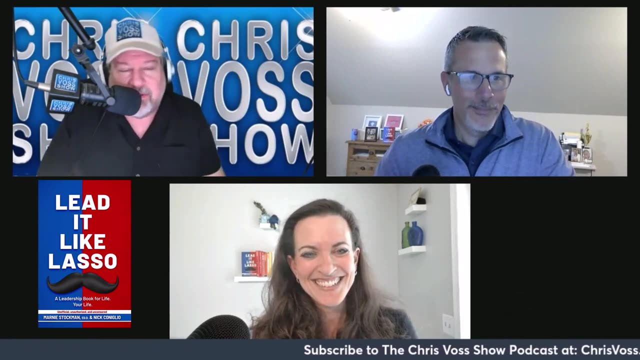 Cause I always thought of leadership is, you know, the Mussolini style? I know I can go back to that, but seriously I I always thought of getting on getting my little box everywhere I go, my little soap box and giving the big speeches and the you know, always shoving vision up people's ass and, you know, trying to. you know, Hey, you know, and always the big oh a. 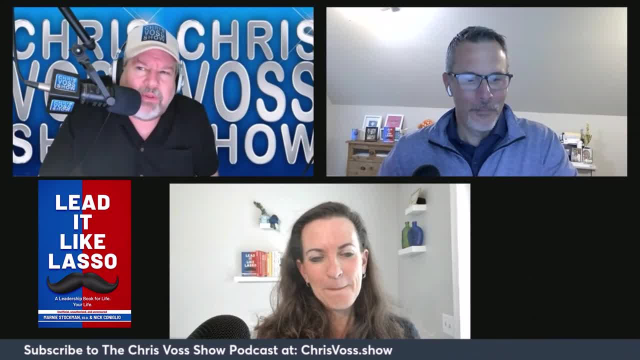 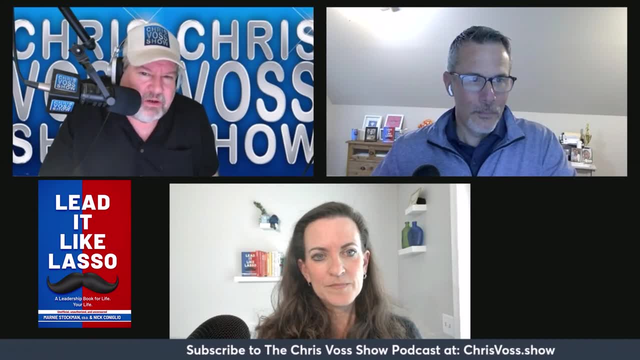 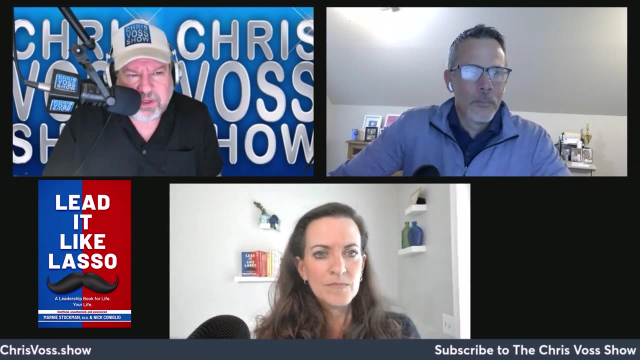 rock And I had. I had one of the. he was. he was the head of the ship during COVID who? it was one of the first attacks on the on on one of our ships during COVID. It was a Navy captain who oversaw the. I think it was the Theodore Roosevelt, if you remember that. 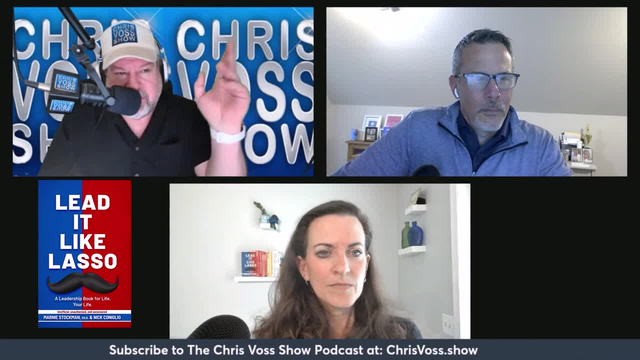 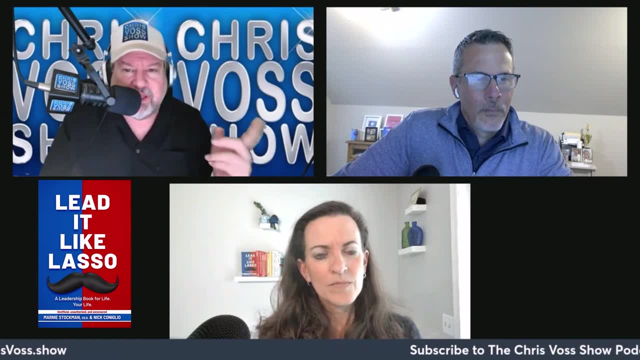 And he, he, the chain of command wasn't going up to the chain of command Wasn't going up to the Pentagon fast enough as COVID was ravaging the ship, And so he Wrote a letter directly to COVID. end up the president gone involved at that time an orange haired guy. 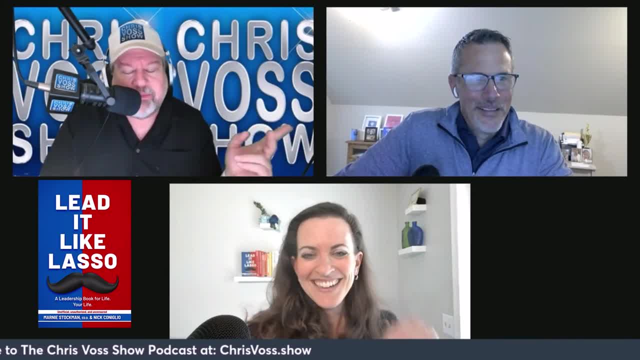 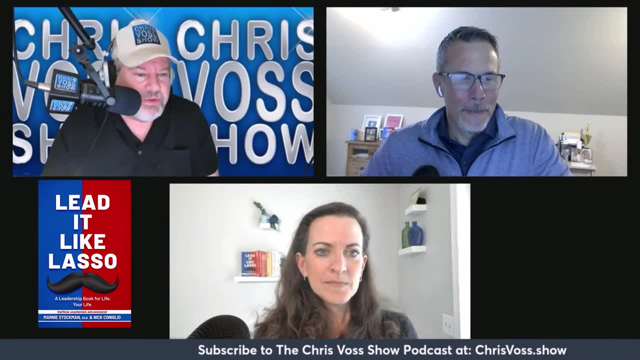 You may have heard of him and I think he's bankrupt or something, but anyway he got viscerated because he was making COVID seem as bad as it was that they were trying to hide. He was a. it was a captain, Navy captain Brent Crozier, and his books are full. 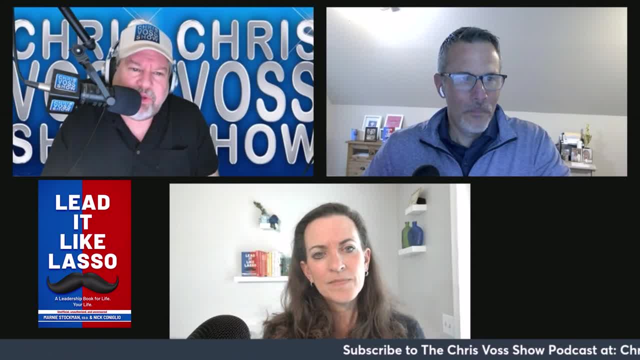 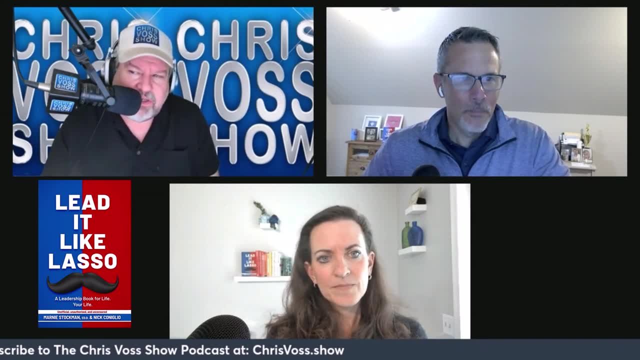 You can't. he was on the show and what was interesting to me was how. how he wasn't the raw, raw sort of leader. He was the he, his, his leadership was very stoic and very quiet and very mild. 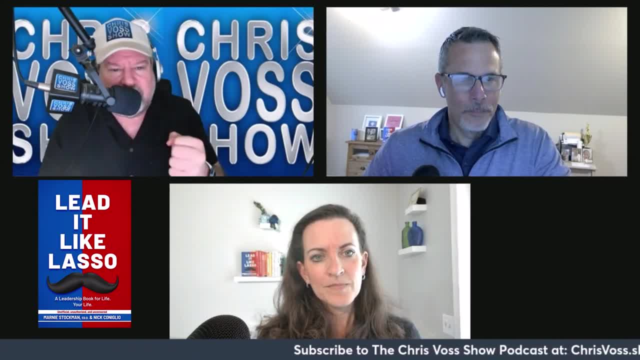 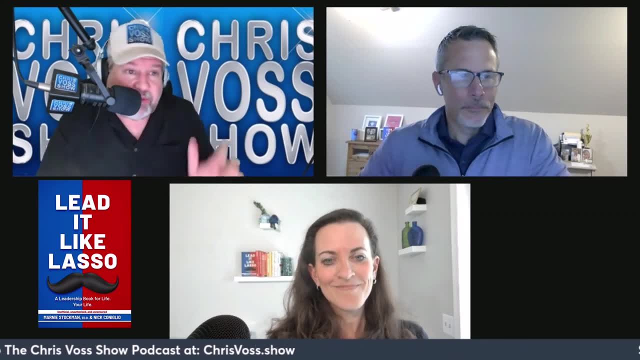 And he really made me rethink the raw, raw sort of leaderships things. And if you remember, the story was when he was removed as captain of the ship because he'd spoke out and broke protocol. He was trying to save his sailors. The whole ship cheered him as he left. 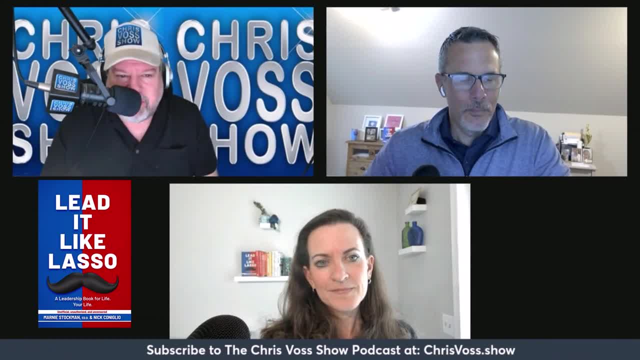 And even when I asked him, I go. what does it like to be eviscerated by the president of the United States on Twitter and be run through the thing We've had? a few People on the show have gone through that experience. 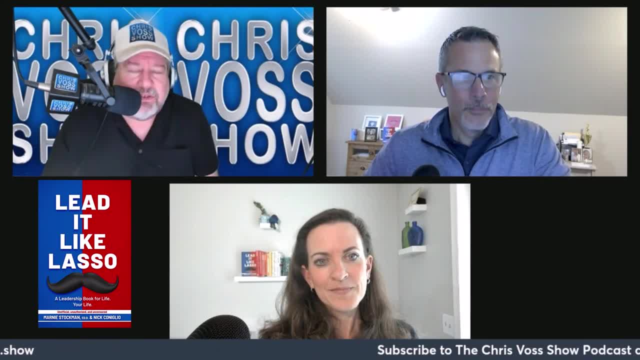 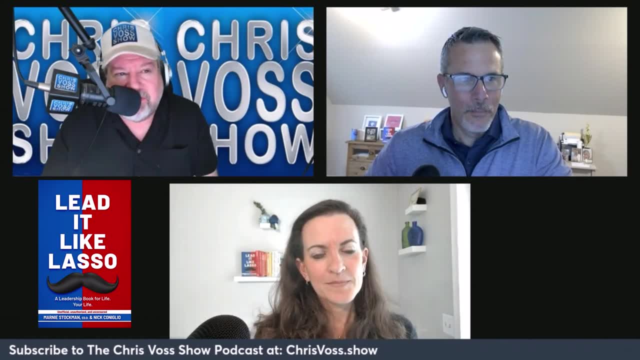 And I'm like, what is that like? And it's your commander in chief as well. So it's just not the president of the most powerful and just the most nonchalant, careless, just there was no emotion at all. He's like man. everyone's entitled to their opinion. 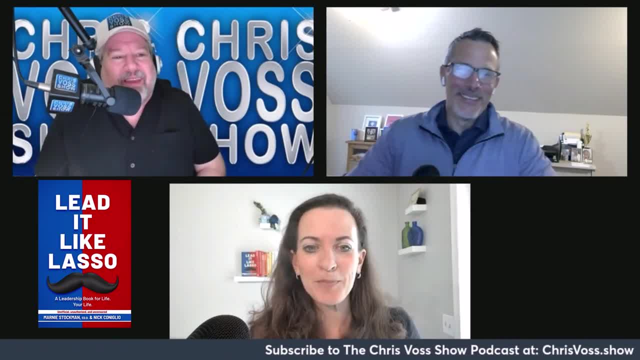 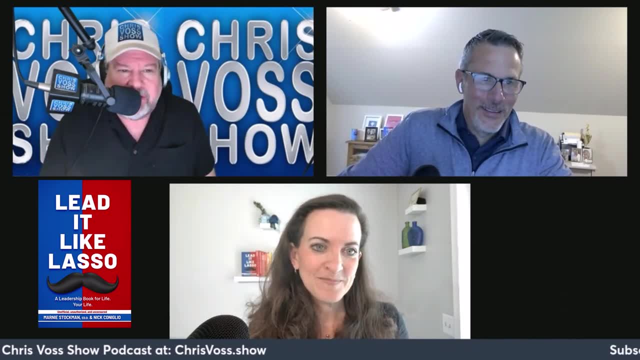 Yeah, I was like the whole world would be a better place if everyone could take feedback like that, And so it really. it really made me think less about how you don't need to be that leader. Who's the raw raw? 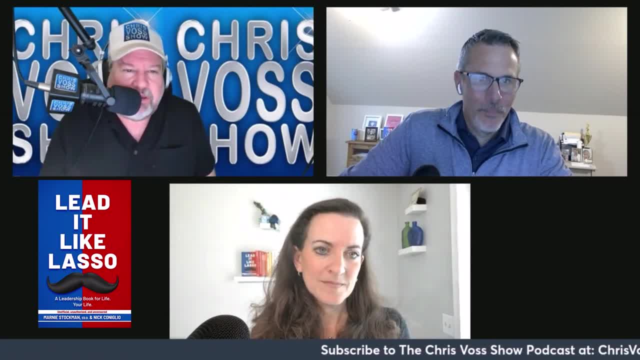 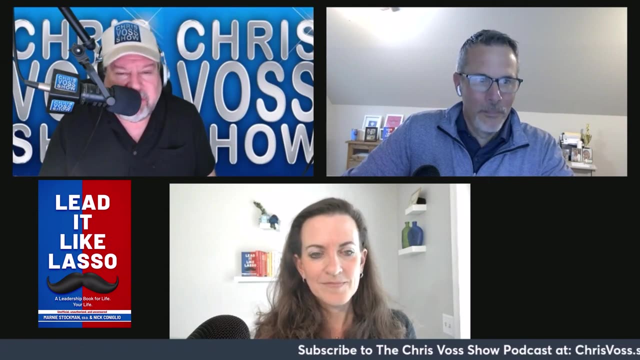 Who's the raw, raw cheerleader. you know barking orders, barking vision. you know blasting people in their face all the time trying to get control, sending out PR things. you know some of the things you espouse in the book and the the lasso thing of. you know listening, empathy, all these different facets that that kind of turn you out as a better leader. 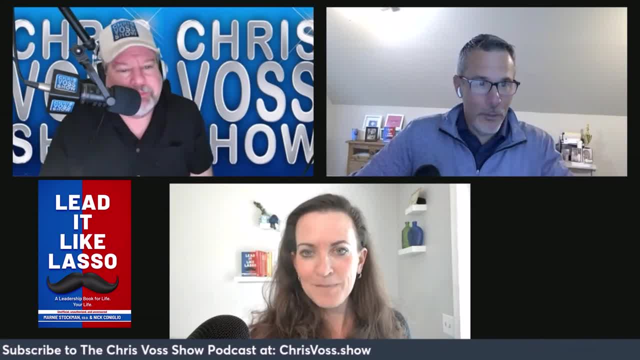 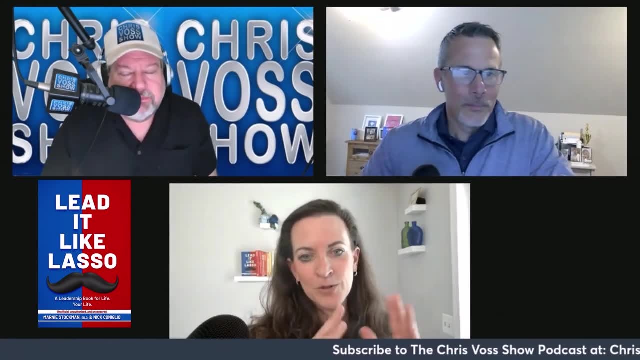 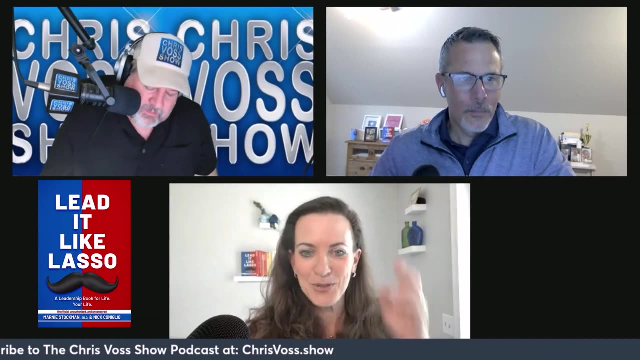 Yeah, no doubt. And I mean I was going to say Jim Collins book good to great. The difference between a level four and a level five leader is humility, Humility and force of will. Right, So I think the humility shows the the, not the rah rah, Nick, I doubt that's what you were going to say. 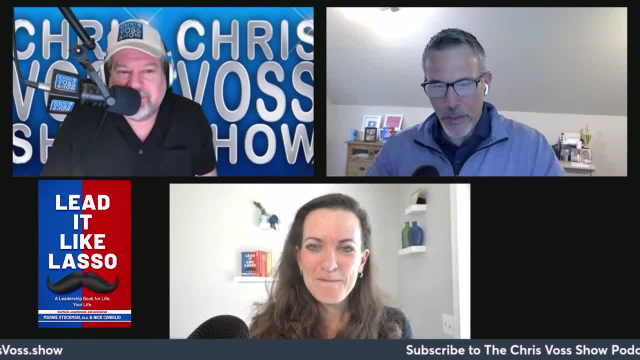 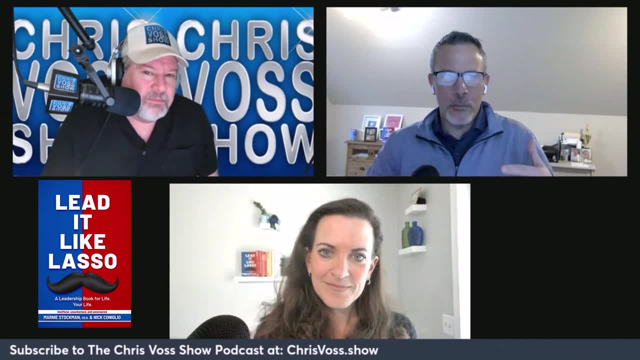 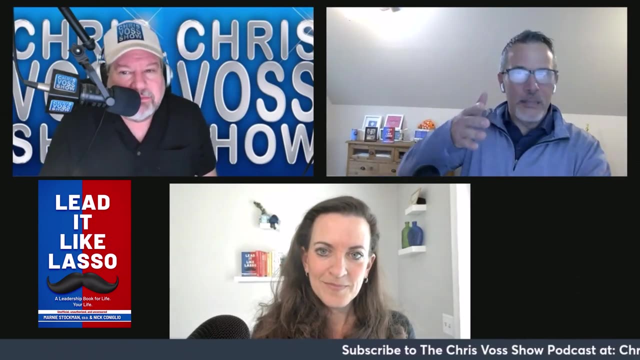 No, I was. I was just going to add right, And we were talking earlier about you have to earn. earn your respect, you know, earn your title of leader every day, And you know what you talked about, Chris, is the difference between the traditional, old style command and control leadership. you know who speak, you know, compared to the, the more modern leadership. 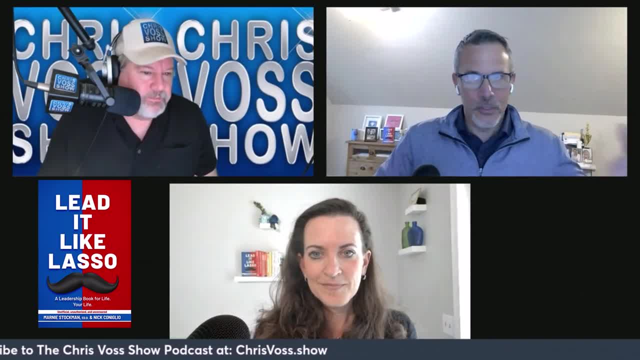 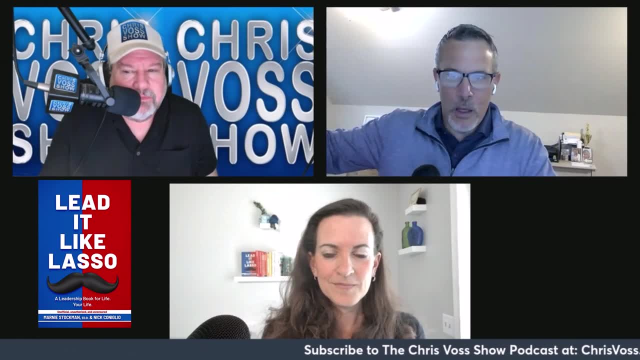 Who listens right? It's. it's the old style of Hey, all I'm concerned about is outcomes versus the new style, which is all right, I am. I I'm very concerned about the growth and development of my team and to us, it's. it's the difference. 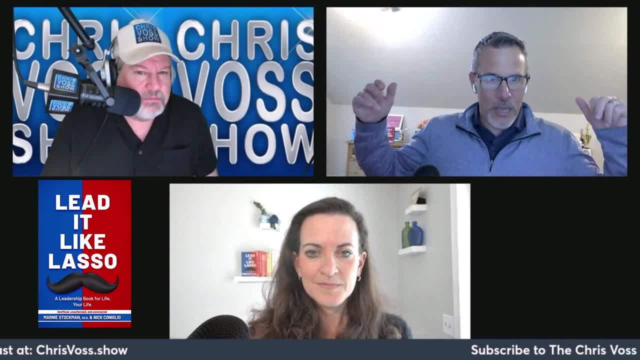 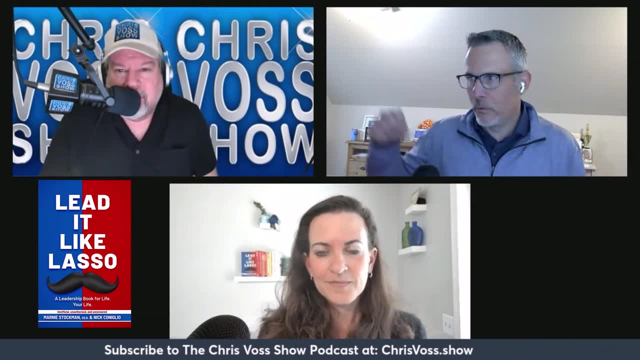 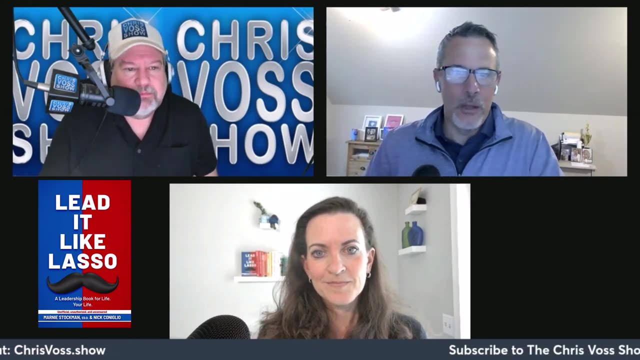 Although you're technically a leader because you have the title. what we're talking about is the difference between a manager, right, Somebody who's very task oriented and barks out orders, versus a leader, somebody who inspires, And I think your, your story and anecdote is is very much aligned with the exact messages that we try to get across in our book. 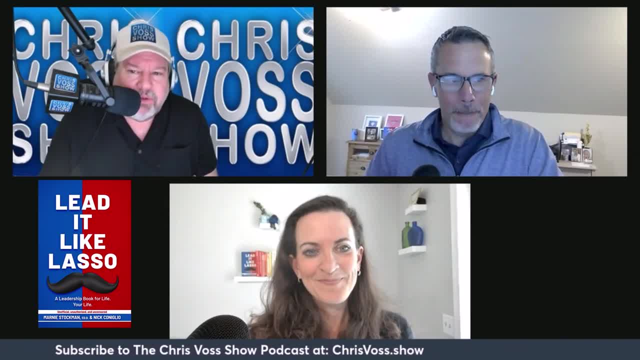 There you go: Servant leadership- They call it a lot nowadays, Yep, And you know between the things that we're talking about- compassion, empathy, loyalty, fun, teamwork, achievement, honesty, growth and a partridge in a pear tree. 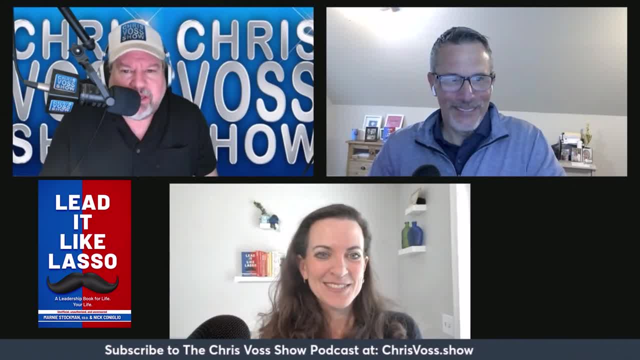 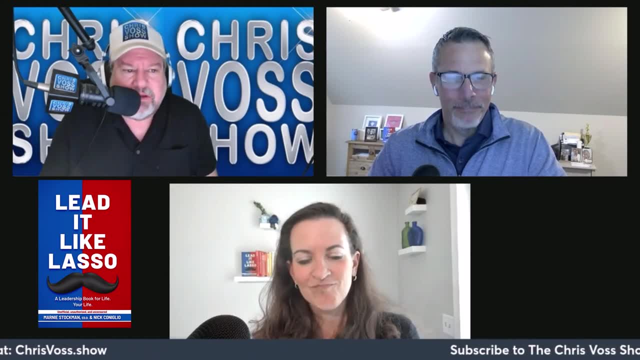 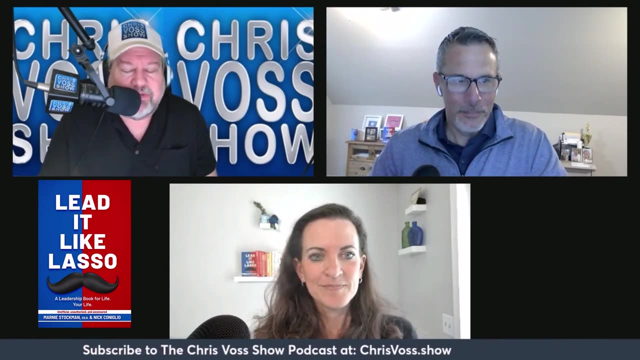 These are all things that you know. we've kind of learned over the decades in age that they bring out the best in human, in the human condition, in the human ability And in they bring out the best in human beings and so many people you know. I wish I'd pull the stack because we quote it so often on the show, but most people leave a job because they're sick of the poor leadership. 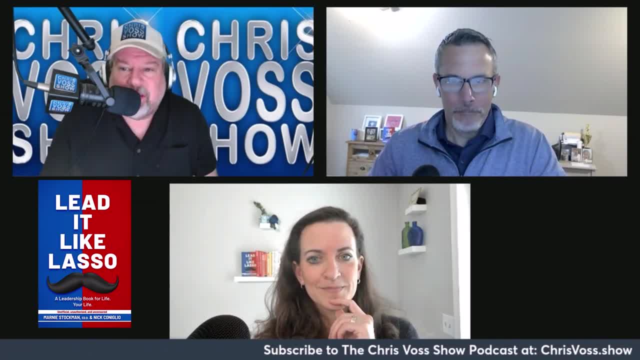 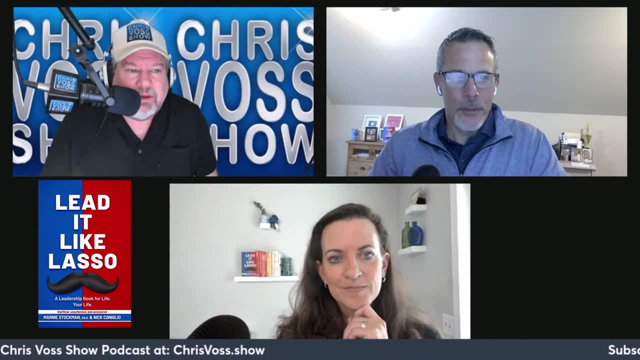 Oh, absolutely, And it really comes down to that. I mean, and there's so many companies I've seen that have failed and really the person who's responsible for it as a CEO at the top and and you're like you've- you've really ruined, like everything. 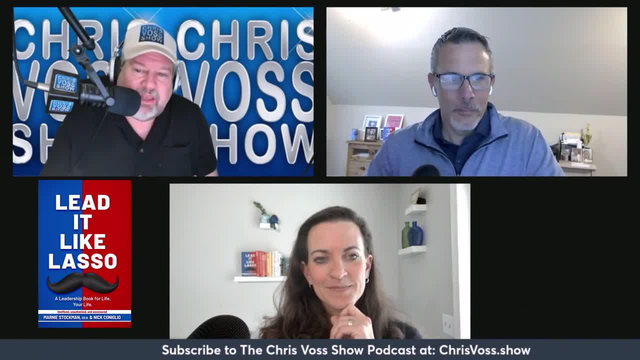 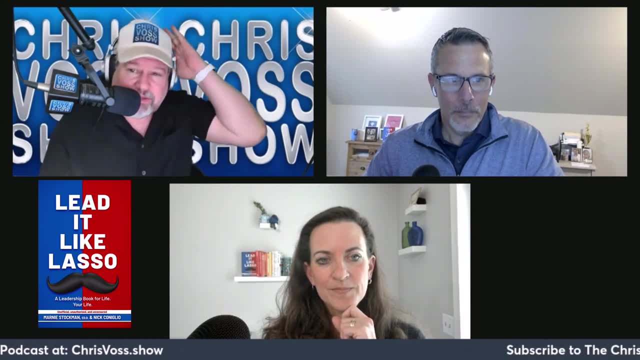 And and it It's you, but sadly, a lot of times they lay off so many people and they put you know their employees through the the thing first, And usually after they lay off and fire enough people, they, you know the board starts going. maybe it's the CEO. 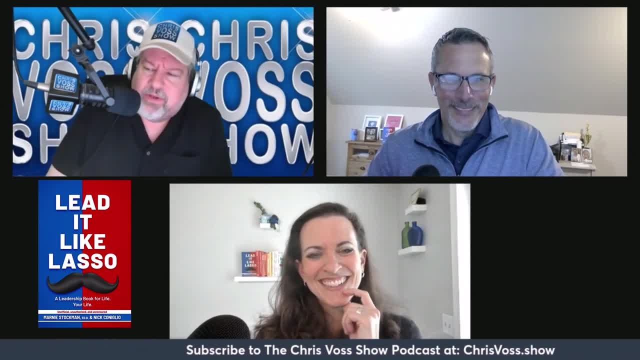 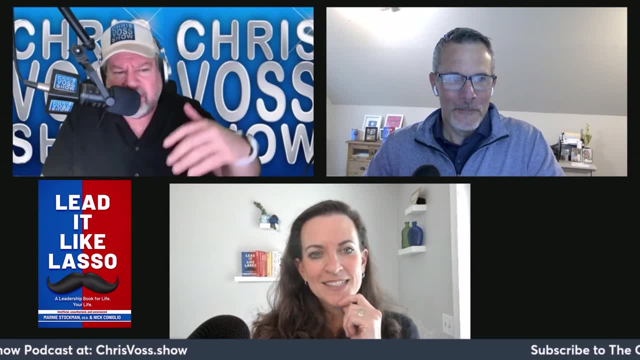 Maybe it's them. You should have started there first. So final thoughts as we go out on the book: any tease outs maybe we didn't talk about, or any topics we want to cover? Are you guys doing coaching or advising or consulting? 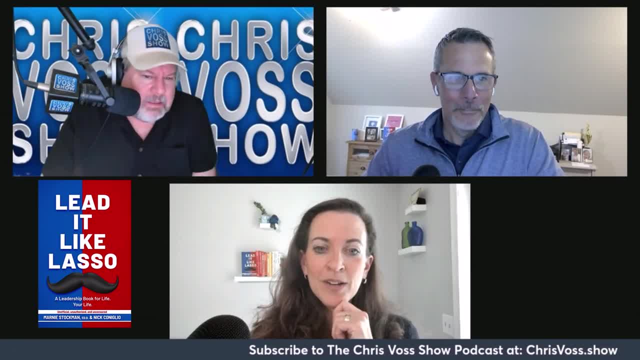 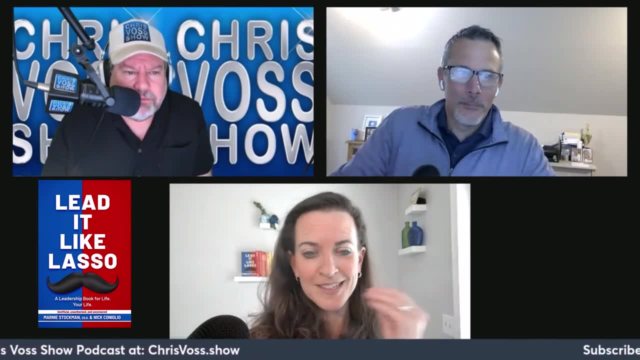 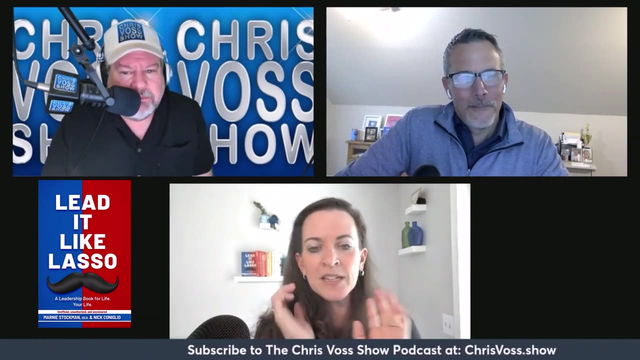 I noticed there's some different things on the website on resources, So we are currently building a masterclass. So folks that are interested in learning more about their own personal leadership, they should follow us at lead it, like lassocom. I did want to say one thing you had mentioned when you're the leader, that is, the Nick said command and control type of leader. 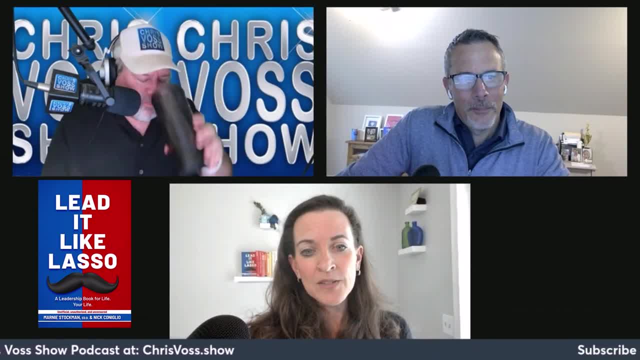 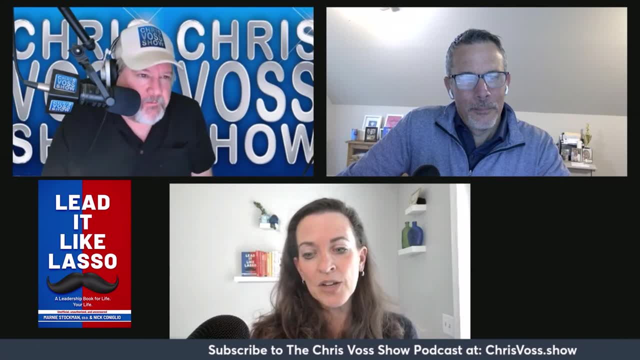 Folks don't often believe that they can challenge you, And so the entire growth of the company is limited by your own. you know limitations, And so in Ted lasso there's a group called the diamond dogs, and it's the other folks that he trusts in. 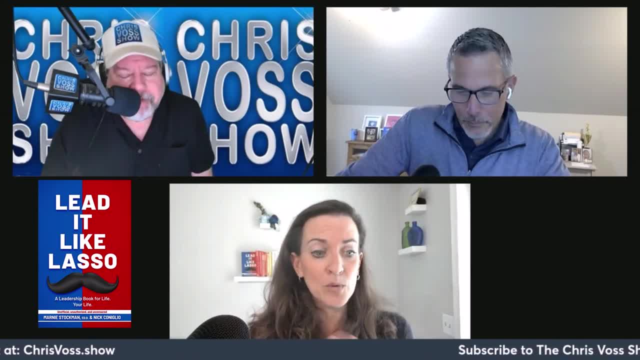 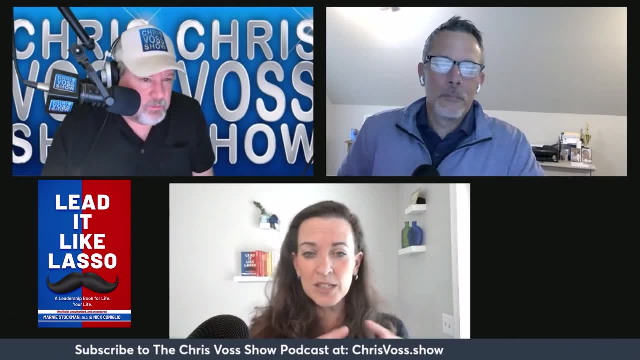 And to have someone that you trust and are vulnerable enough, or a team that you trust are vulnerable enough to give you honest feedback to help push you to the best version of you, I think is really critical for any human, not just someone with the leadership title. 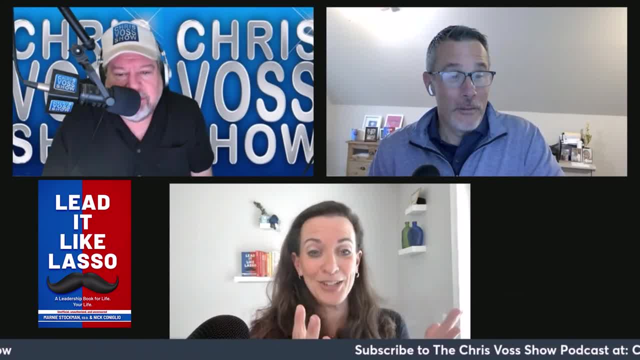 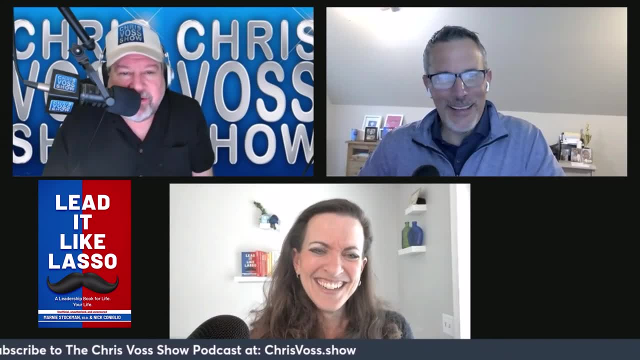 Maybe you should have a diamond dogs mascot. There you go. That way they can kidnap and pull around Atlanta. This is why I get to pay the extra $5- more than most people- for these ideas Brilliant. They're only worth $5. 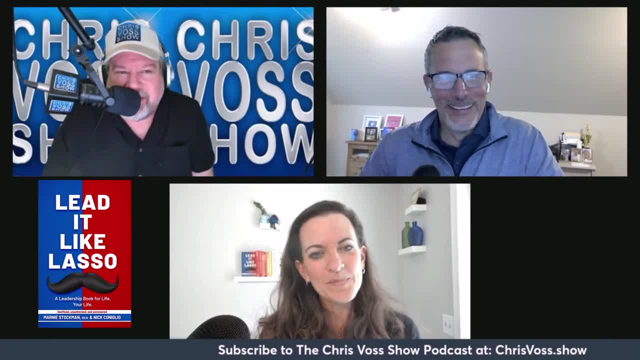 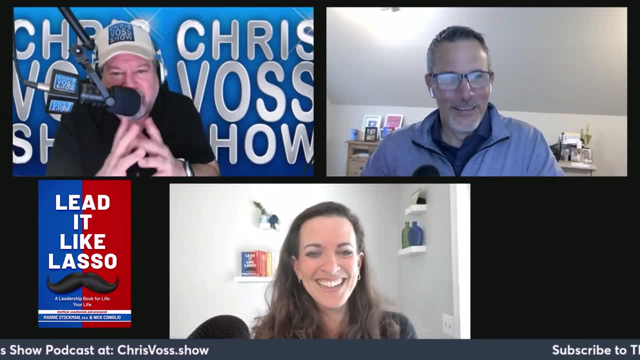 The diamond dogs mascot. Yeah, I should have a mascot, because the mascot, you know, could walk around and I don't know he can entertain people and keep them motivated And I'll just sit in my office and scheme things, where I'll just have a cat evil. plans of Mussolini max coming. 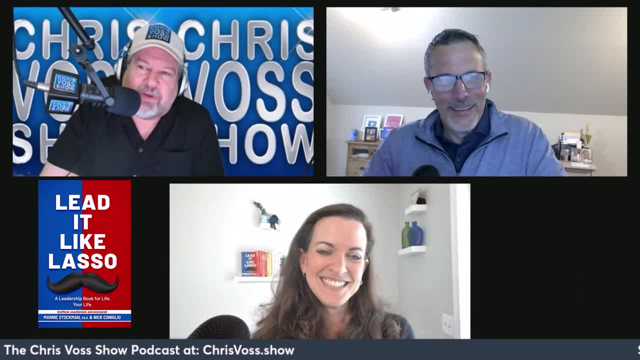 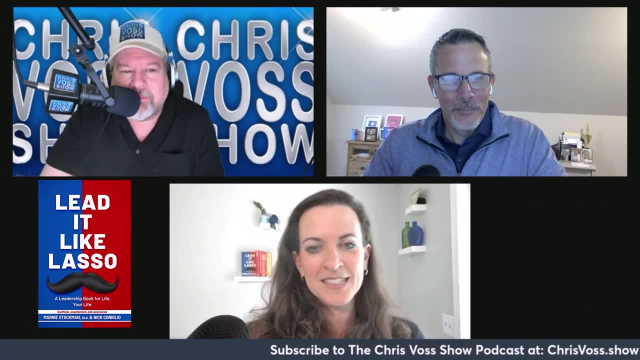 I don't know what that means, but uh, uh, thank you guys for coming on the show. Give us yourcom. So where can people find you on the interwebs? Yep, Lead it like lassocom And then all the socials at lead it. 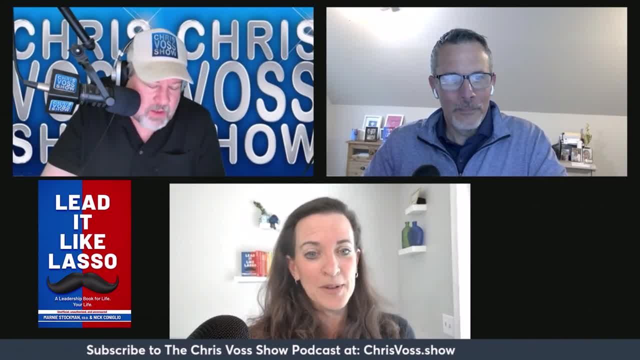 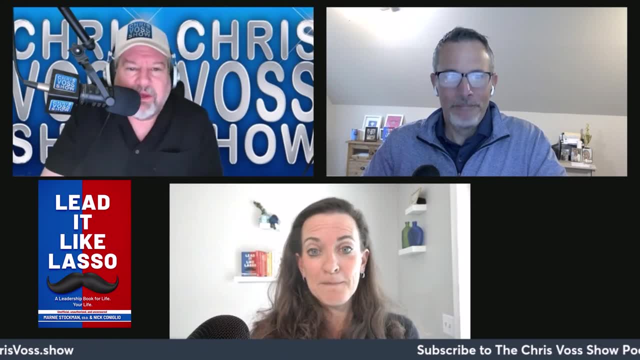 Like lasso, And of course, we're both on LinkedIn with relatively recognizable names. There you go And I got both of your raises in there. Everybody's in, Yes, Everybody's in. You know you could do that. You could take the mustache that's on the cover of the book and you just wear it. 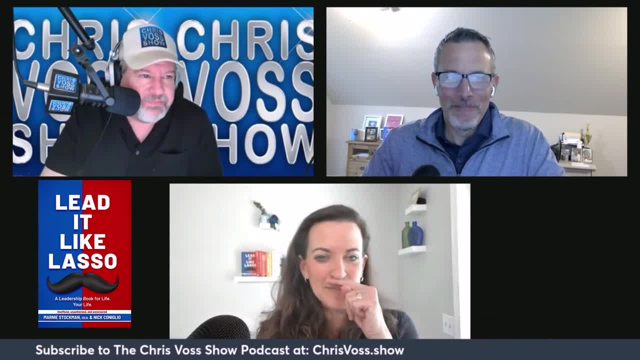 Everywhere is, I don't know, a branding symbol or something I I we do have. I must ask you a question: ideas. Yeah, there you go. If you guys come back on the show, we're going to make you wear the mustache. 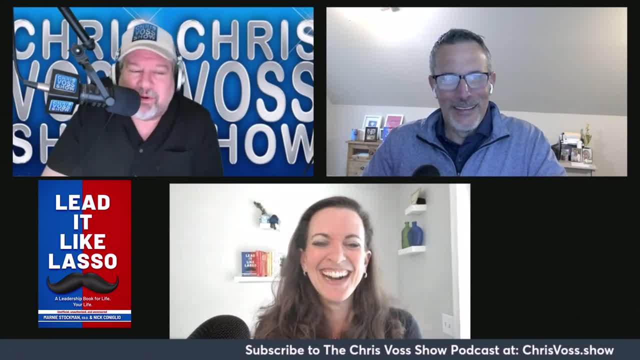 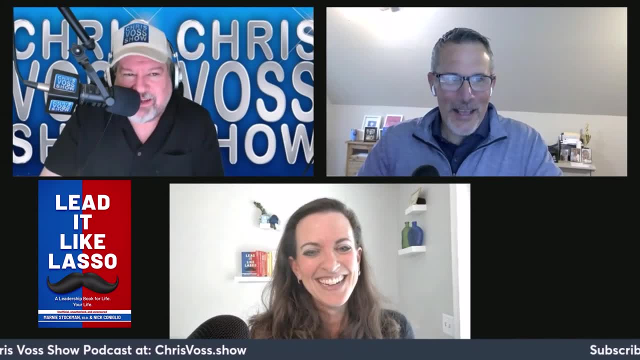 Okay, Deal, Both of you. I'll wear one too. Wait, I already have one. I'll work on it. See, there's pills you can take that can fix that, I'll just. I'll just grab my cardboard, one that's in the kitchen. 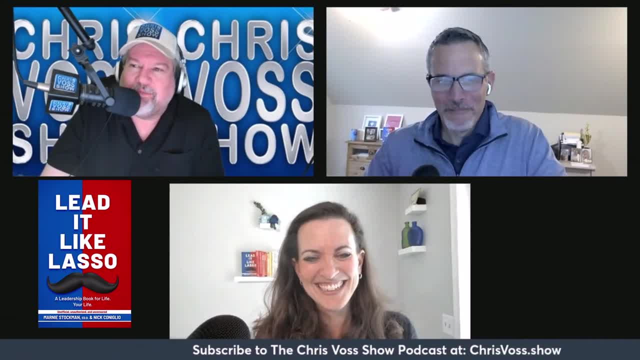 Get some testosterone, start shooting that up, You'll be. you'll have hair in no time. So there you go. Thank you both for coming to the show. We really appreciate it. It's been a lot of fun. Thanks for having me. 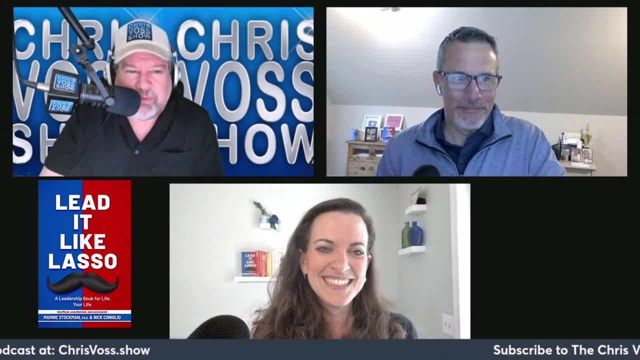 We appreciate you, Chris. Thanks, There you go, folks, And order wherever fine books are sold. Stay away from those alleyway bookstores because you might need a tetanus shot or you might get mugged. So there you go, Stay. go to the good ones. 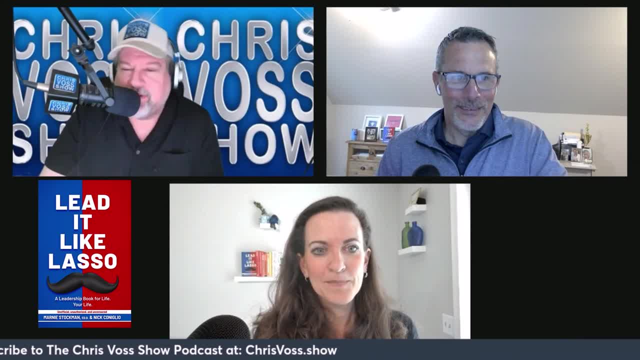 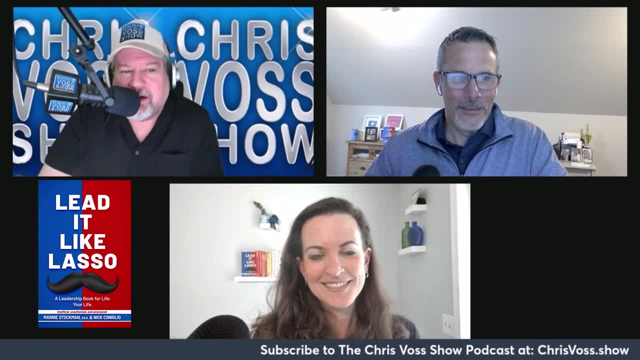 You can find on Amazon at lead it to. I'm sorry, let's recut that The book is entitled. So lead it like lasso: a leadership book for life, your life out October 7th, 27th, 2023.. 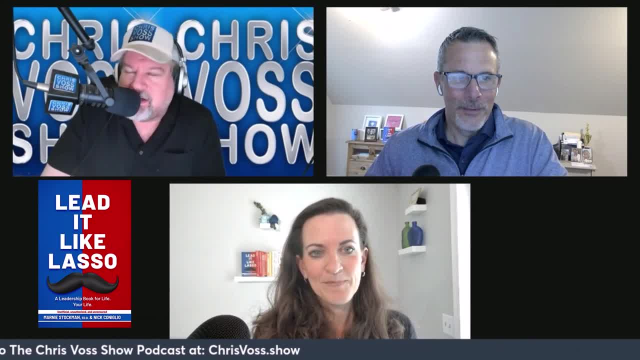 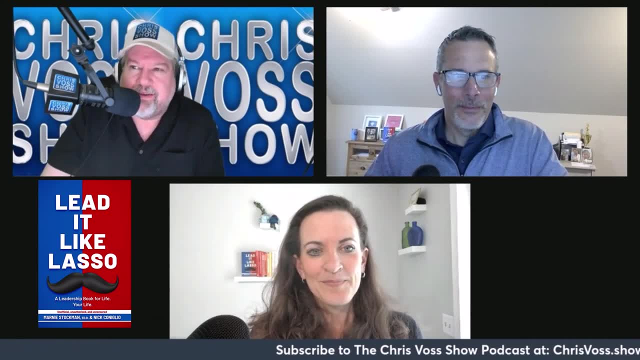 Thanks for tuning in. Go to good reasoncom for just Chris Foss. linkedincom for just Chris Foss- all this crazy place in the show or on the internet, and refer the show to your family, friends and relatives, or else I don't know what that means. 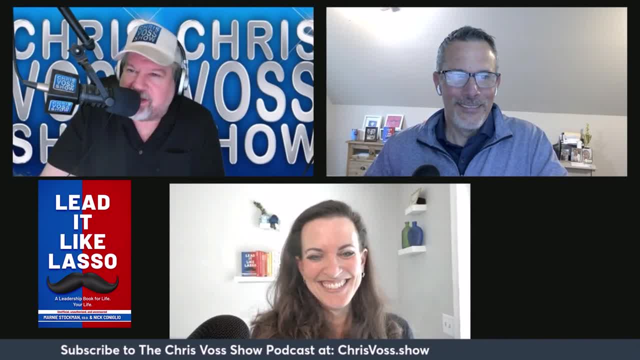 I'm just kidding. Take care, Be good to each other, Stay safe. We'll see you guys next time.